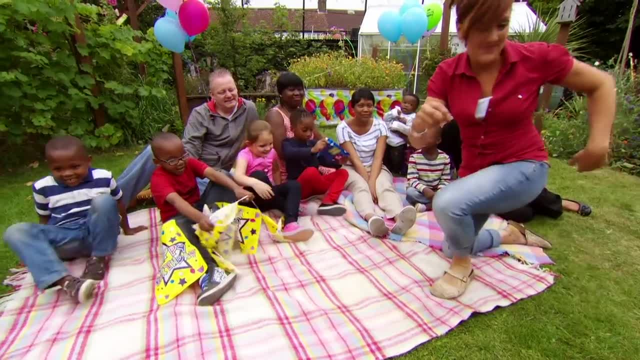 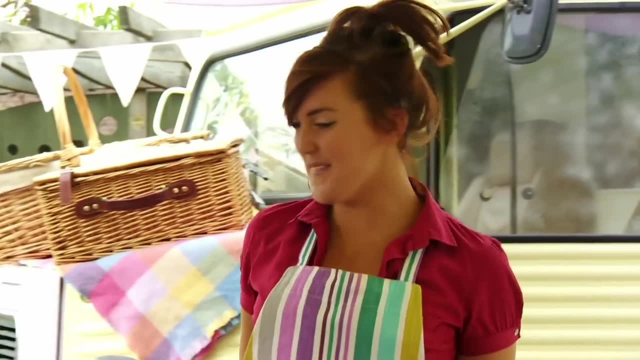 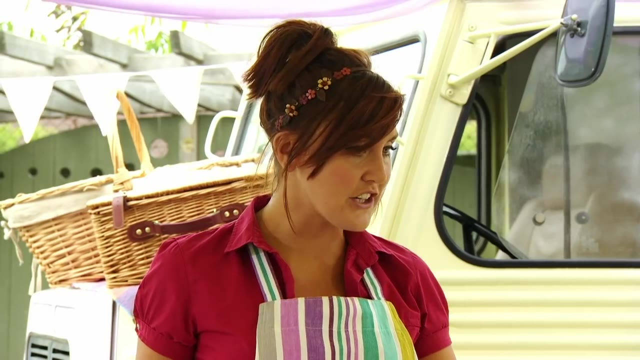 Let's do some cooking everyone. Yeah, Come on then, follow me. Welcome to my outdoor kitchen, everybody Who's excited about doing some cooking Me. Do you want to know what recipe we're going to cook? Yeah, Okay, I'll show you. Today's recipe is celebration. 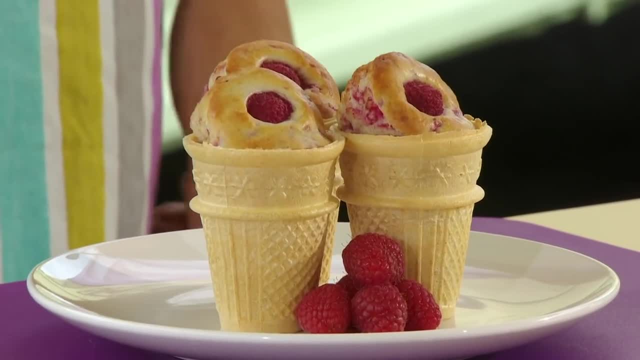 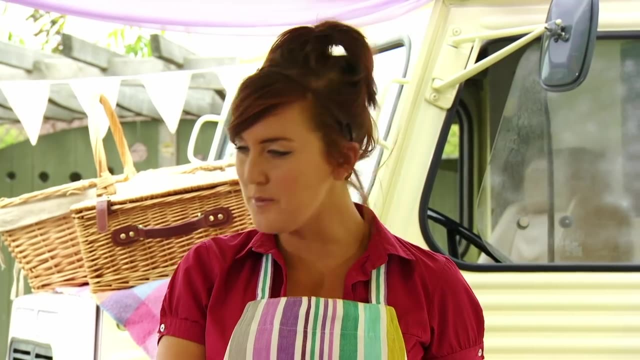 cornet cakes. Look at this, Mmm. Nice, hey, But before we get cooking, we've got to do some cooking. Yeah, We've got to do some cooking. We've got to do something really important. Does anyone know what it is? 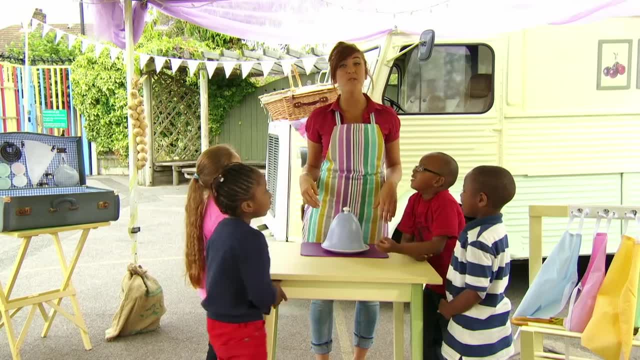 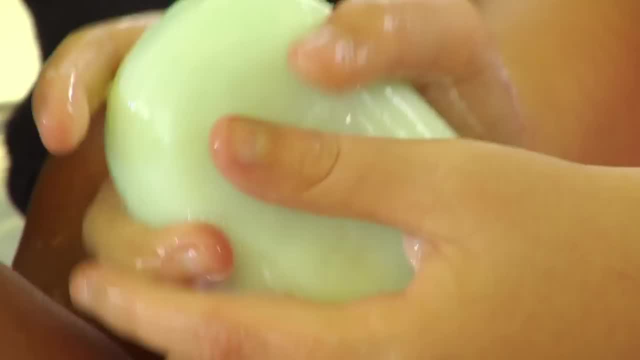 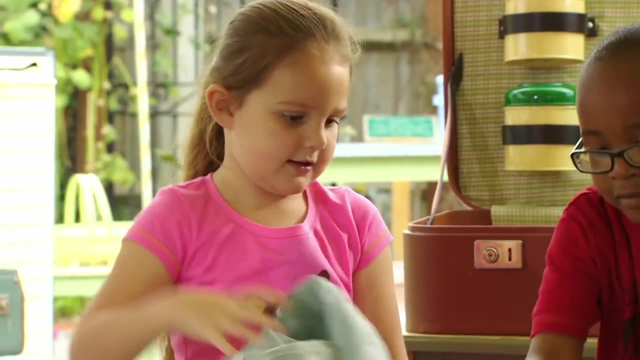 Wash your hands. That's right. we need to wash our hands, of course. Come on, everyone, let's get going. Roll up your sleeves, give your hands a wash With slippy dippy soap, swish, splash blosh. Have you done your hands Washed and dried? Sleeves rolled up, apron tied. What can you do? 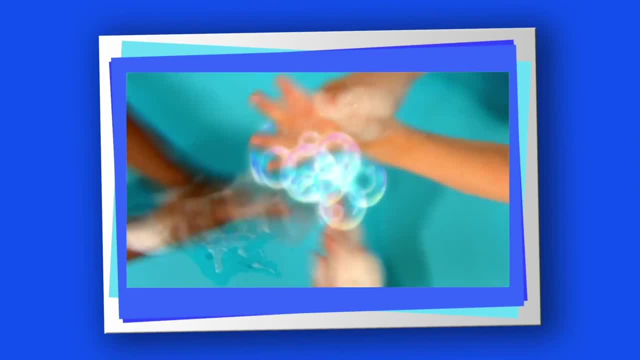 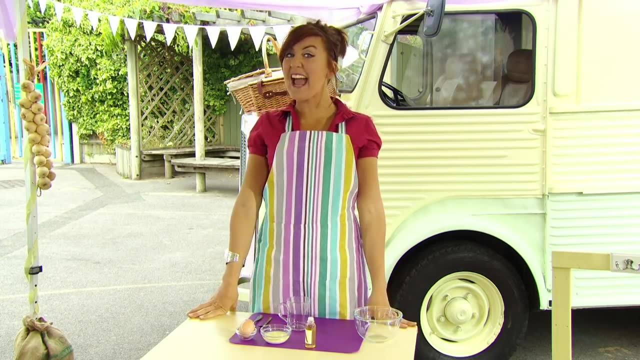 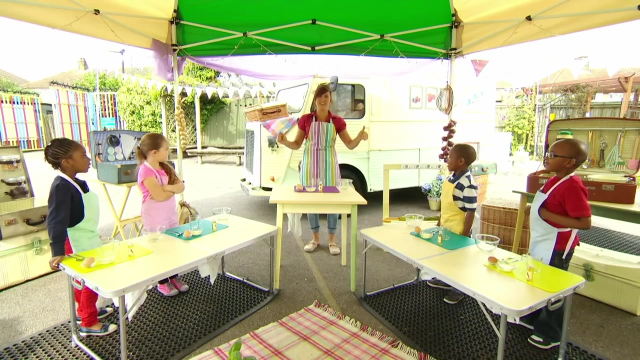 What can you do? I can cook. Let's get started. The first thing we have to do to make our celebration cornet cakes is crack an egg. Now, where do you think eggs like this come from? Chicken? Yes, Let's do the chicken dance, everyone. You put your hands like this and we go. 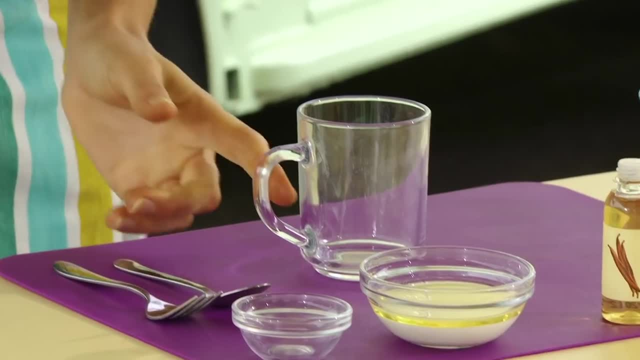 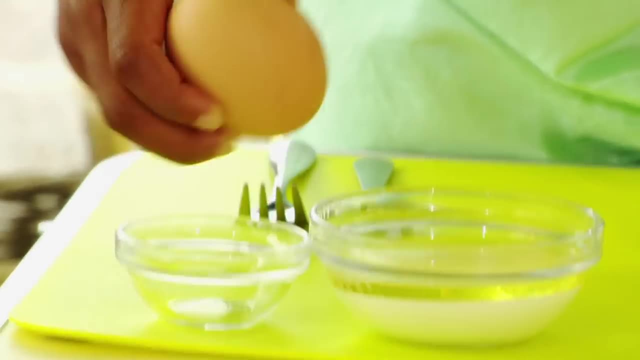 Let's get cracking with this egg. To crack an egg you have to hold the handle of your cup, just like that, and then we need to make a crack in the egg. So we very gently need to knock on the door, Knock, knock, knock until we make a crack. 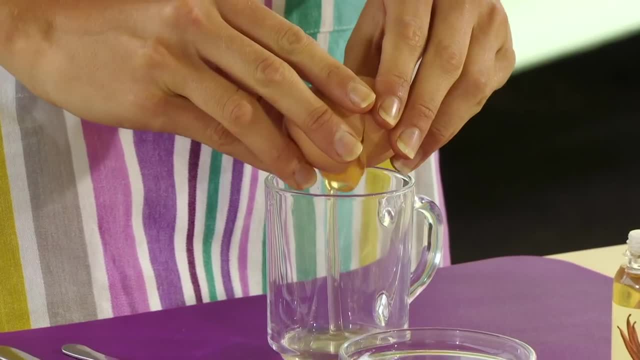 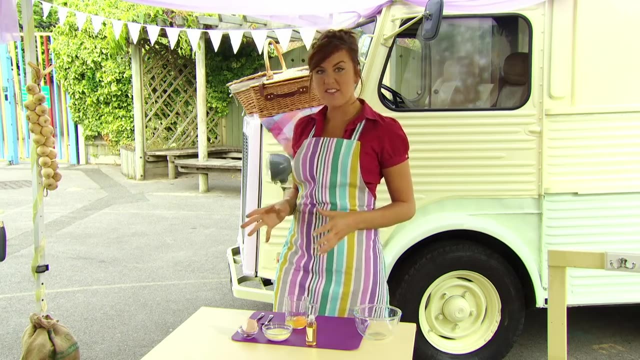 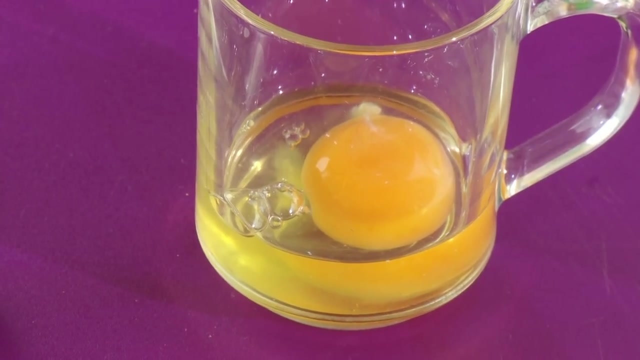 And then very quickly use your thumbs to open it up like this. Watch Ta-da Open up like a door, opening two doors, And the next thing we have to do is separate the egg yolk from the egg white, And the egg yolk is the yellow bit in the middle. Can you see that bit? Yeah, 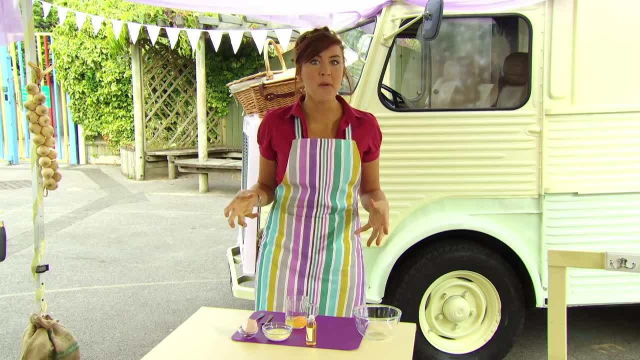 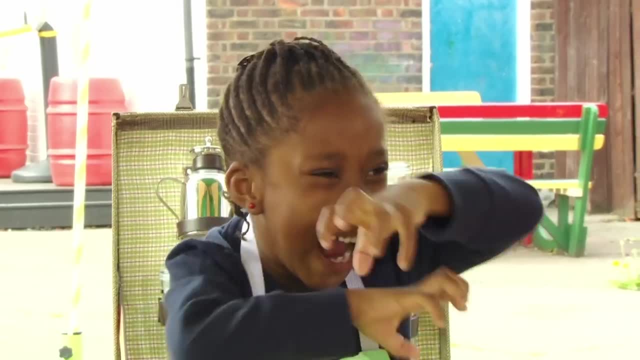 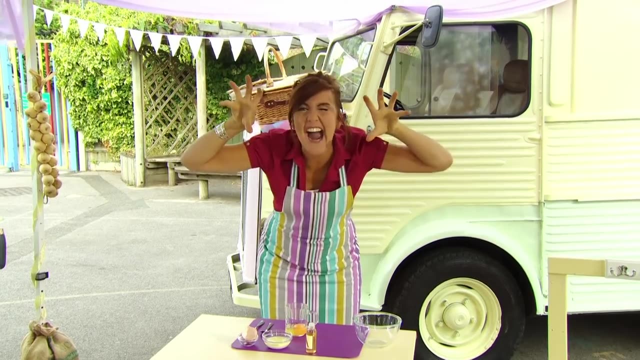 And to help us do this, we're going to pretend to be a monster with big claws like this. Who can pretend to be a monster? Ready, You're very scary. Have you got big monster claws too? Let's see them With our claws, we're going to turn them upside down and then we're going to use one of them. 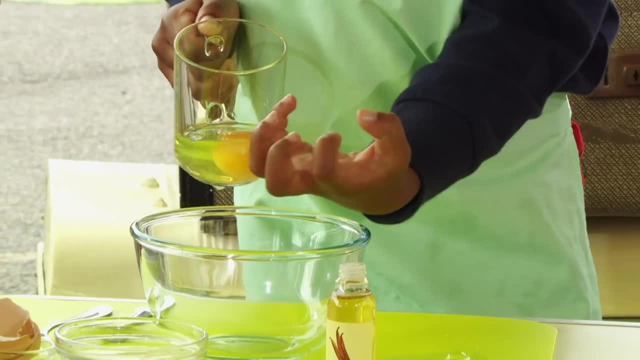 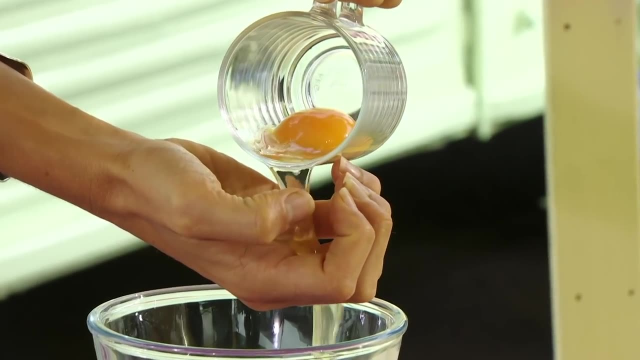 Put your monster claw over your bowl and hold your cup in the other hand and we're going to pour it into our egg. We're going to use our monster claw hand and we want to keep the egg yolk in our hand. Make sure that the yolk doesn't go through your fingers. Keep your monster claw. 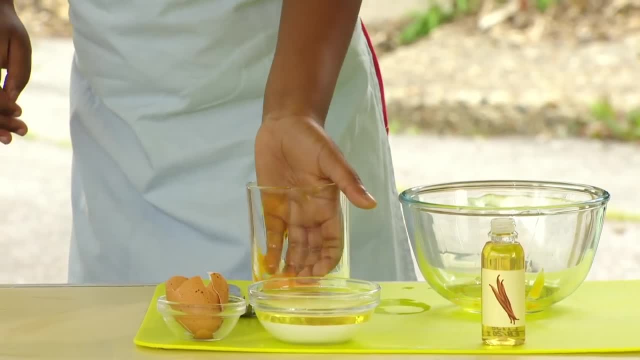 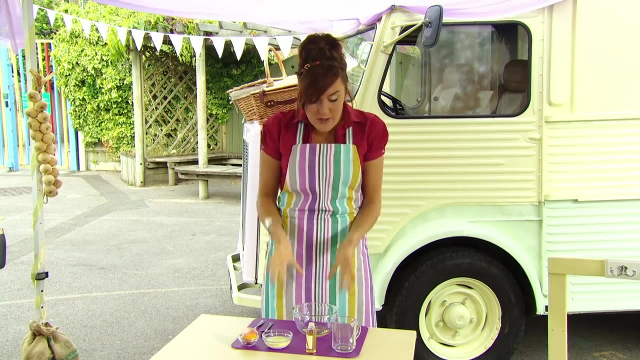 OK, everyone, put your egg yolk into the cup, and now we've done that, let's give our hands a quick wipe. The next thing we have to do is some whisking. We are going to whisk this egg white until we've got loads and loads of bubbles. 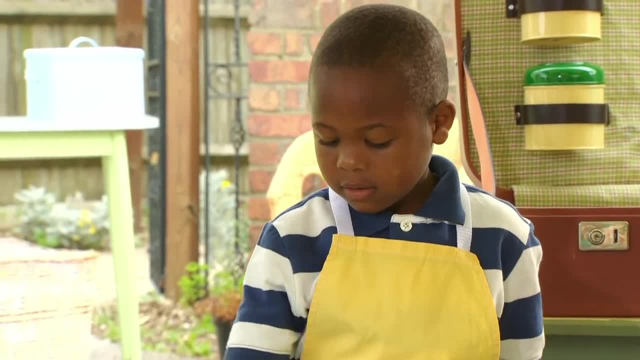 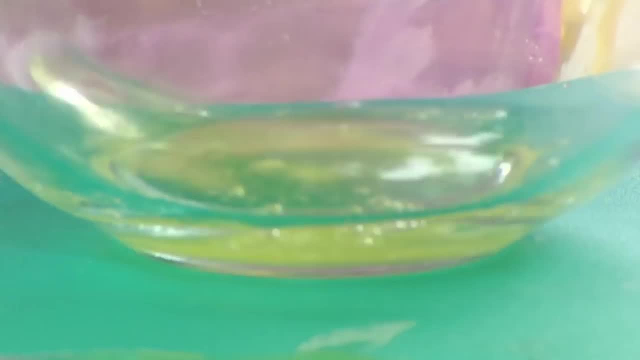 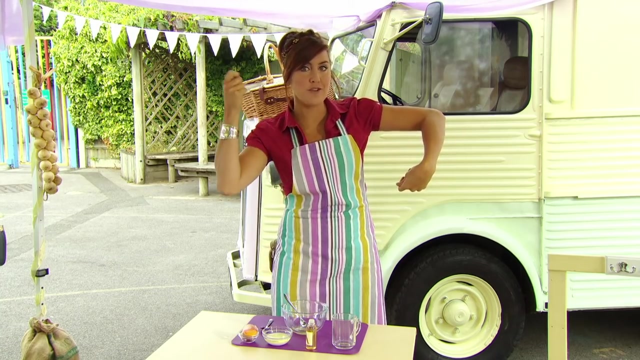 So everybody take your fork, Everyone hold your bowl. Let's get whisking. You need to go really fast, everybody. If you wiggle while you whisk, it actually helps and you can join in. Get your bowl and your fork and whisk and wiggle and whisk and wiggle and whisk, and wiggle and whisk. 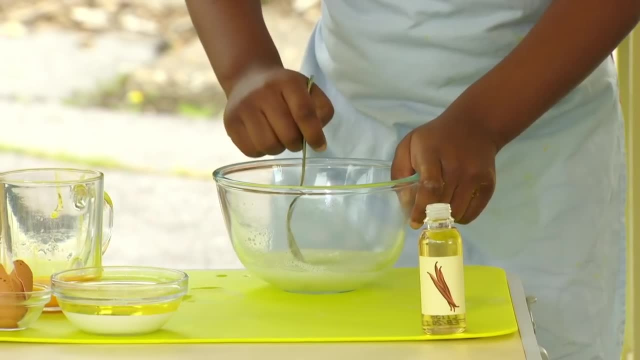 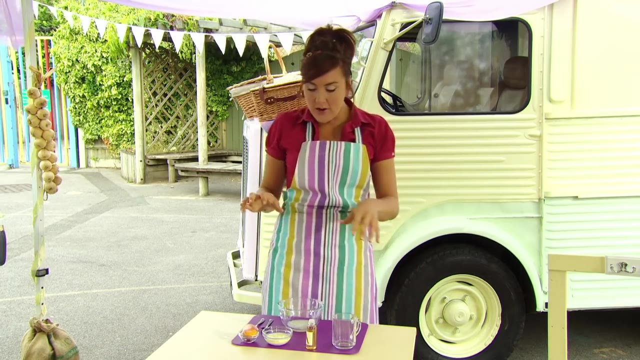 And when you've got lots of bubbles in your egg white we can just stop mixing. I have lots of bubbles, You've got a very bubbly bowl, And to our egg white we're going to add some milk and oil that's already been mixed together for you. 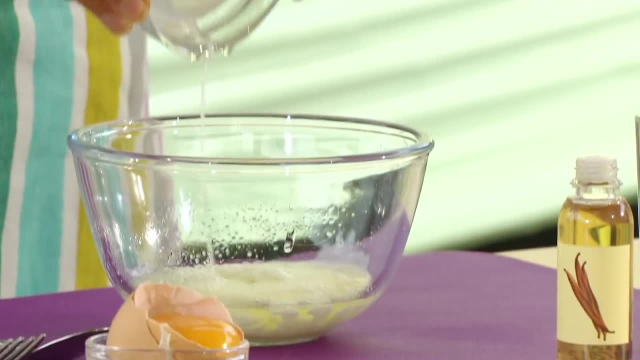 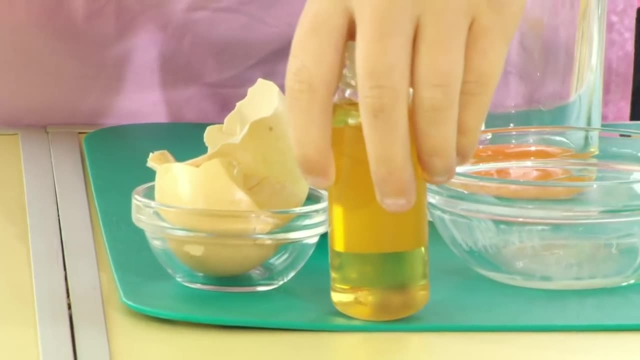 And we're going to add it in with a big splash Ready, Splash, Splash, Fantastic. The next ingredient we need to add is this: It's called vanilla extract and it's got a really strong smell, Anthony. what does it smell like? 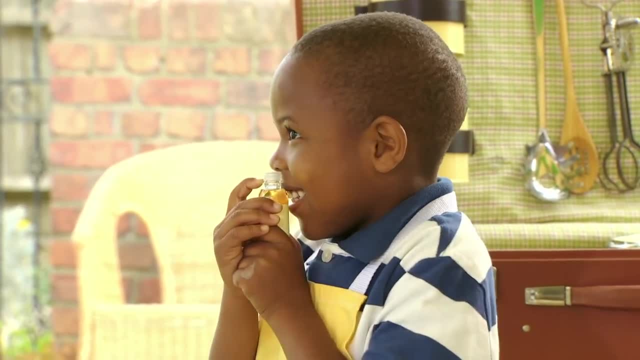 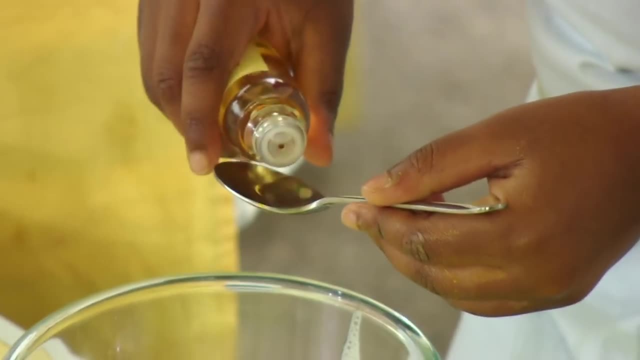 Smells like perfume. Oooh, It would be nice to wear that perfume, wouldn't it? Right, we're going to add half a teaspoon of vanilla extract to our dish. So, everyone, we're going to drip, drip, drip a few drops of vanilla extract onto our teaspoon. 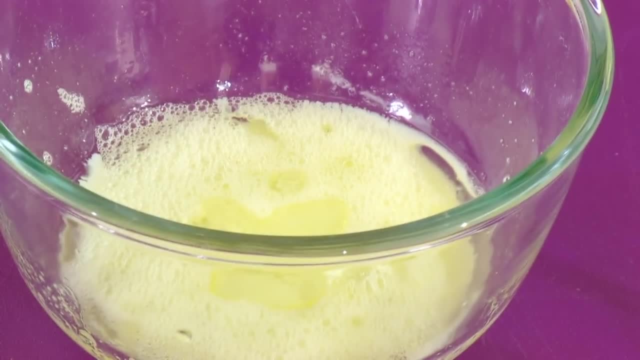 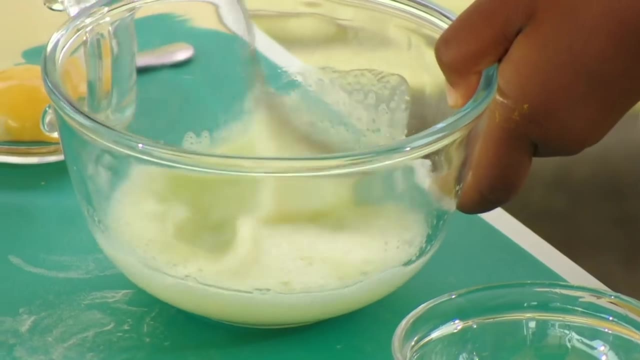 And then we just splash it in Splash And then we finally need to give it one more whisk. A wiggle and a whisk, and a wiggle and a whisk, and a wiggle and a whisk. That's great. OK, everyone, stop whisking. 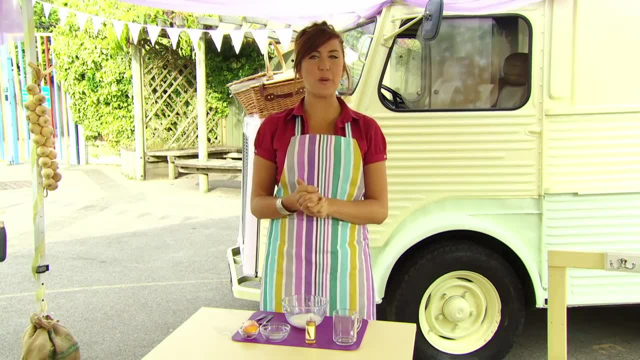 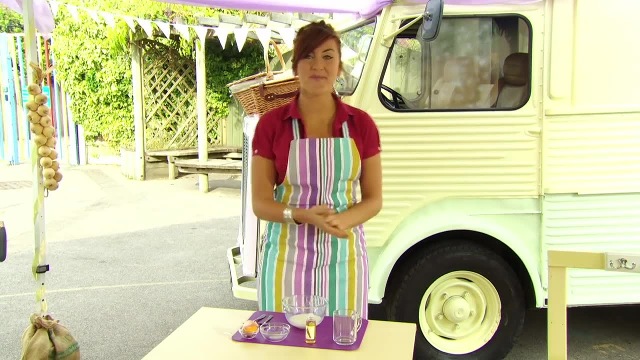 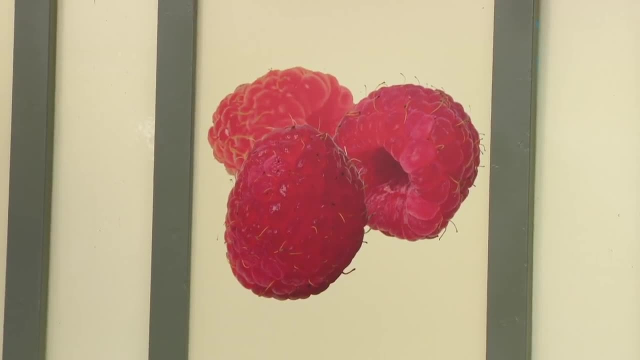 So next we need to add something fruity to our celebration cornet cakes. I wonder what it could be. What is next? Well, let us see if you can guess what it could be. So what have we got? Some cherries, some raspberries and some cream. 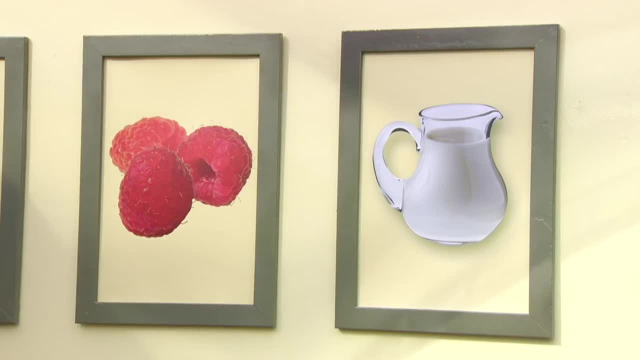 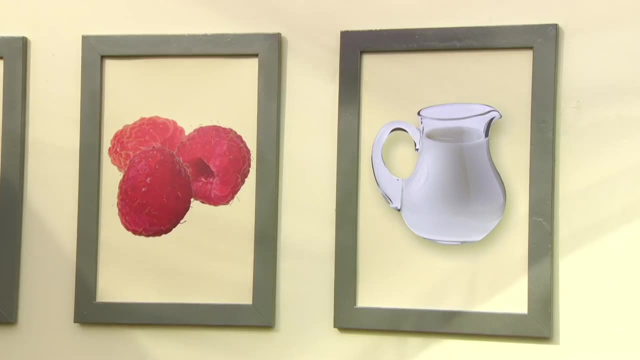 What would you choose for our celebration? cornet cakes. The special ingredient is a fruit. Well, cream's not a fruit, is it? That comes from milk, So we can take that one away. OK, here's another clue for you. 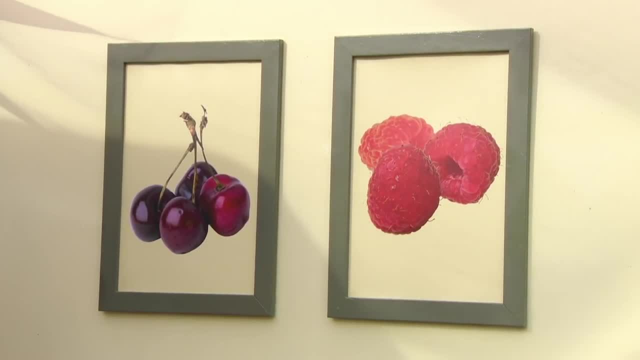 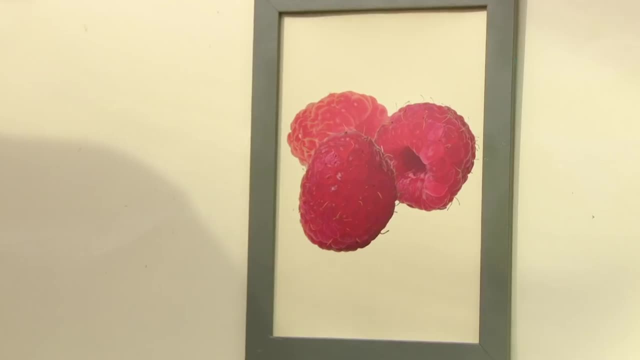 The special ingredient is a fruit, and it grows on bushes. Well, cherries grow on trees, So we can take that one away too, Which leaves us with raspberries. We're going to need some raspberries in our celebration cornet cakes. 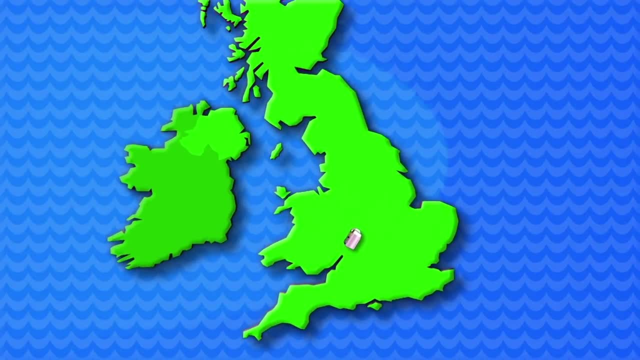 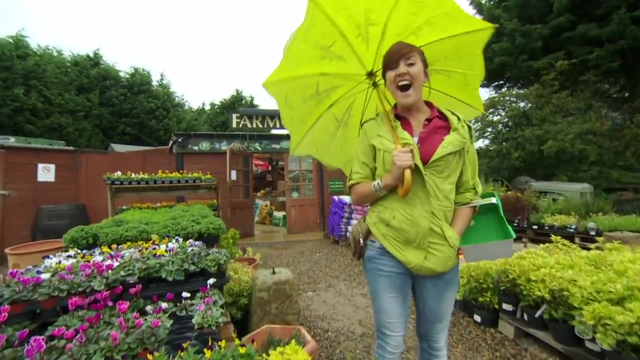 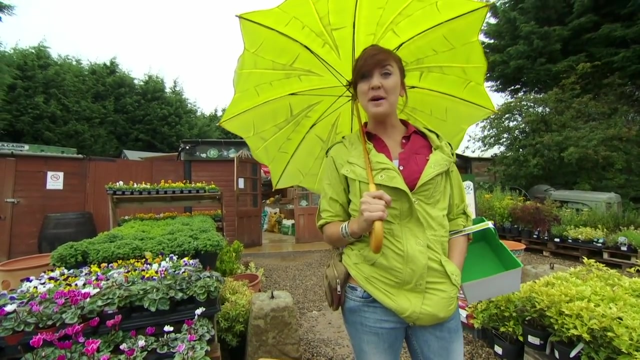 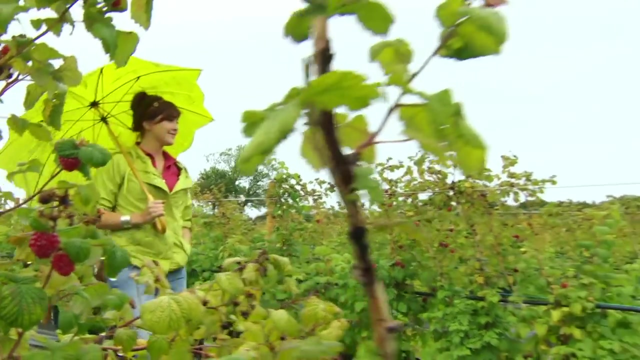 And I went to find some. I've come to Corbridge in Northumberland to find some raspberries, And the raspberries grow here on the farm on bushes. So come on, let's go and find some. When the raspberry grows, it starts off as a flower. 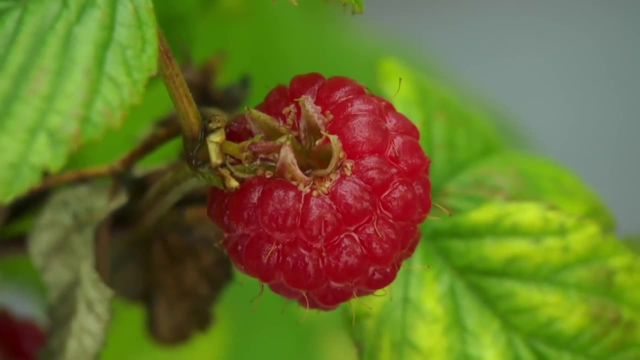 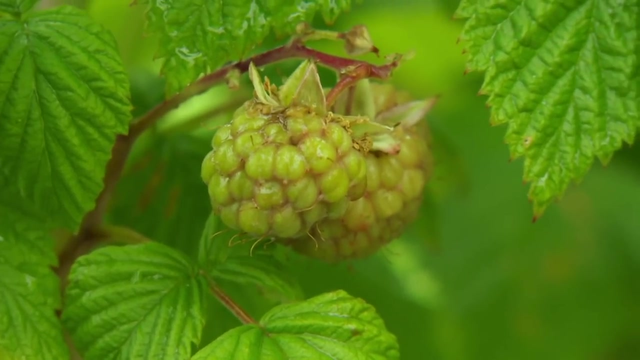 And then the petals fall off and the middle part of the flower grows into a raspberry. When you pick the raspberries, it's really important to check that they're ripe, which means that they're ready to eat. Now, if we look at this one here, it's very, very green and it's really hard. 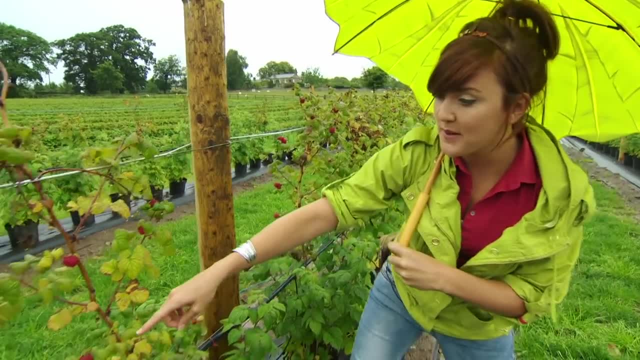 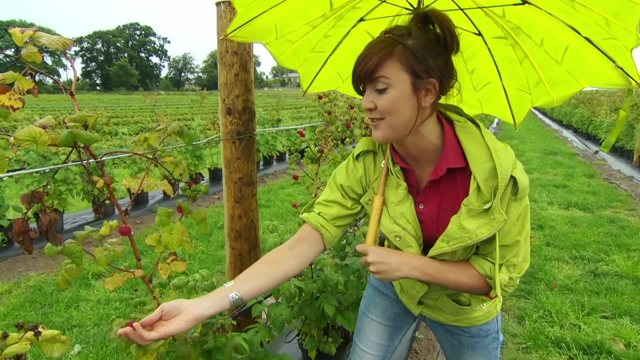 So that's definitely not ripe. Oh, look this one here. that's a really deep red And it's much bigger and squishier and it slides right off. Look at this: That one is definitely ready to eat. Ooh, lovely. 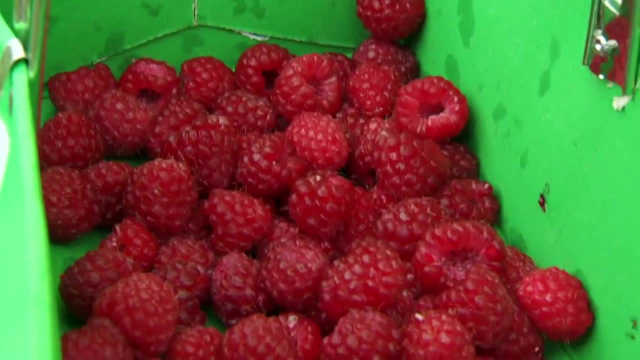 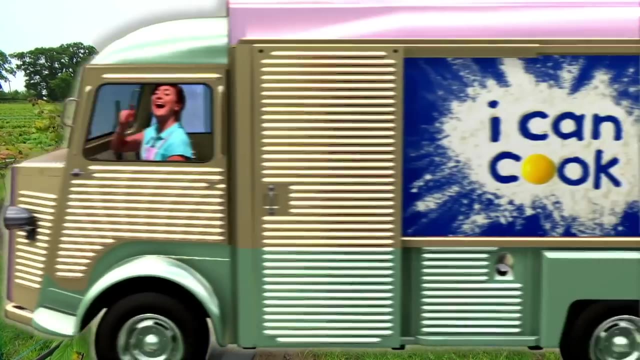 I think that's enough raspberries for everybody. These are going to taste so good in our celebration cornet cake. Let's get them back to the kitchen. I loved picking those raspberries. And look, we've got them here ready to use in our recipe. 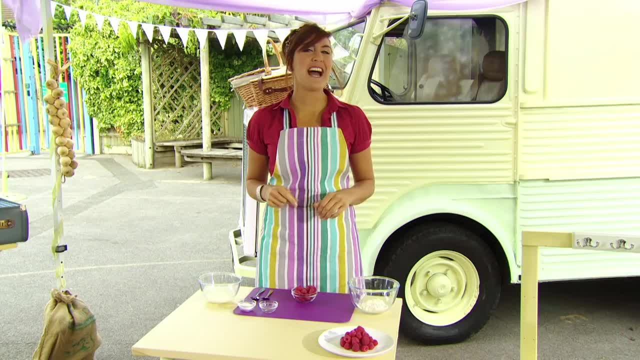 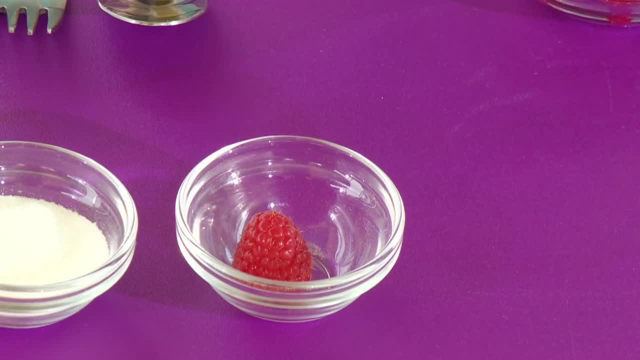 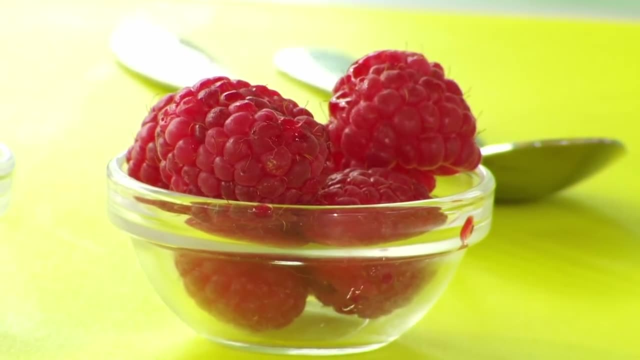 We're going to do some counting with them. first, We're going to count six raspberries into our pot, which we're going to save for later on: One, two, three, four, Five, six. Now we need to put the rest of these raspberries into our bowl with our egg white mixture. 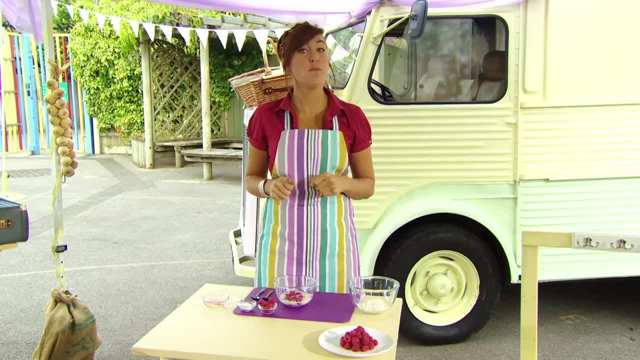 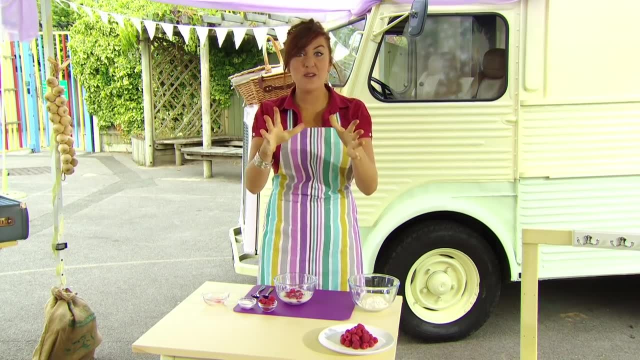 And next we need to do some squishing and some squashing. And you can pretend to do squishing and squashing at home, like this: Squish squosh, squish, squosh, That's it. You squish at home and we'll squish here. 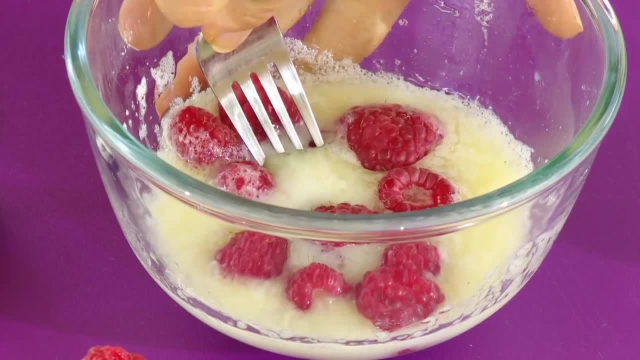 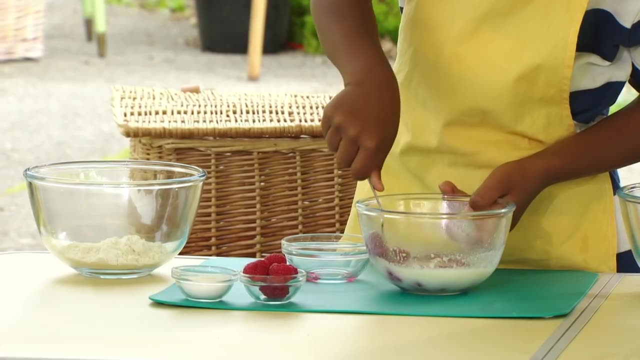 We're going to use our forks to do that, And we can just squish our raspberries against the side of the bowl like this And go Squish, squosh, Squish, squosh, Ooh. what's happening to the mixture? Charlotte? 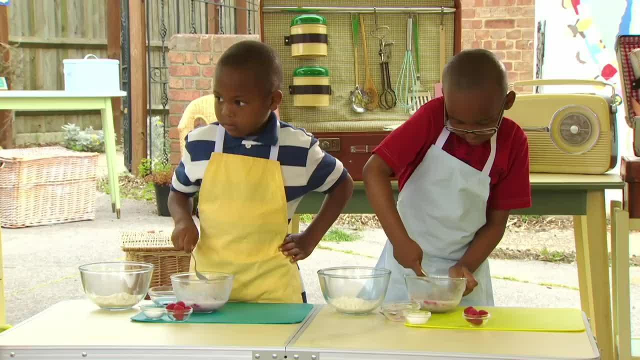 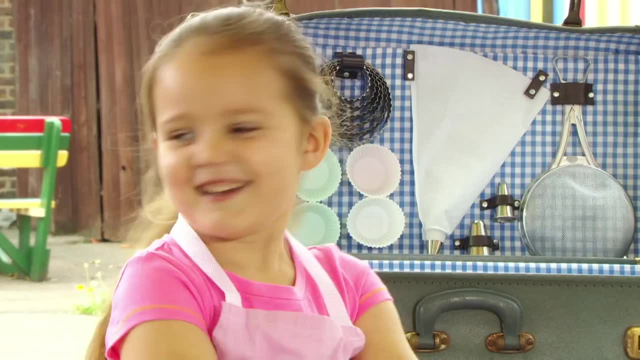 It's going all pinky, Perfect, And put your forks onto your mat Now. everything in this bowl is wet, so we're going to call it the Wet bowl, The wet bowl, And we're going to put the wet bowl to the side for now and use that in a minute. 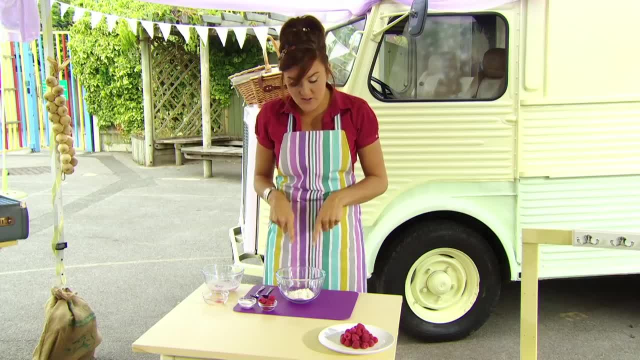 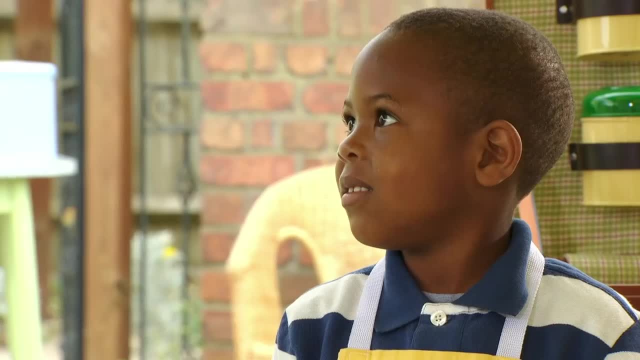 And we're going to bring this bowl over onto our mat. This bowl's got self-raising flour in it, And self-raising flour is magic. Do you know why? Why? Because when you put it into a recipe, it makes everything rise up magically. 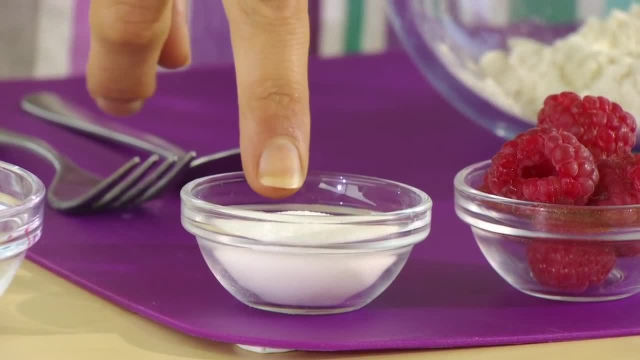 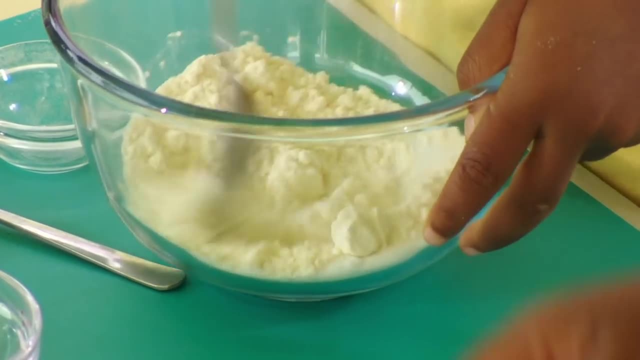 And to the self-raising flour we're going to add some caster sugar. Sprinkle, sprinkle, sprinkle. I sprinkle now. Now, everyone, use your fork to give your self-raising flour and your caster sugar a quick mix, Easy peasy. 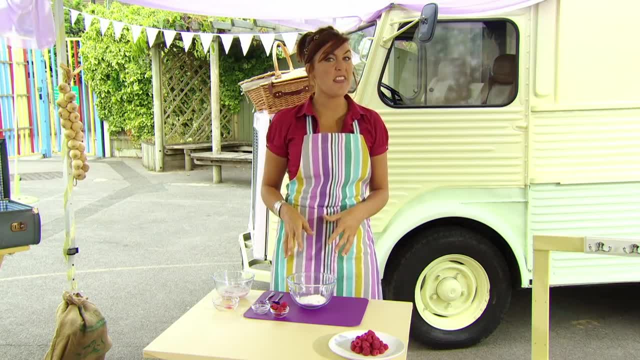 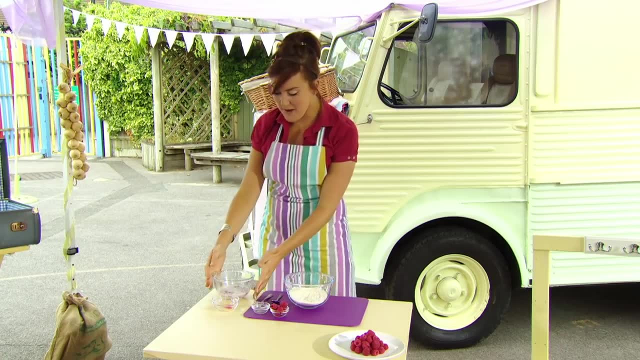 And because everything in this bowl is dry, we're going to call it the Dry bowl. You got it, team. The next part is a fun part of the recipe. We're going to take the wet bowl and splash it into the dry bowl. 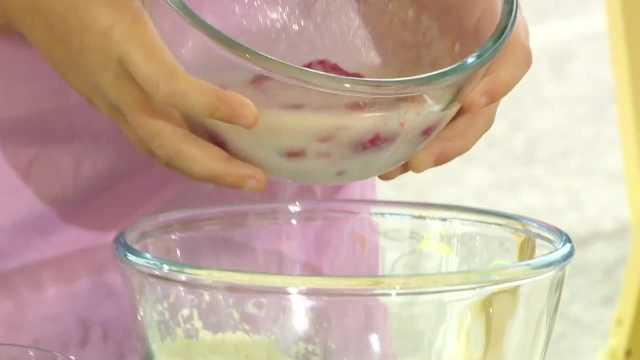 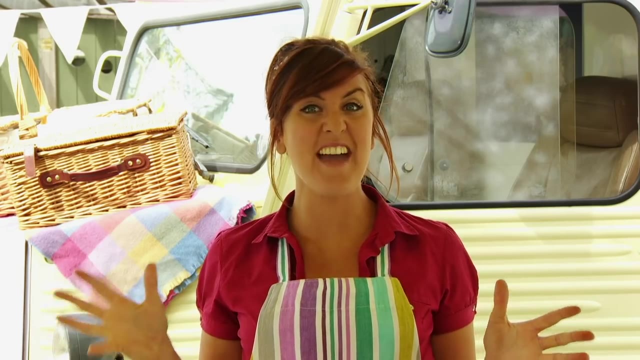 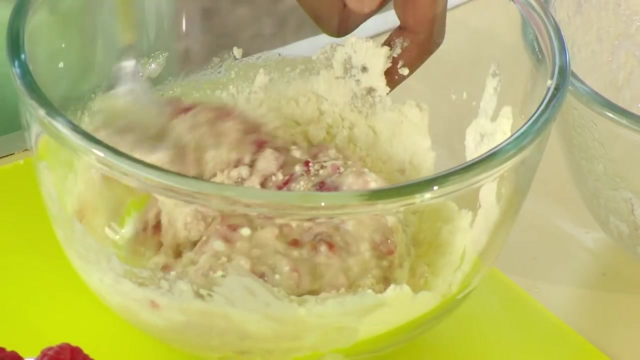 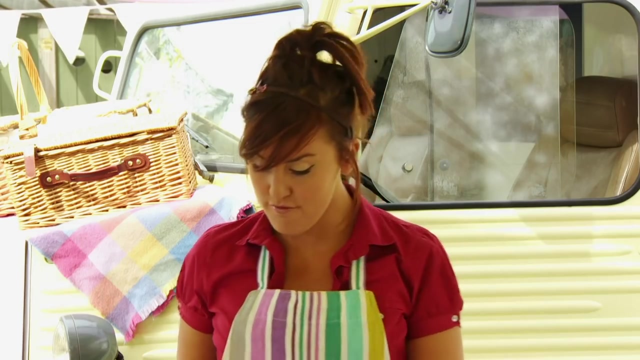 One, two, three, splash, Splash. Ooh, That one looks like a river. It does, So let's give everything a giant mix, Giant mix, And keep going until all the flour has completely disappeared. Next, we'll need three of these. 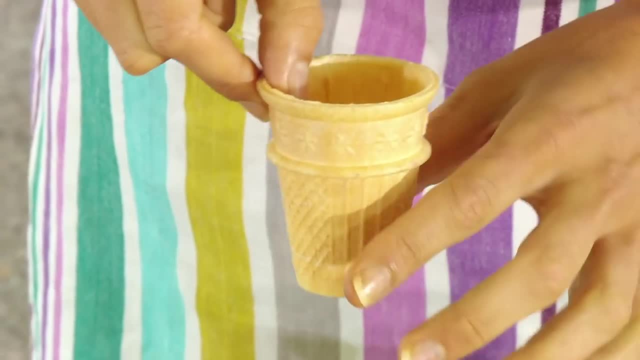 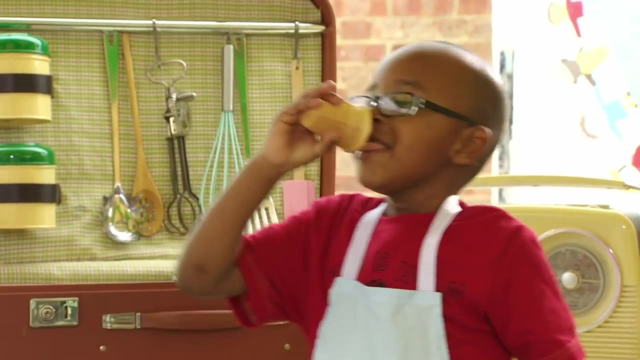 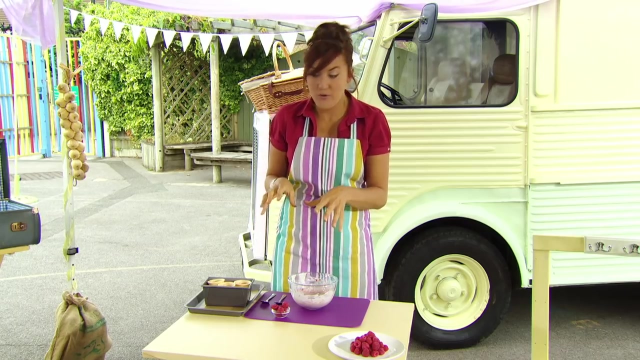 They're ice cream cornet cups. Shall we pretend to lick an ice cream Ready Mmm? Now we're going to do something a little bit secret. We are going to put a raspberry at the bottom of each of the wafer cups. 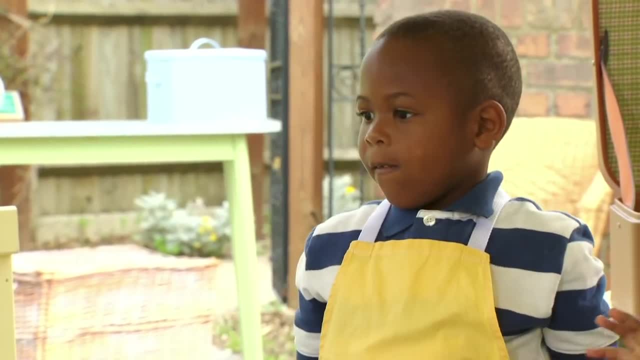 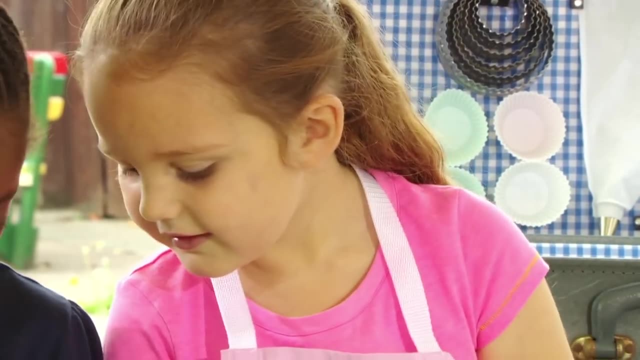 so it's a surprise when we eat them later on. So take a raspberry and put it into the bottom of this one, and then one into the next one, and one into the next one, And next we're going to play the two-spoon game. 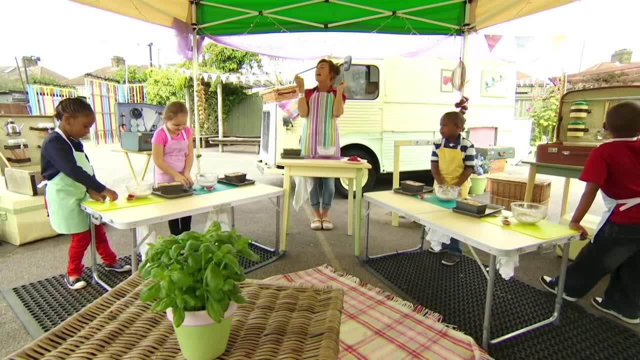 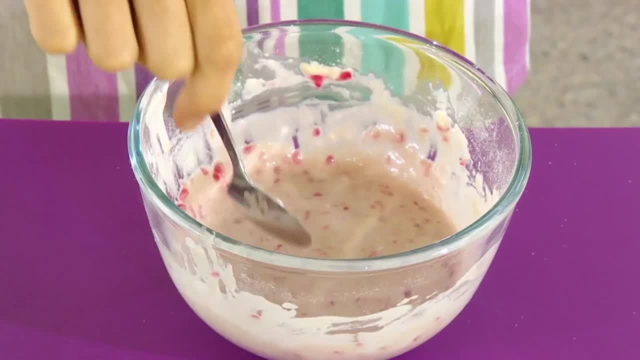 So we need our two spoons. My spoons are called John and Millie. Everyone say hello John and Millie, Hello, John and Millie. Now to play the two-spoon game, one of the spoons has to scoop up the mixture like this: 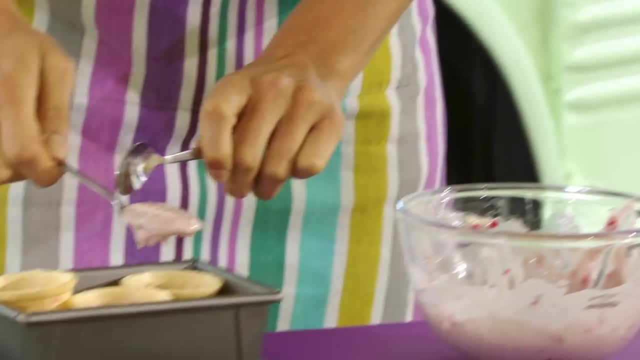 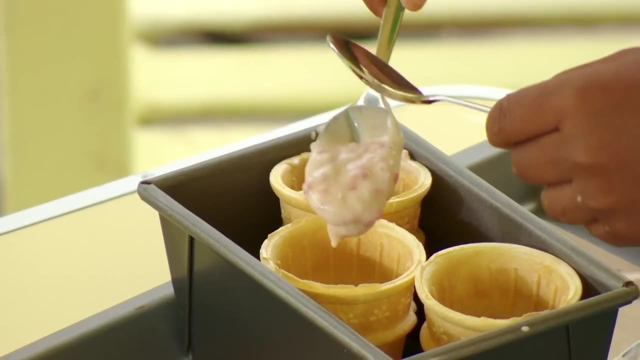 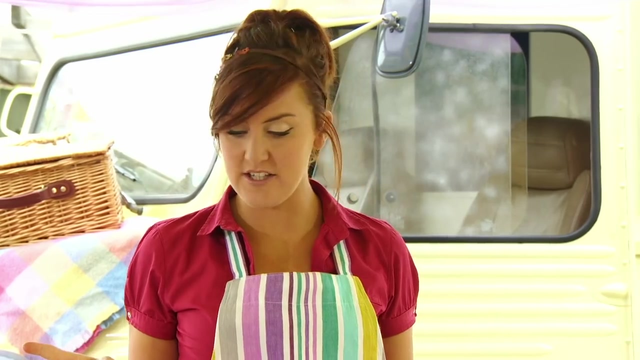 and then the other spoon has to slide it off, Slide. So we scoop and slide, Scoop and slide, And we keep doing that until we've used all of our mixture up And the final thing we need to do is add these three raspberries on top. 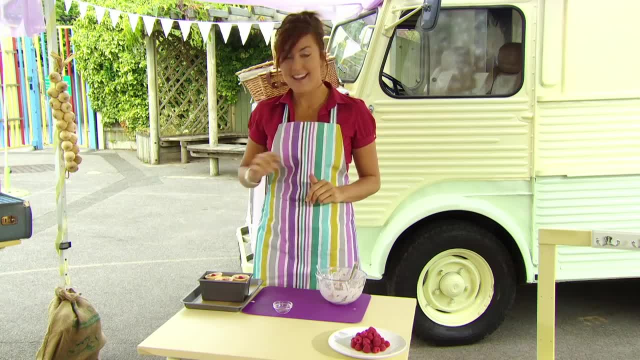 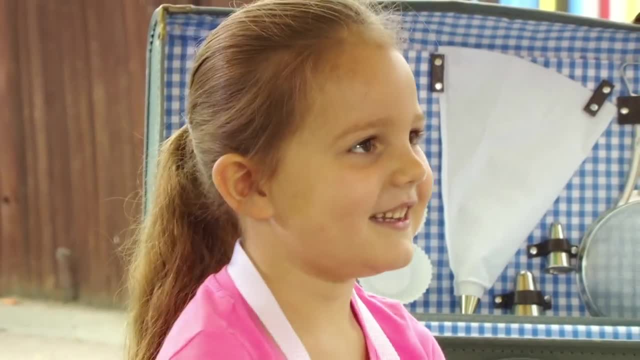 Done it, Done it. Ah, they look great, And that's it. You've done it. You've put all the ingredients together for your celebration course And now you can prepare for your celebration cornet cakes all by yourself. Now it's time to put them in the oven to cook. 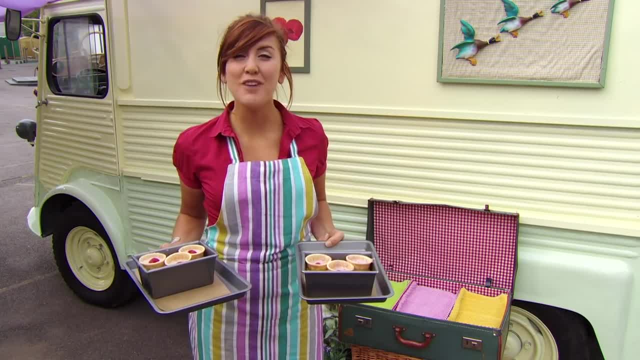 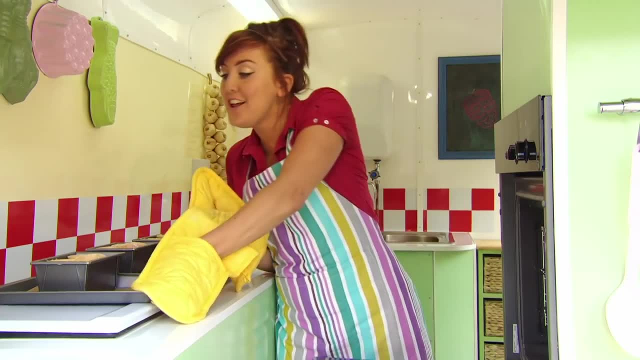 But remember, ovens are hot, so don't go near. Ask a grown-up to help you here. Now we've cooked with you and had lots of fun. Let's tidy up and think of all the things that we have done. There was. 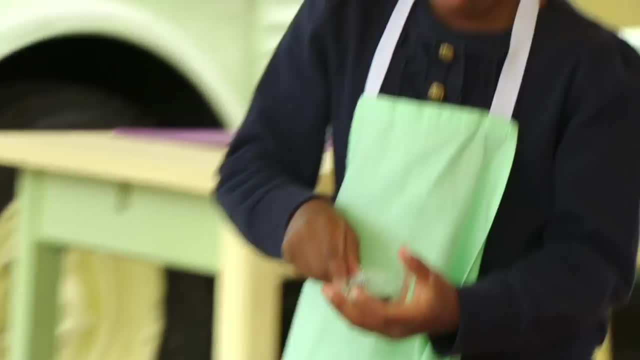 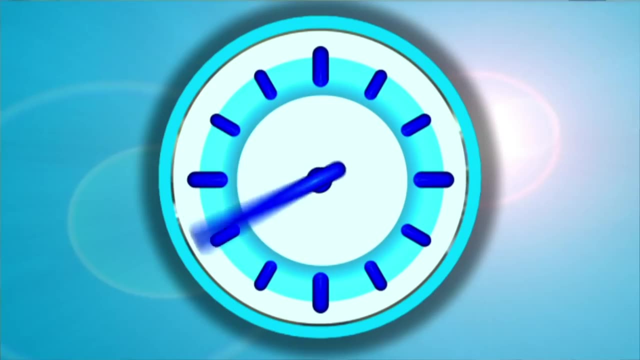 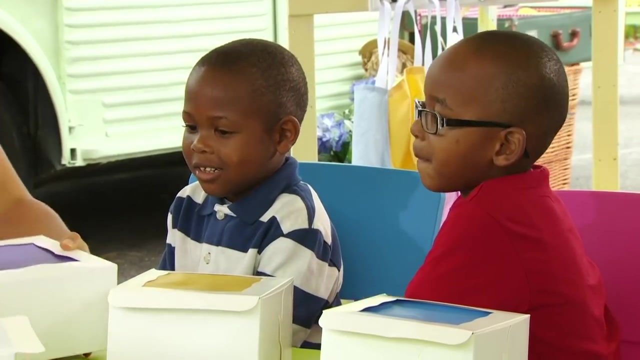 Cracking, Pouring, Scotting, Clearing any mess And putting things away. It's always fun to do at the end of the day. And here are your celebration cornet cakes, and they're all cooked. OK, let's have a look at Charlotte's. 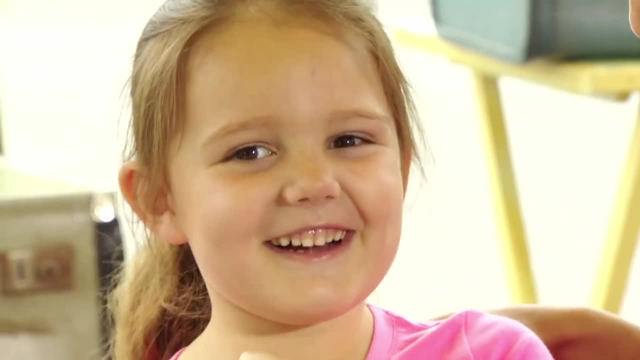 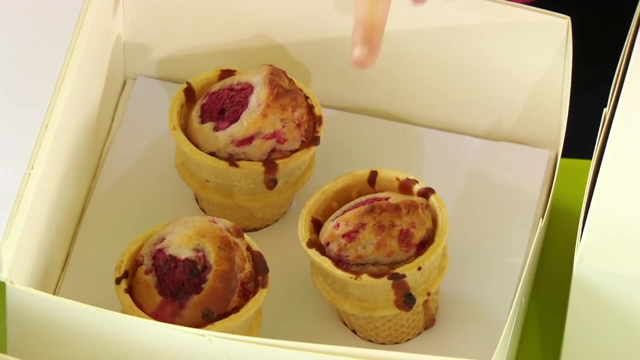 Wow, They smell like raspberries. They certainly do. That's because we've got lots of raspberries in them. And what's happened to the raspberries on top, Charlotte? They've squashed them. They've squashed. OK, everyone, let's put our lids on. 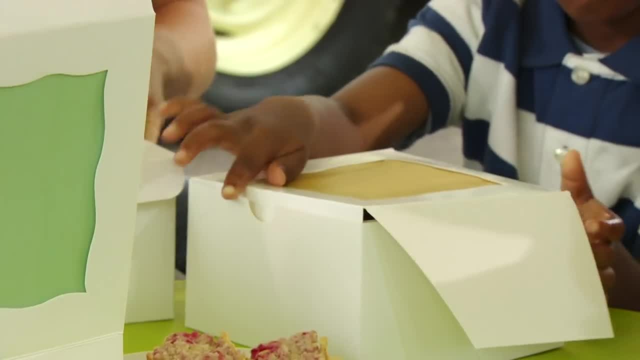 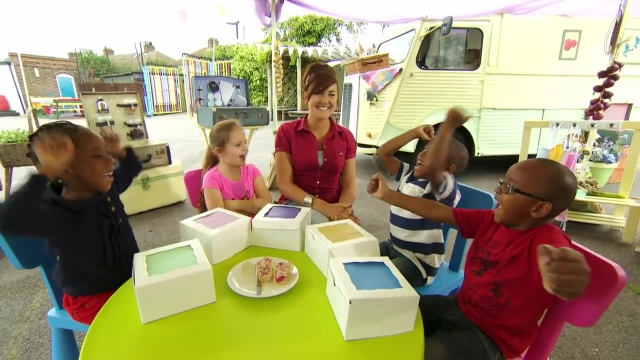 and we'll save our celebration cornet cakes for later on. We've travelled to you, we've cooked and had fun. Now let's have a party with everyone, Yeah, And you can come with us, so follow me. Come on, everyone, bring your cakes. 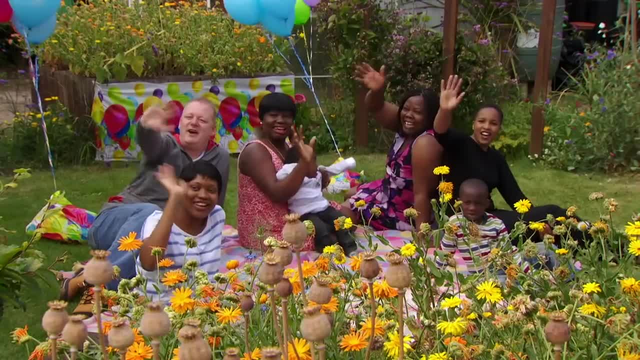 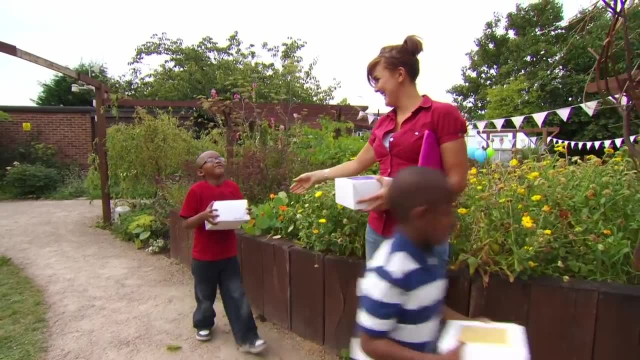 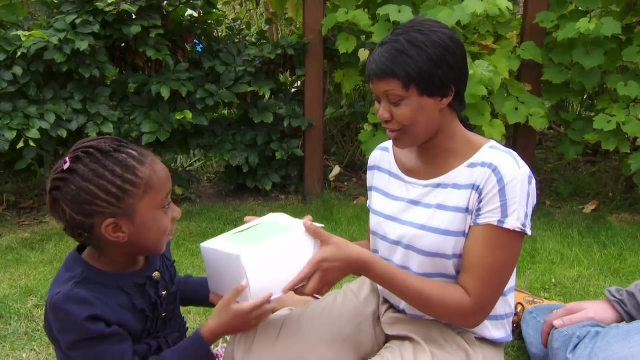 Oh, look, there's everyone over there. Hi, Hello, Has everyone got their food ready? Yeah, Well, come on, then Let's go and join in. Oh, that's a lovely box. Let's see what's inside it. 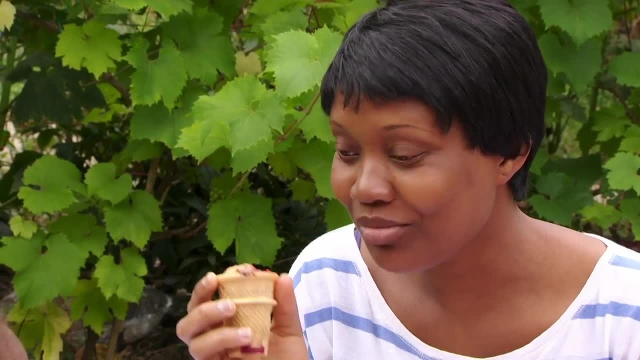 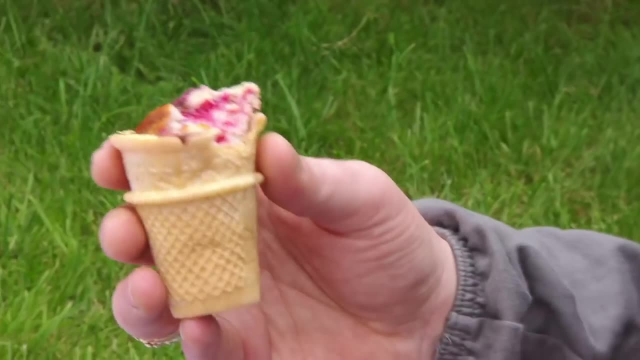 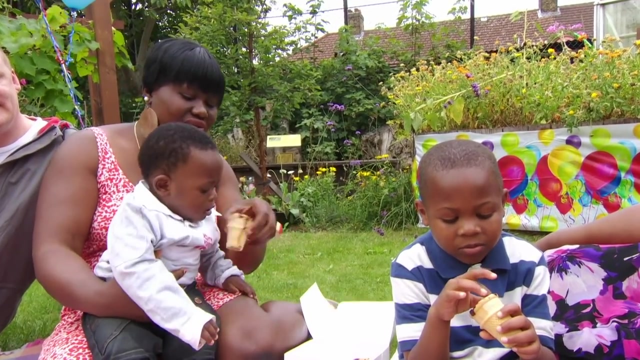 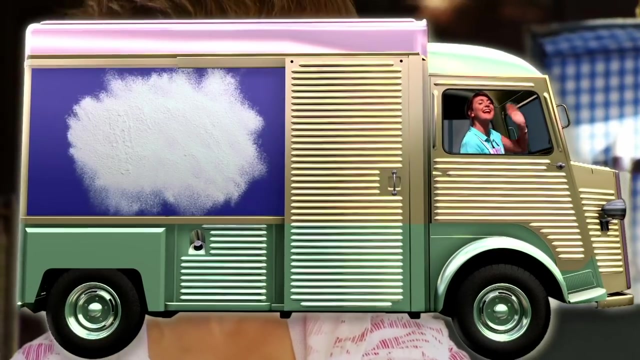 Let's taste it. Mmm, Very yummy. Wow, they look really nice. Mmm, Raspberry, Mmm, It's really lovely. Do you want some, Emmanuel? So what can you do? everyone, I can cook. I can cook. 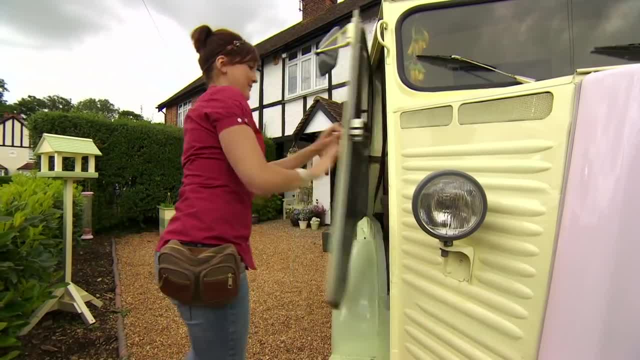 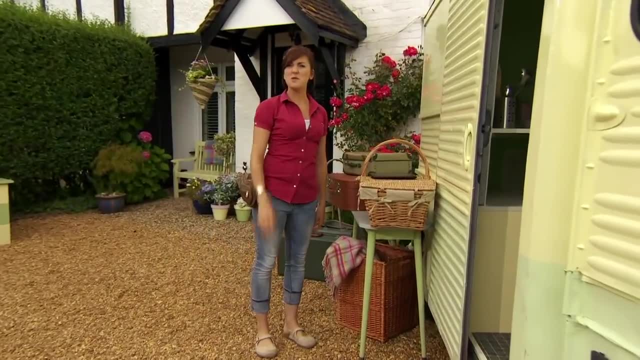 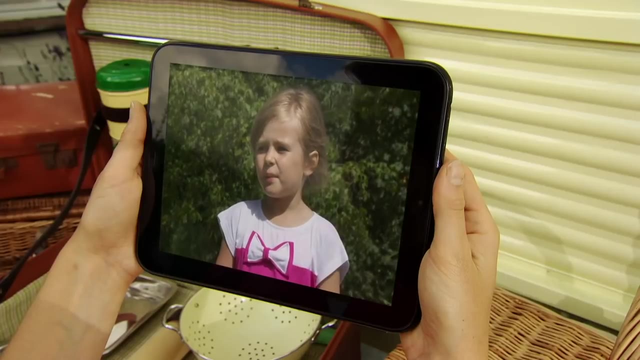 With you. Oh, great, Great. I was hoping you would come. I've just been getting everything ready to go on a journey and I hope you'll come too and meet some new friends. Katie, I love walking my dogs along the river. Can you help me make something? I love fish. 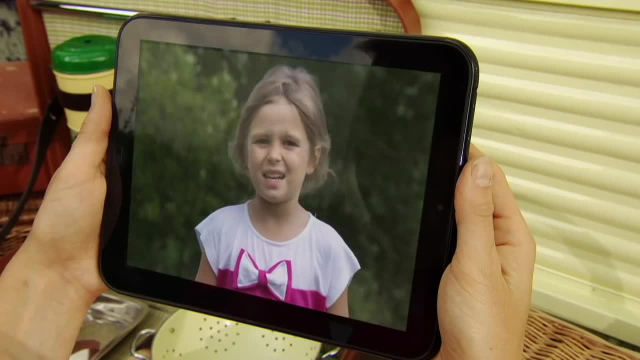 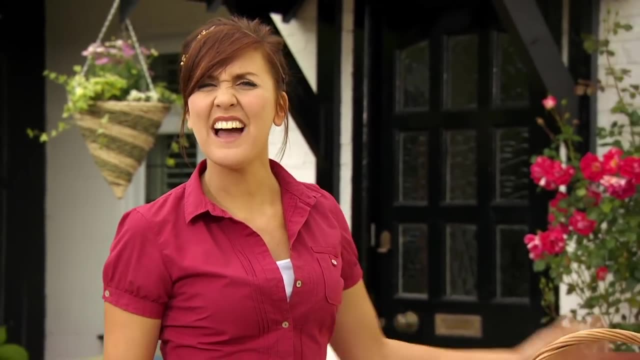 Definitely that will be so much fun. Katie, can you cook with me please? I certainly can, Great, and you can cook with me too, and I love dogs, so this is going to be fantastic. I just need to get all of this packed into the van and then we can get going. 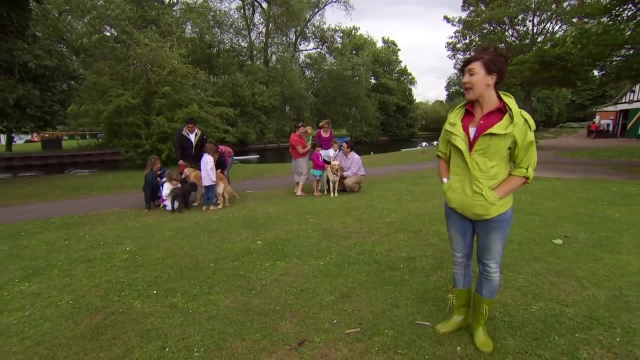 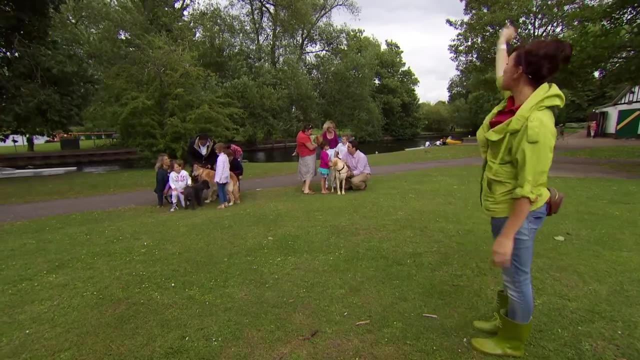 Well, here we are, down by the river where I've been invited by Ami. Oh, look, and there she is with all of her family and friends and her lovely doggies. Hello everyone, Hi, Hi, Ami, Oh, great to meet all of you. So what's your name? 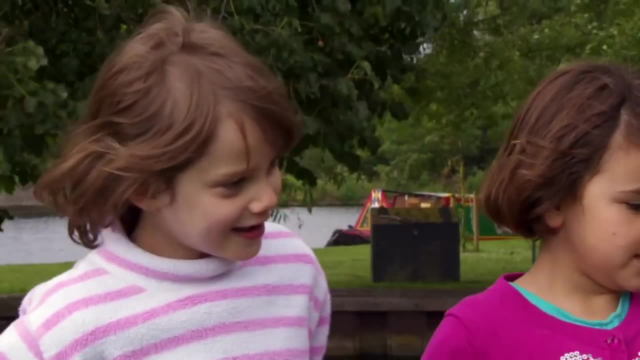 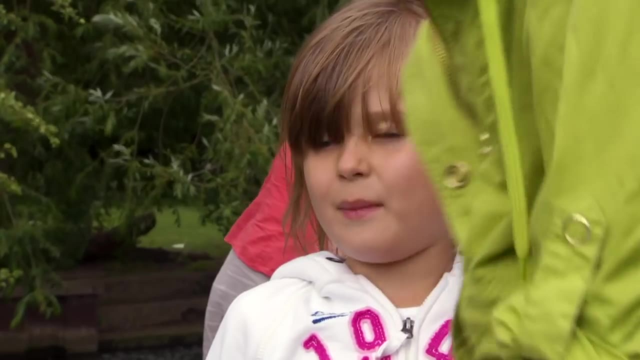 Otti, Samba Me, Nora, Fantastic to meet all of you. So, Ami, what are we going to be doing today? We'll be cooking some food for when we give our dogs a walk. Brilliant, Well, I have got the perfect thing to cook with all of you. Come on, follow me. 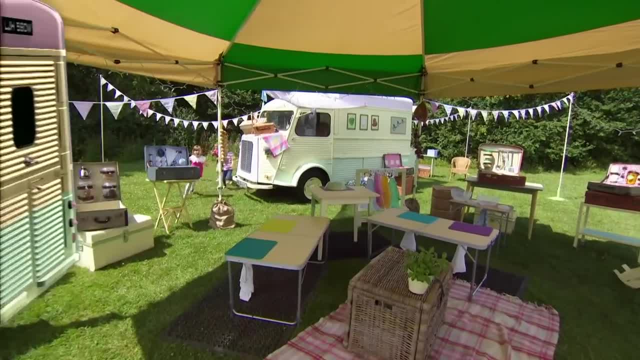 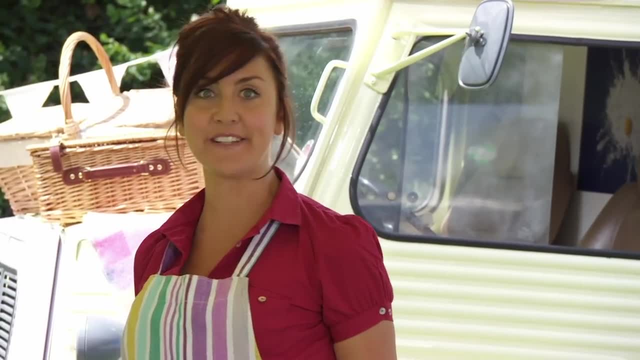 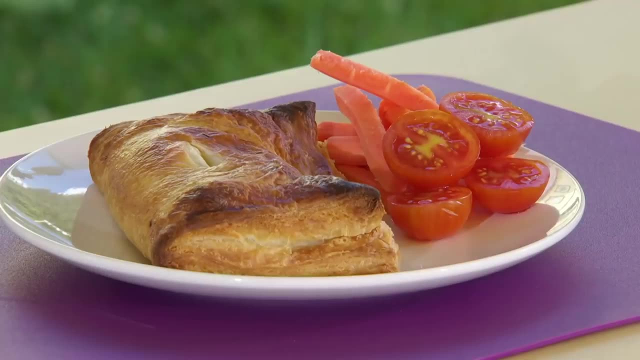 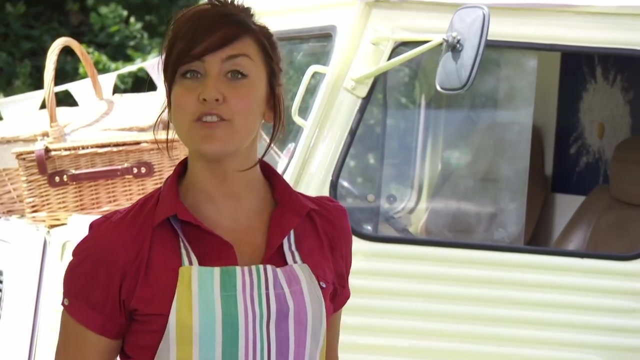 Welcome to my outdoor kitchen. Now, who wants to know what we're going to cook today? Me, Well, today's recipe is delicious: It is haddock puff. Now, doesn't that look good, girls? Yes, Can't wait to make it. but before we do make it, we've got to do something extremely important. What do you think it is? 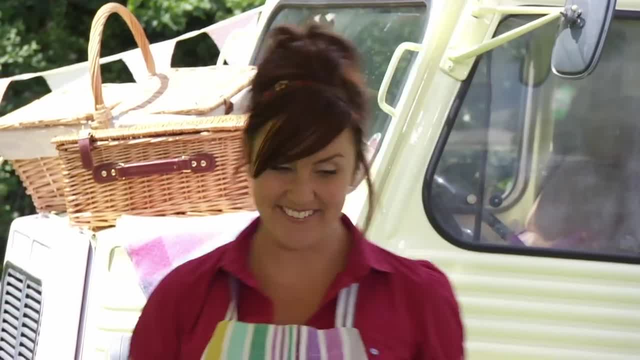 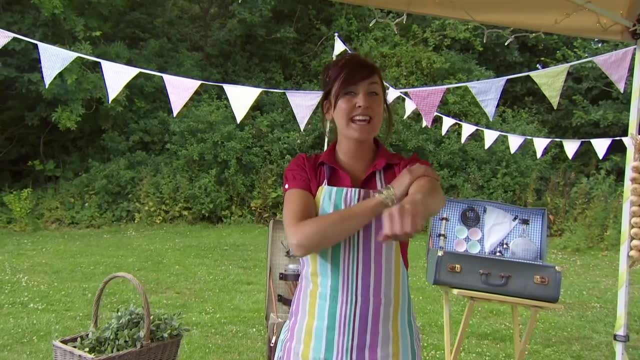 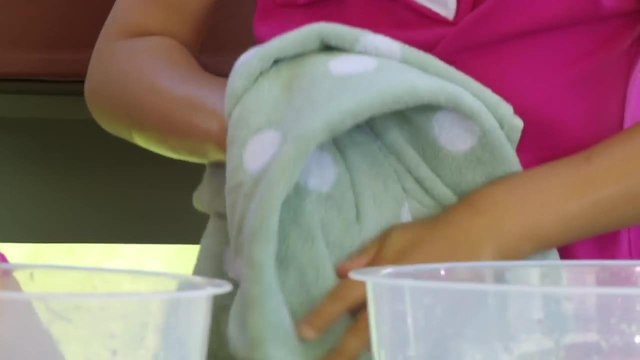 Wash our hands. That's right, Let's get going. Roll up your sleeves, Give your hands a wash with slippy dippy soap, Splish, splash, flush. Have you done your hands Washed and dried, Sleeves rolled up, Apron tied? 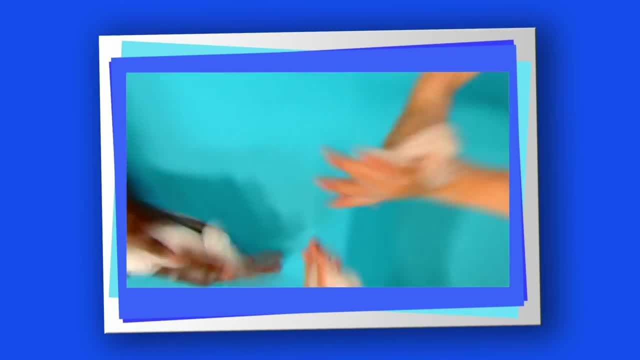 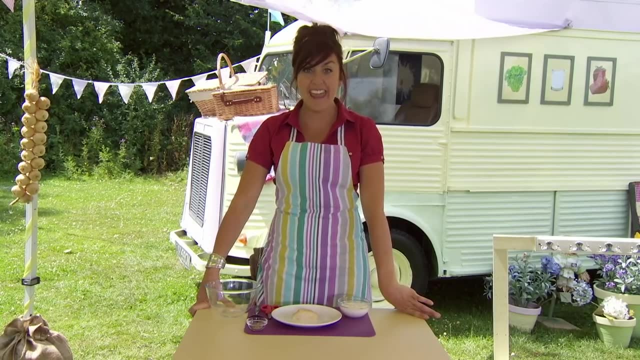 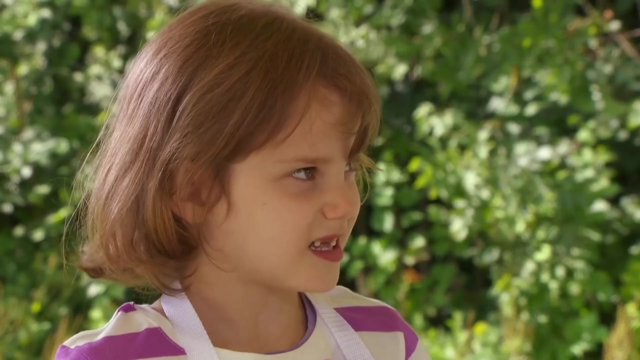 What can you do? I can cook. Let's get started. The first thing we need for our haddock puff is haddock. Now does anyone know what haddock is Fish? Yes, that's right, It's a fish. Can anyone do a fish face? How about this one? 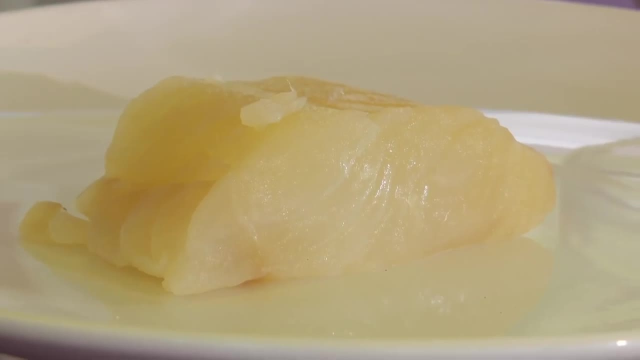 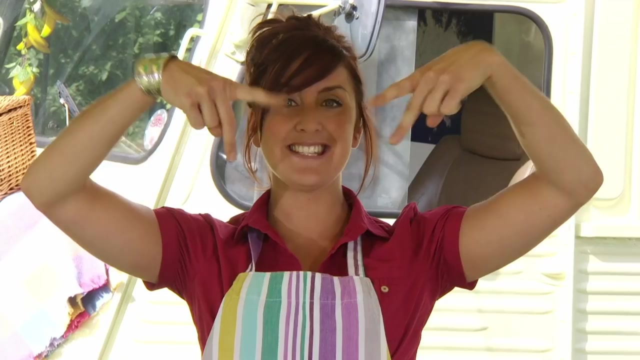 That's a good one. So the first thing we need to do is snip our haddock up. Can you snip, snip, snip with us like this: Snip, snip, snip, Snip, snip, snip, snip. 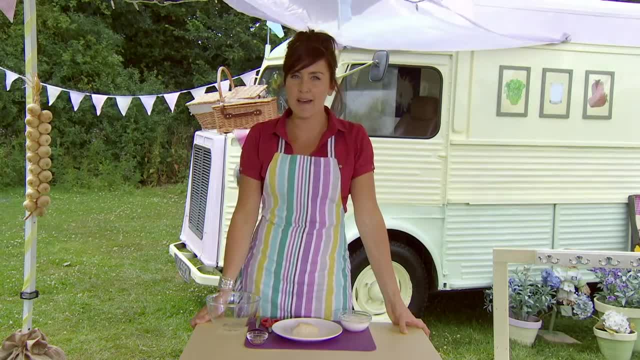 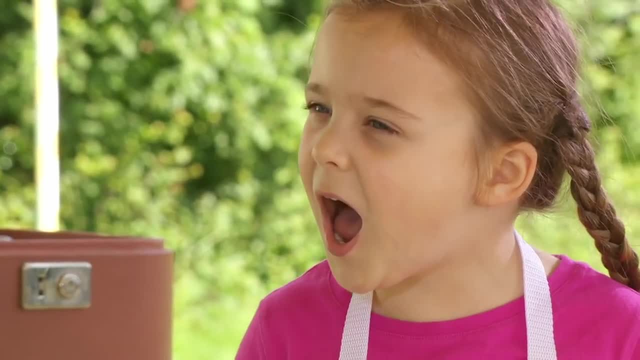 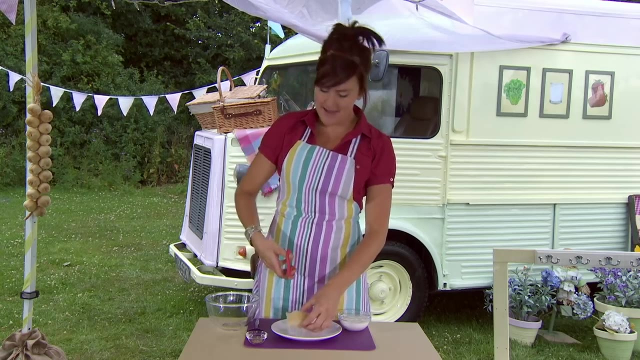 Now we're going to use our scissors, but remember, be safe with scissors. Everybody knows you point them down towards your Toes. That's right, team. We need to get our scissors and point them down towards our toes and let's get snipping. 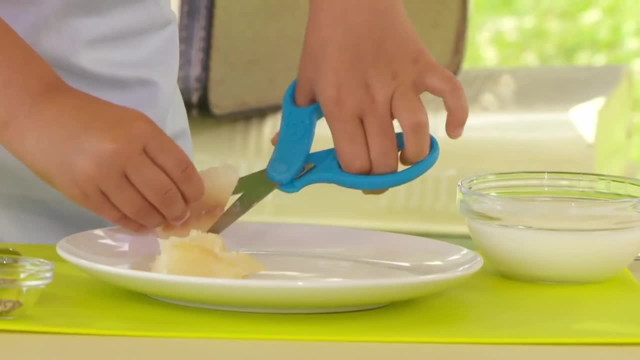 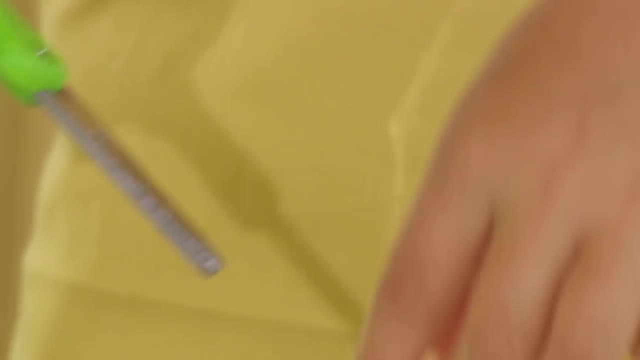 Ooh, the fish feels really funny. I know, I know What does it feel like? It feels like it's squishy Squishy. Yeah, I've done it, That's it. And when you've finished snipping, we're going to put our haddock pieces into a bowl. 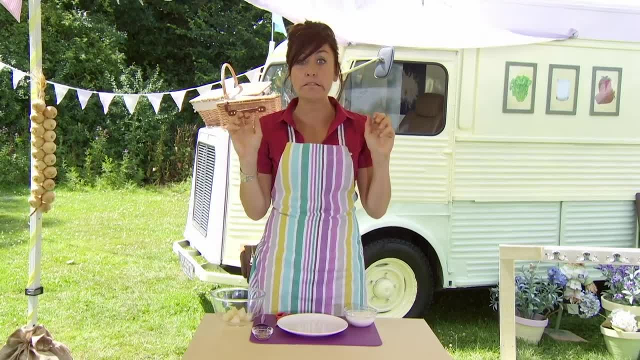 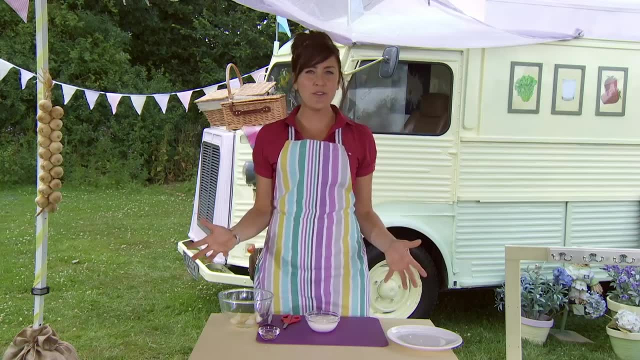 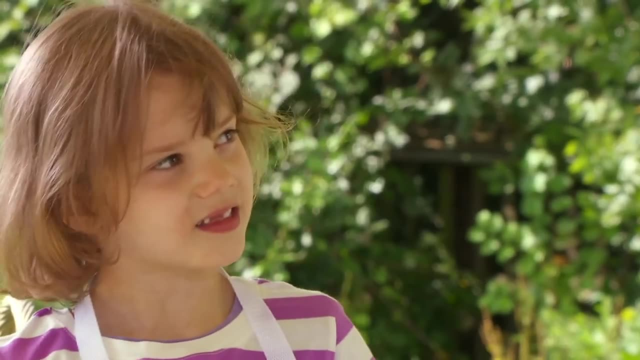 Brilliant And then give your hands a little wipe because they're a bit fishy. Now, the next ingredient we need is creme fraiche. Now, does anyone know what creme fraiche is? Cream? That's right, Leonora, It's a type of cream, So we need a tablespoon of creme fraiche. 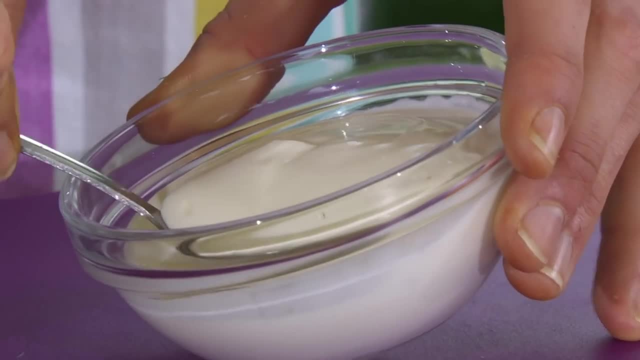 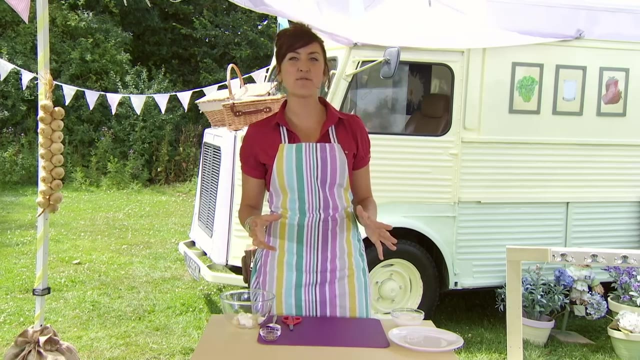 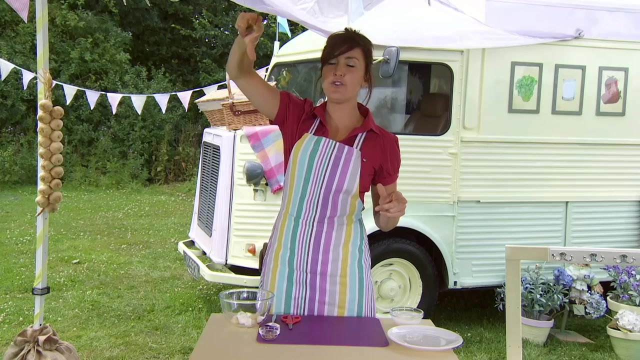 So let's take one big tablespoon and then we're going to put it into our bowl And the next thing we need to do is bring out our pinchy parrots. You get your thumb and you put it down like that, and then you put your two fingers on top and you go. 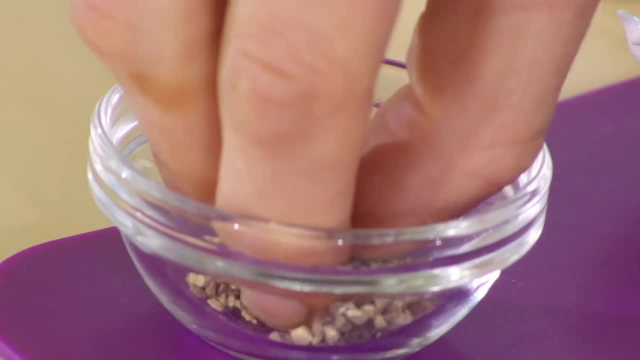 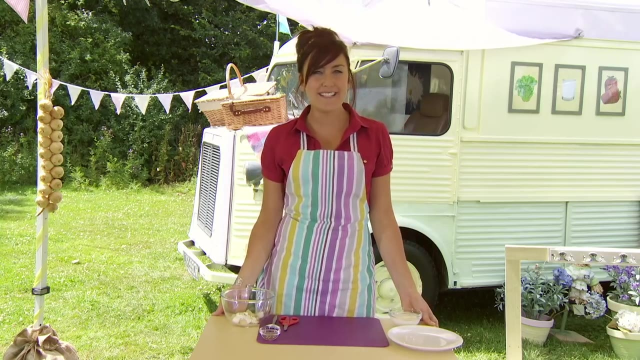 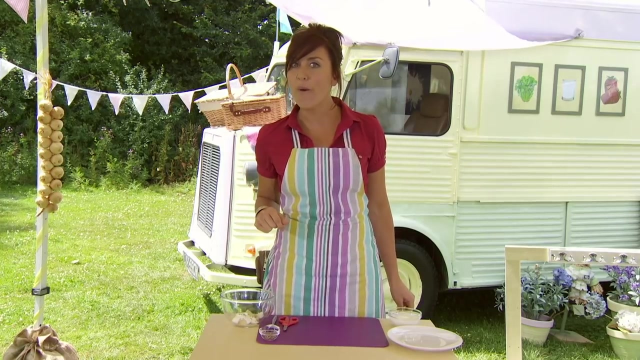 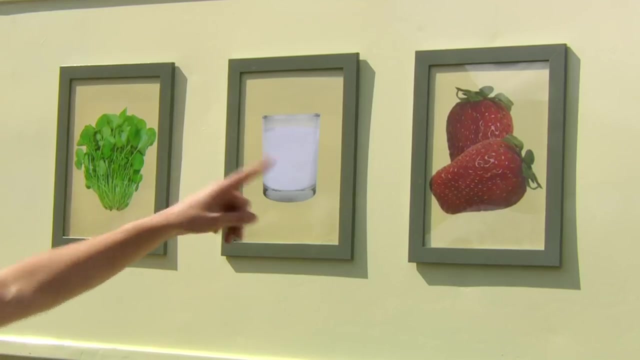 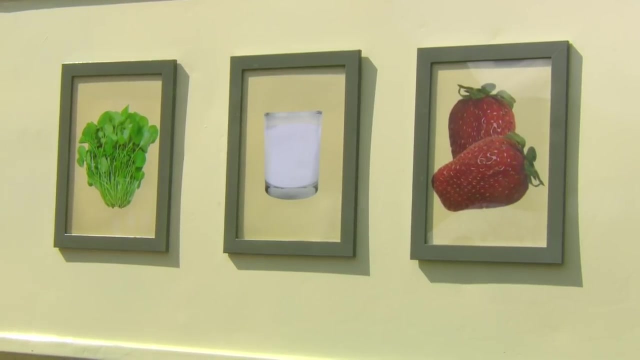 And you take a pinch of pepper and sprinkle it in. And what ingredient do you think we're going to need next in this recipe? What is next? Well, let us see if you can guess what it could be. We have some strawberries, some cow's milk and some watercress. 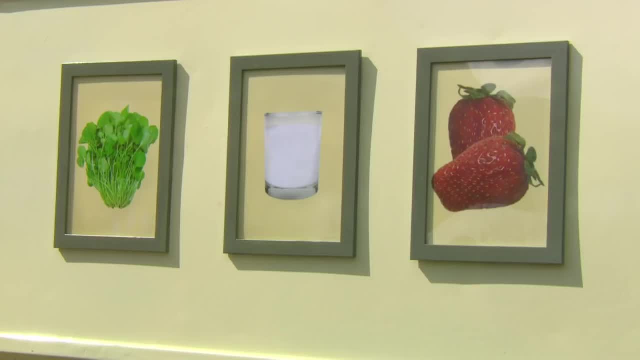 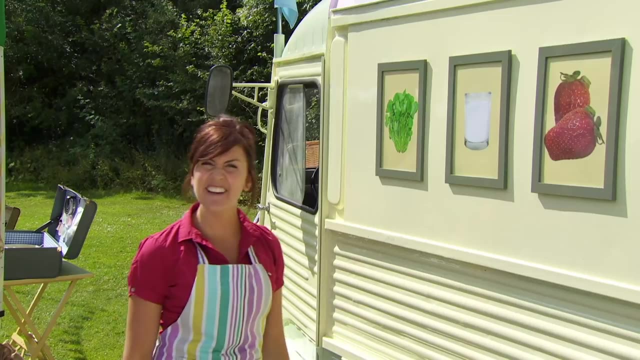 What would you choose for our haddock puff? The first clue is that the special ingredient comes from a plant. Well, it can't be cow's milk, can it? Because that comes from a cow Moo. We'll take that one away. 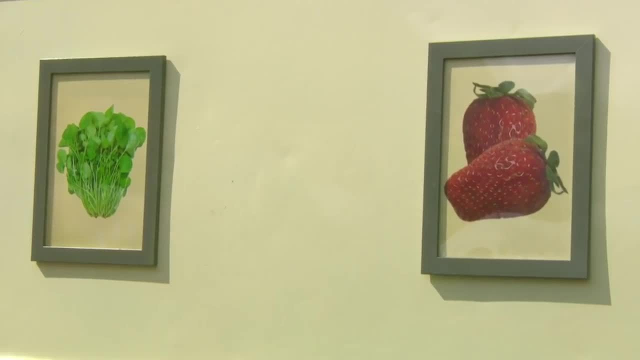 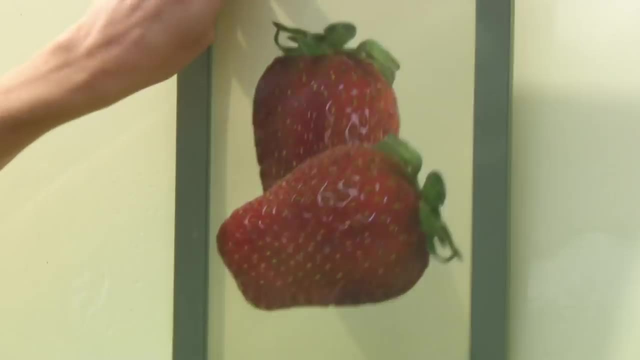 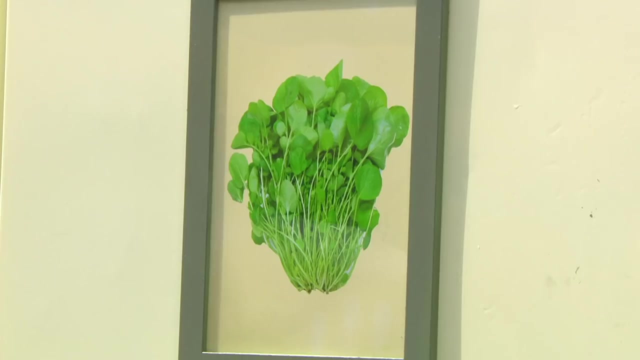 OK, another clue is that the special ingredient is a vegetable. Ah well, strawberries are a fruit, So it can't be that one, Which leaves us with watercress. We're going to need some watercress for our haddock puff, and earlier I went to find some. 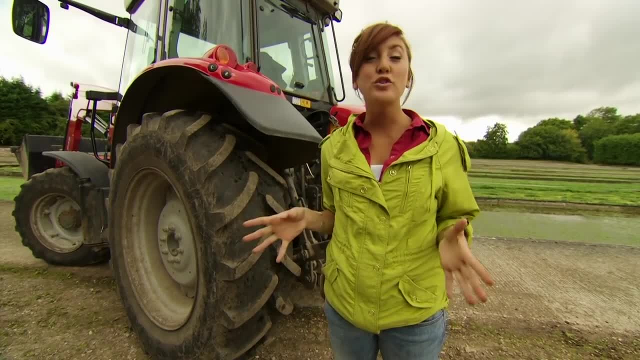 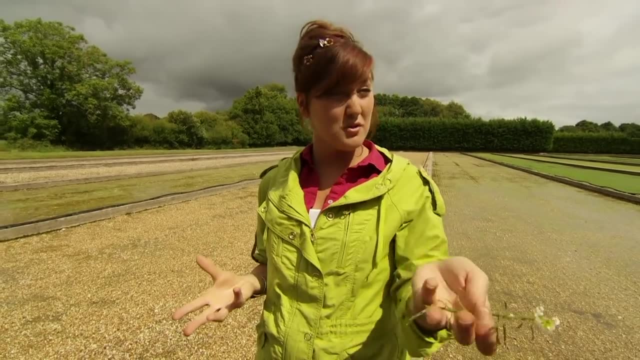 I've come to a farm in Dorset to find out how watercress is grown and collected. Now, watercress doesn't grow from soil like you'd grow things in your garden. It grows in gravel beds which are full of water, like this one here. 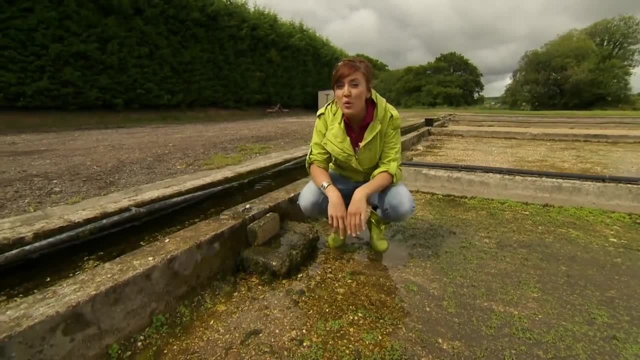 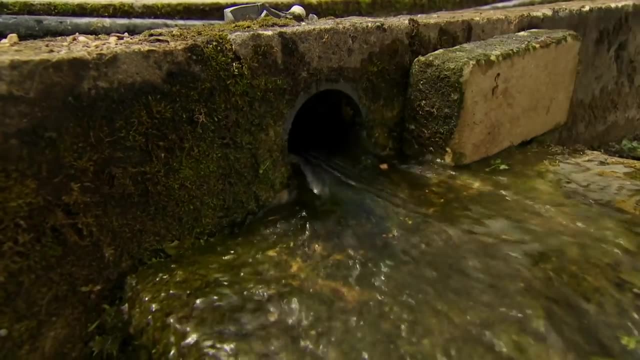 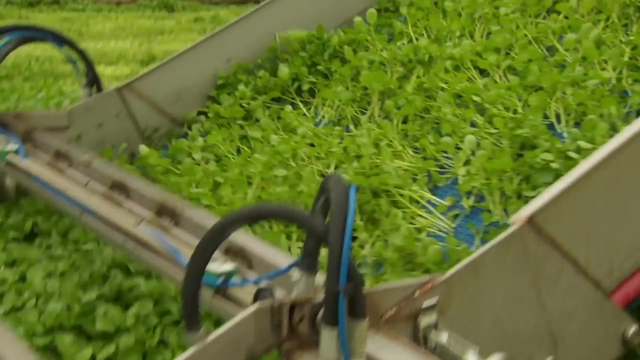 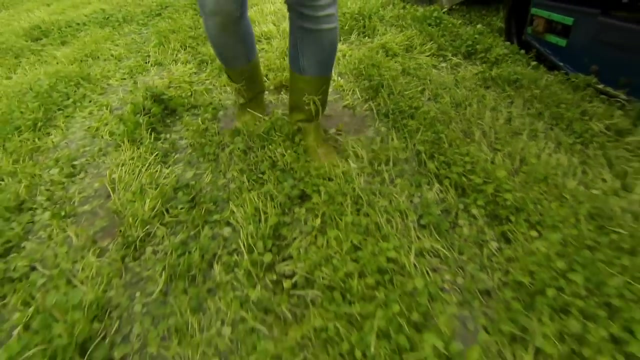 As the seeds grow, more and more water is added to the gravel beds to make the watercress grow bigger and bigger. When the watercress has grown big enough, this huge machine is used to collect it all up. Now this watercress is going to be bagged up. 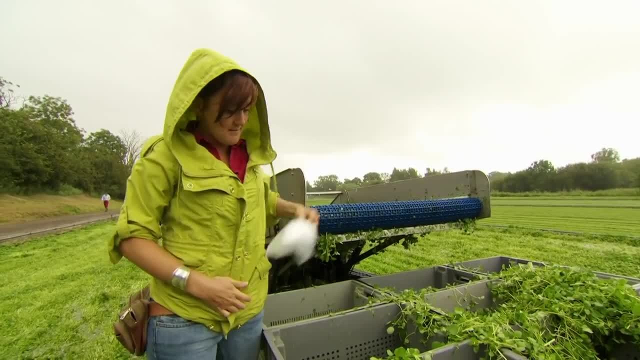 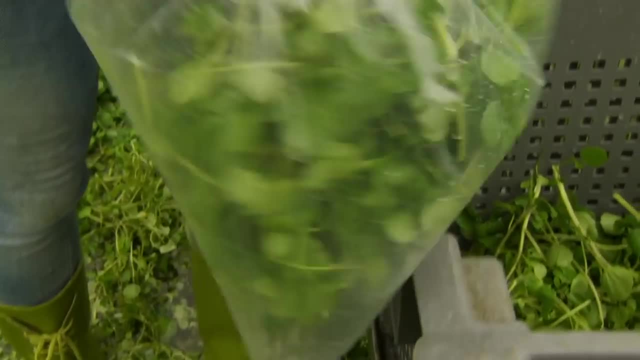 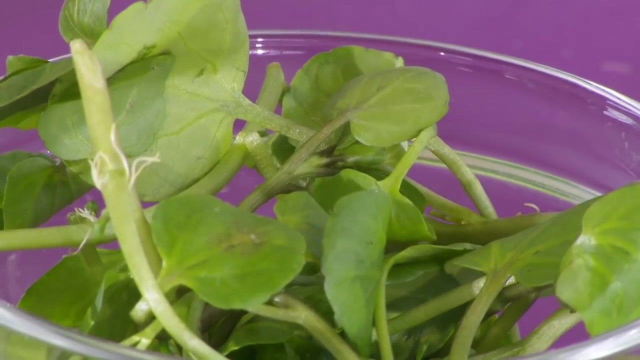 And taken to the shops. I'm going to put some in my bag so that we can use it in our haddock puff. There we go, Fantastic. Let's get back to the kitchen, And now we've got our lovely fresh watercress. we're going to use it in our recipe. 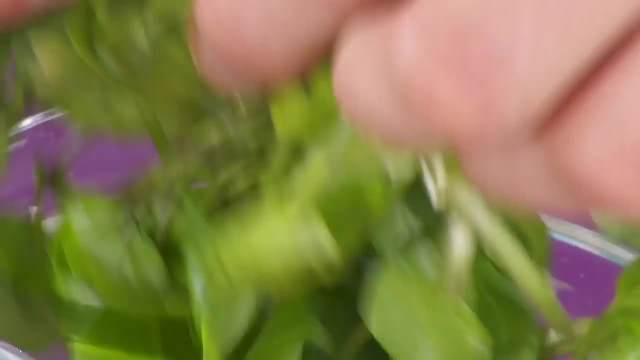 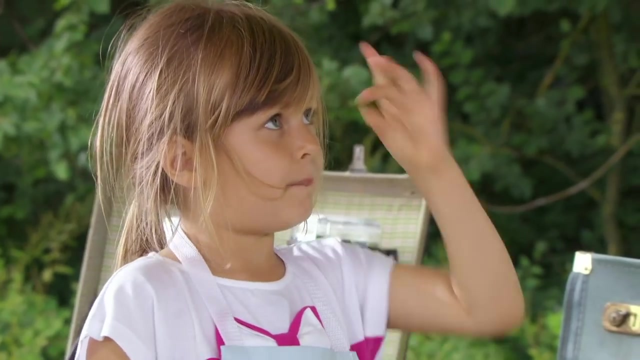 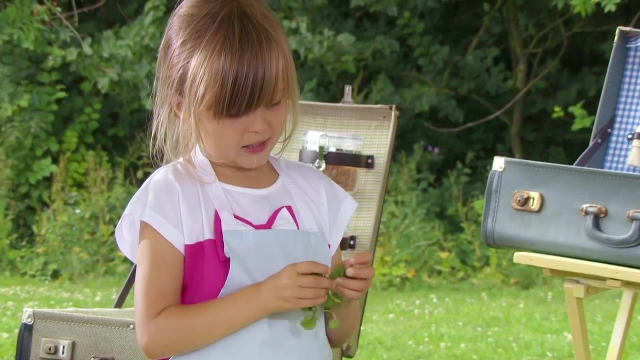 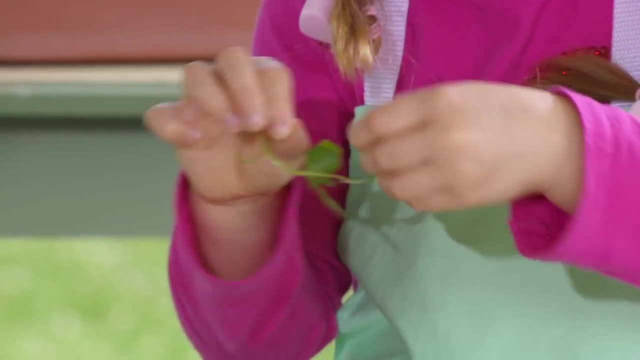 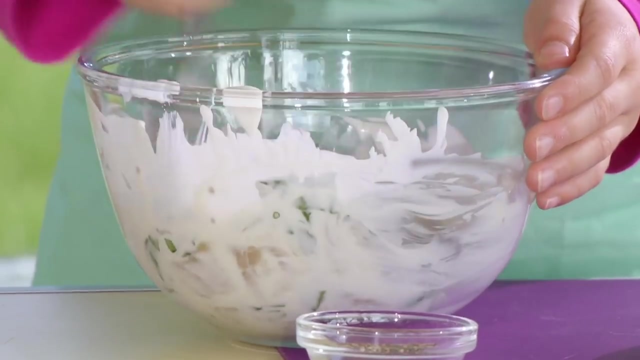 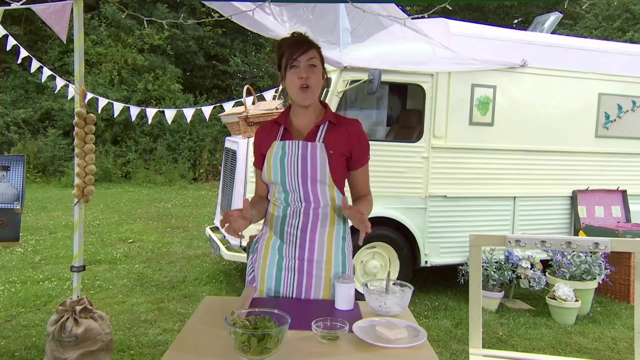 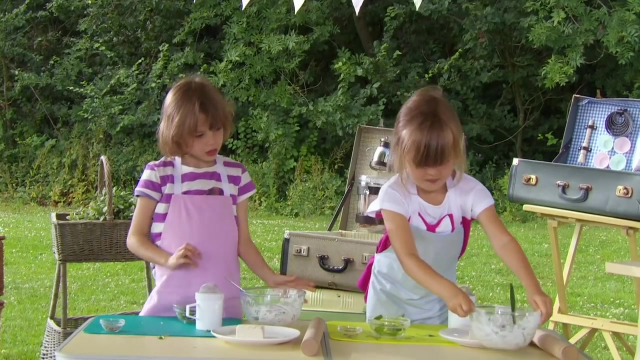 Now, when you've got all of your leaves in the bowl with your fish, we're going to give everything a really good mix. Okay, stop mixing everyone Now. this is the messy part. Who wants to get messy? Okay, now we're going to use some of this. 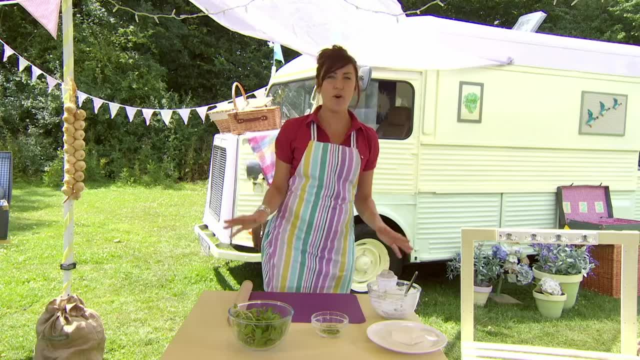 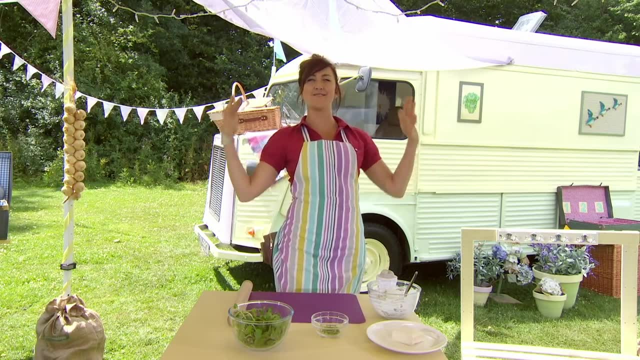 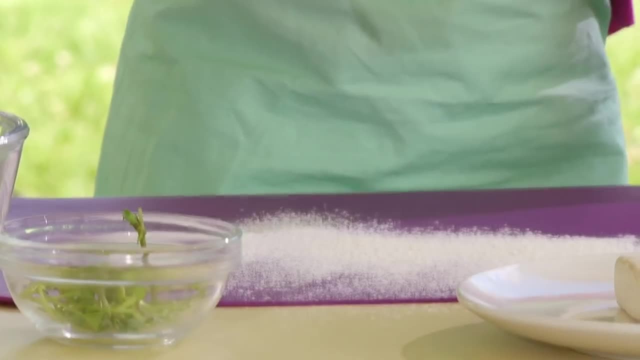 It's puff pastry. Now, before we use the pastry, we need to sprinkle some flour all over our mat. We have to make it snow: Three, two, one go And stop. Fantastic, Okay, put your sprinklers to the side. 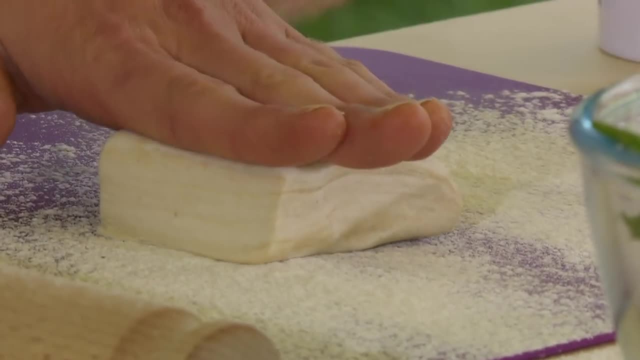 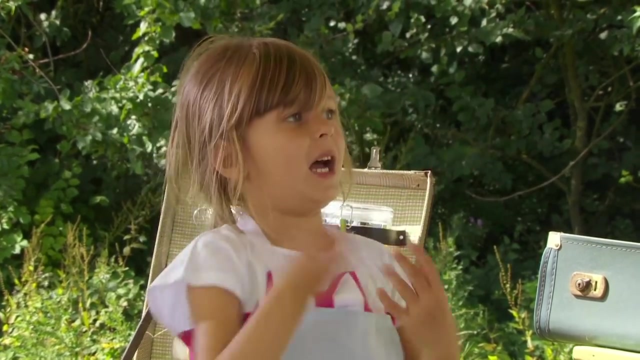 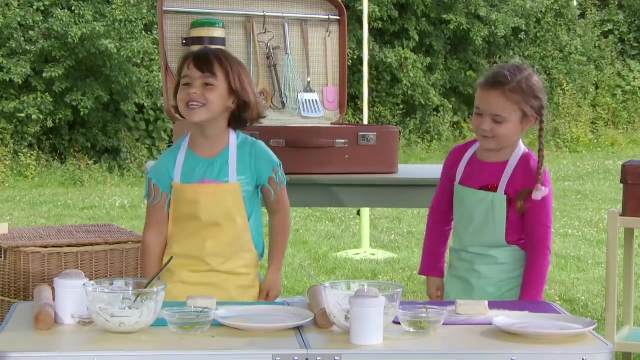 And bring back your puff pastry and put it in the middle of your mat, Because next we're going to do some rolling Ready, roll up, Roll down To the side, To the side, And we roll all around. Are you a bit dizzy? 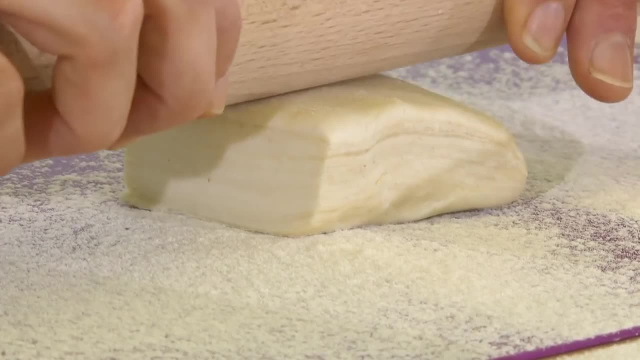 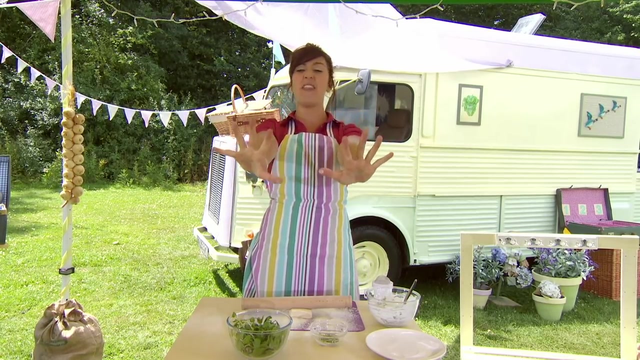 Again. take the rolling pin, put it on top of our puff pastry- And we need to get out our duck feet fingers So you put your hands in front of you and spread them as wide as you can. Okay, keep them really wide and put them on top of your rolling pin. 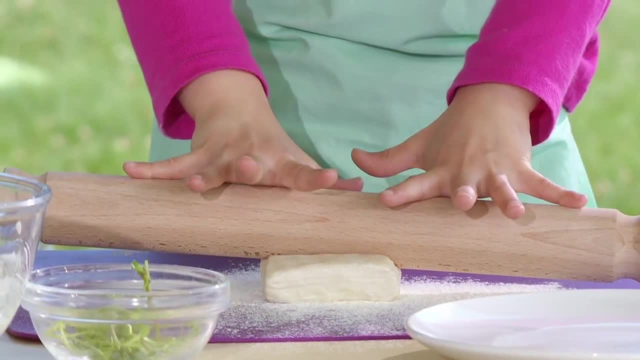 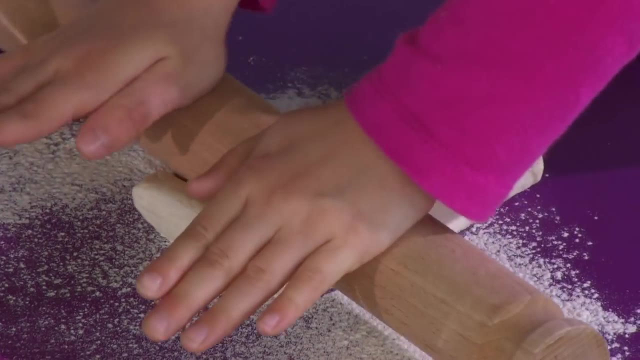 And we're going to use these duck feet, fingers to roll our puff pastry out. That's it. Like this: Yep, Roly, poly, Roly, poly, soly roly. And then put your rolling pin to the side, Pick it up and turn it. 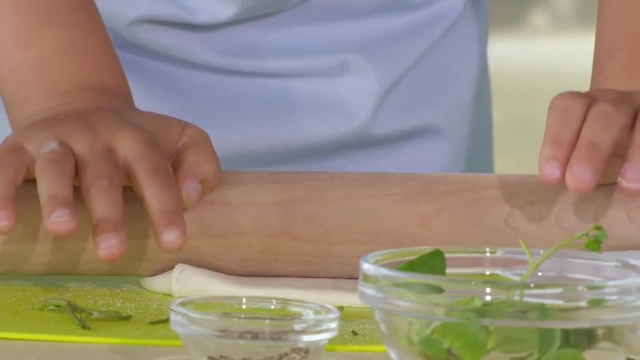 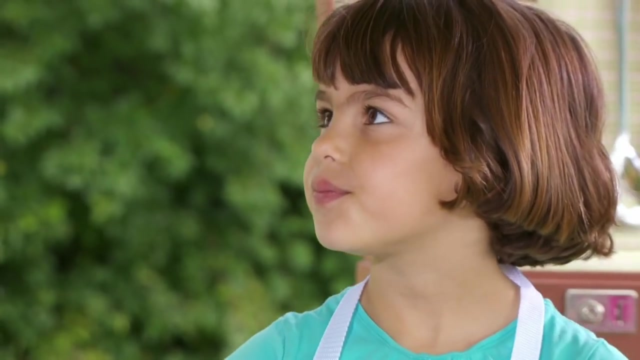 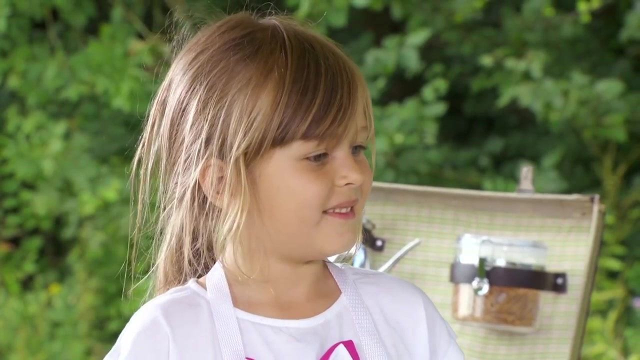 There we go. Ah, Now you need to keep rolling it until it's a rectangle about this size, Perfect. And now we need to add the fish mixture onto the puff pastry. So we scoop it out and we make a big fish mountain. 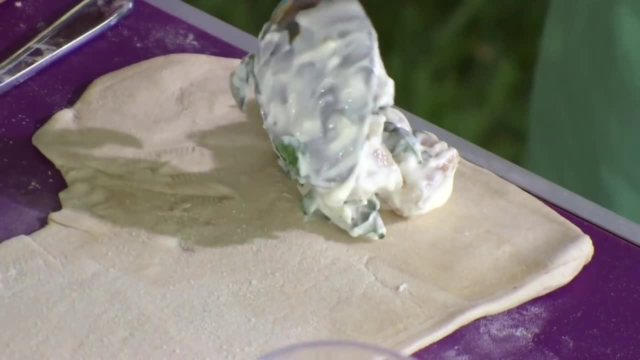 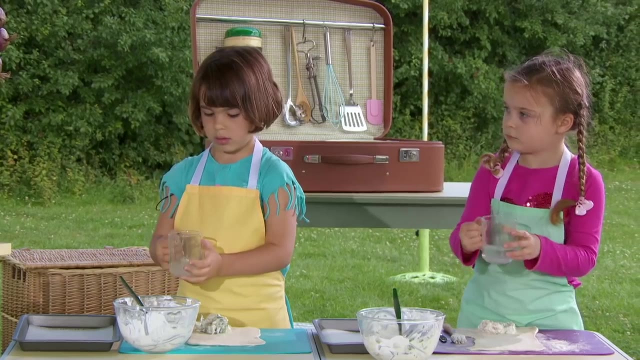 That's it, Leonora. Make sure it's right at the bottom and you leave a little gap underneath. Now we've got a cup here with some water in it And we're going to pour it into our bowl. that had our fish mixture in it. 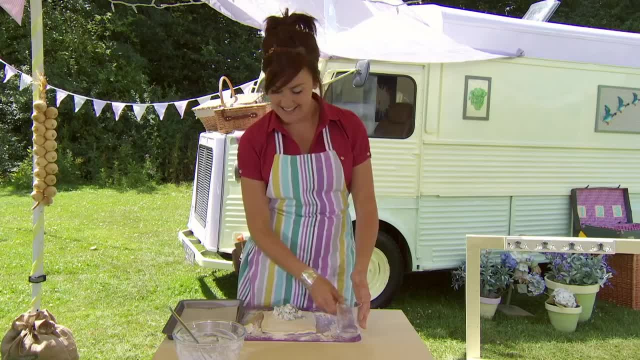 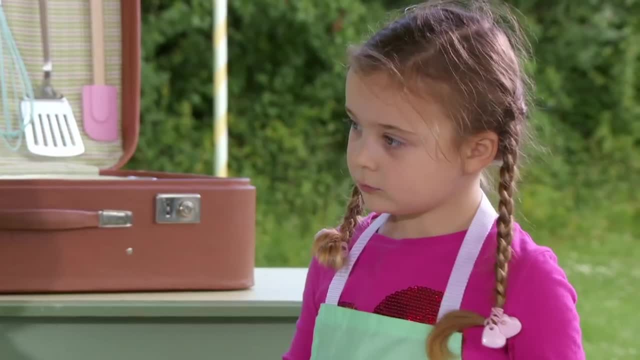 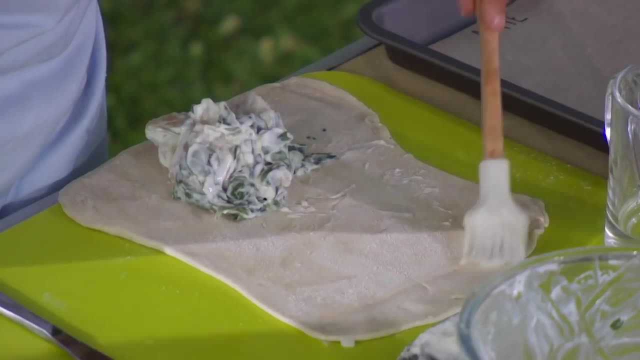 Go And stop. Now take your pastry brush And you're going to mix all of the rest of the fish mixture that's in there. What? all the mixture? And we're going to paint the mixture around the edge of the pastry rectangle a bit like: 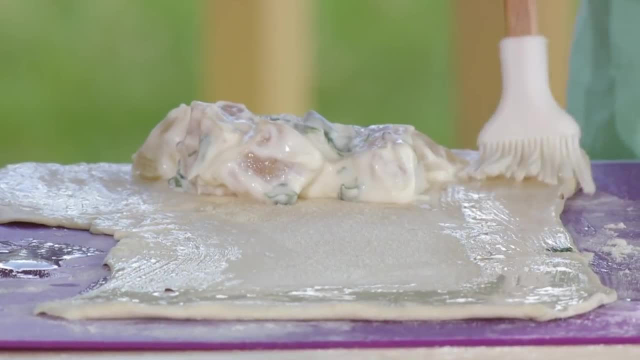 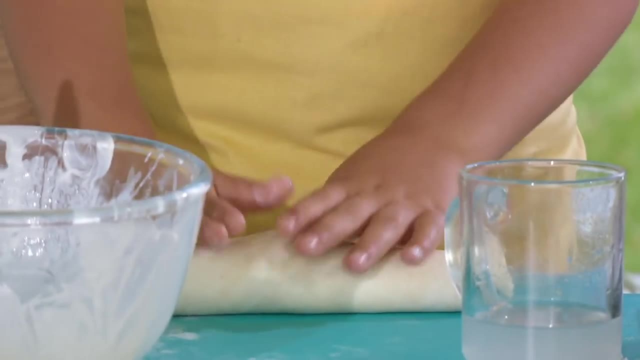 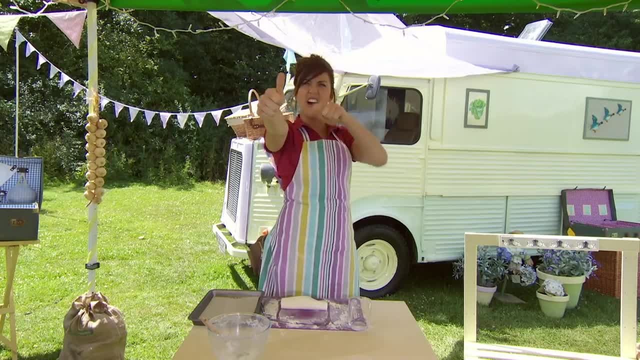 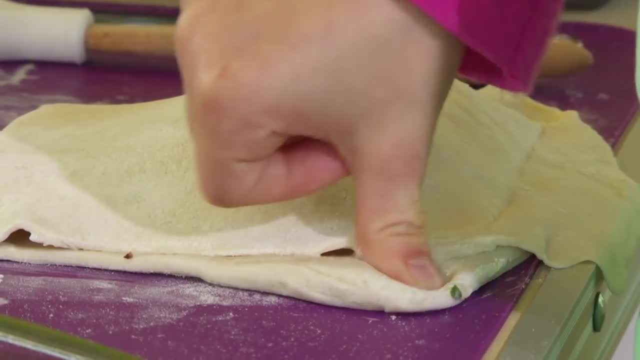 Yeah, Now we're going to use our yeah thumb to walk it around the edge of our pastry. Squish, Squash, Squish. We have to walk all the way around. Squish Squish, Squish Squish. 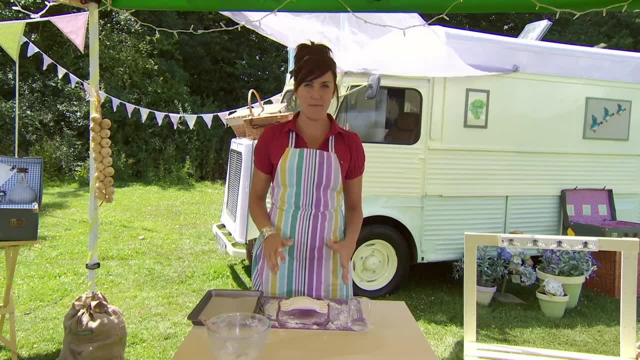 Squish, And now we're going to trim the edges of our pastry, And we're going to use a knife to do this. Now, knives can be very sharp, So you do have to be quite careful, But we're going to use a knife. 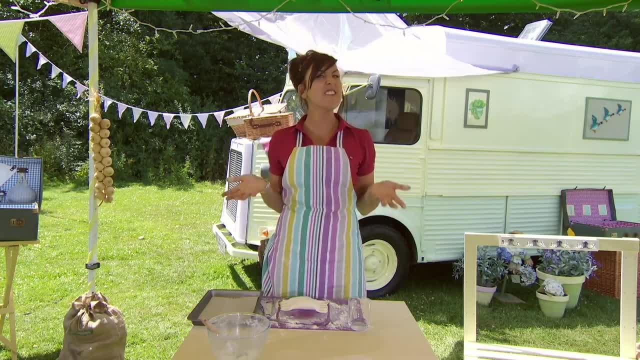 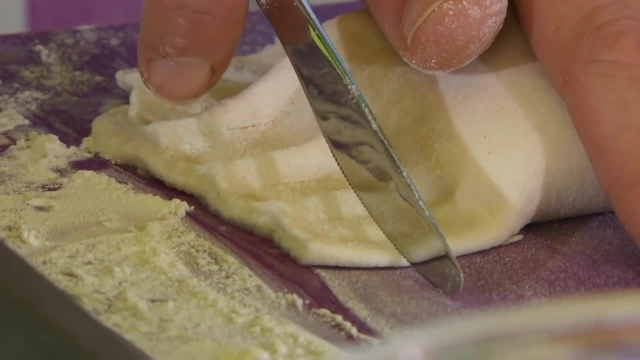 But we're going to use a table knife, Which is the kind of knife that you're used to using at home. I'll show you how to do it. We put our hand on top of the pastry And we cut a line down the side like this: 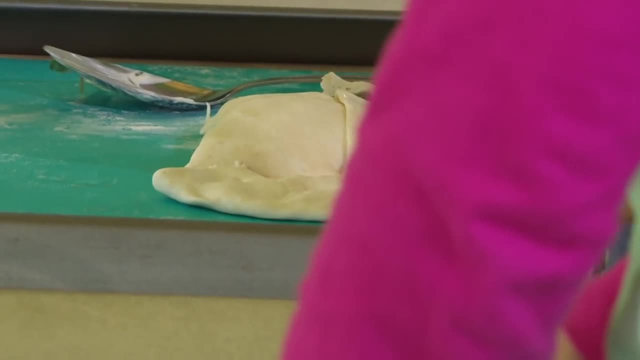 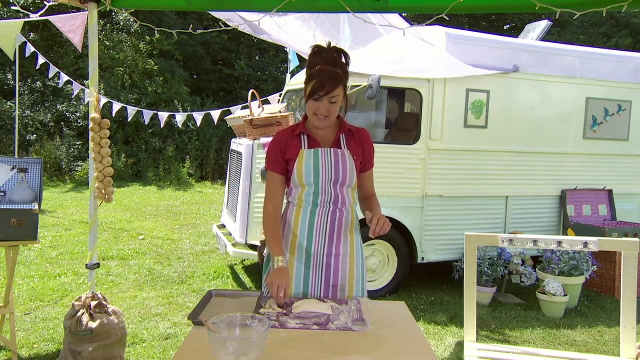 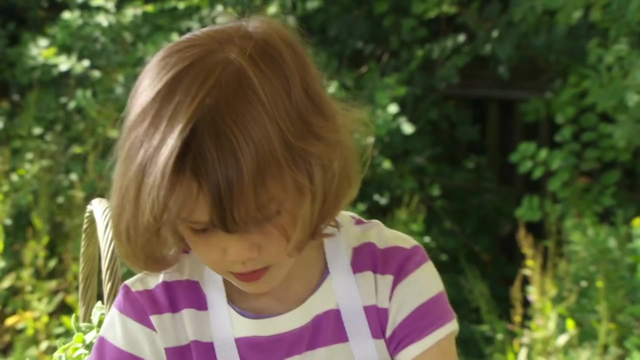 And then you can turn it around very carefully And cut down like that in a straight line, And now we have a couple of finishing touches. We need to make a slit in the top with our knife like this: Now, when the haddock puff cooks in the oven, it's going to get very hot in there. 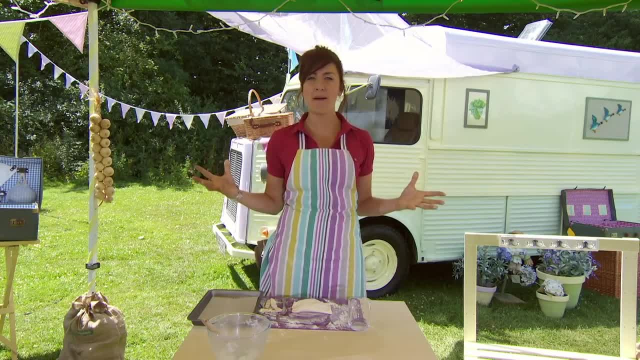 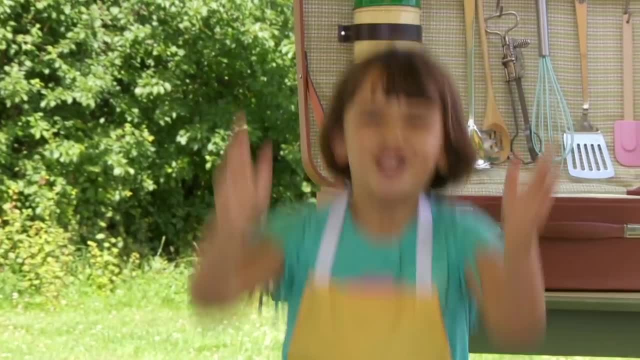 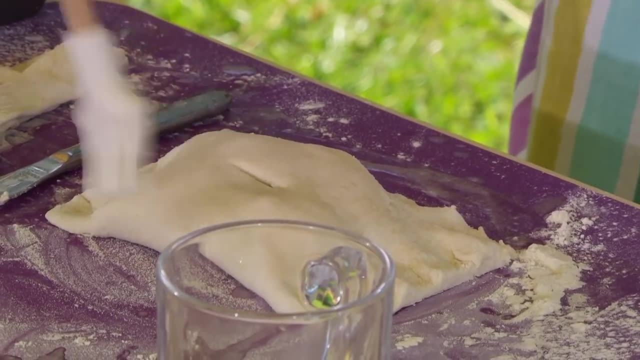 So the slit lets all the steam come out A bit like a train, And the next thing we need to do is a little bit of brushing again. It's going to make it really lovely and shiny, And the last thing we need to do is pick it up very carefully. 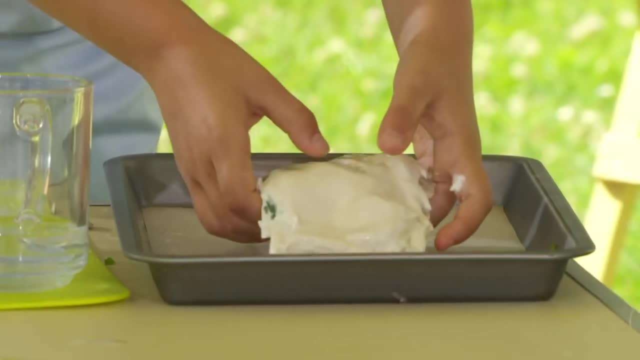 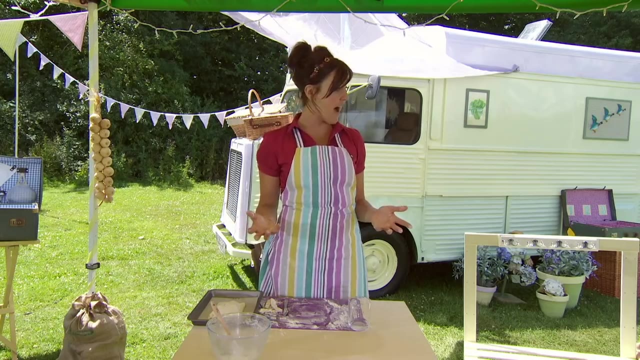 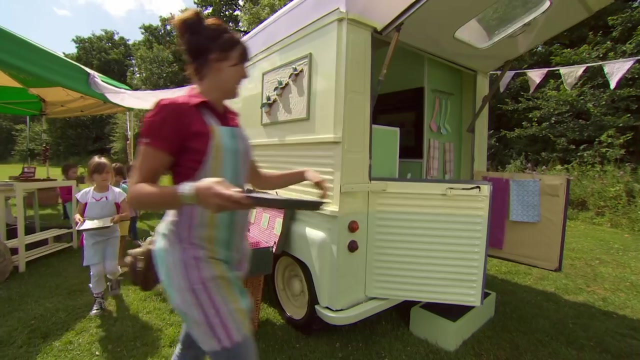 And put it onto your tray, And that is it. You've done it. You've put all the ingredients together for your haddock puff, all by yourself, Yeah, And now let's put them all in the oven. Brilliant, Now remember, ovens are hot. 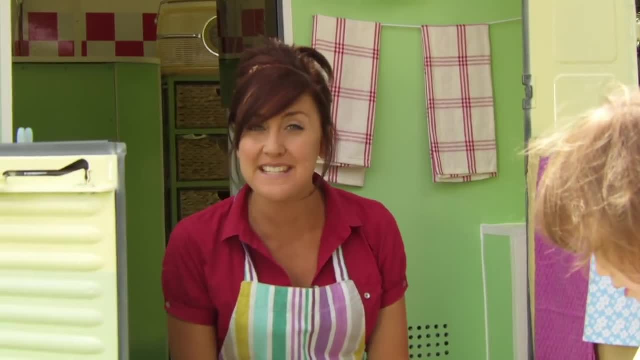 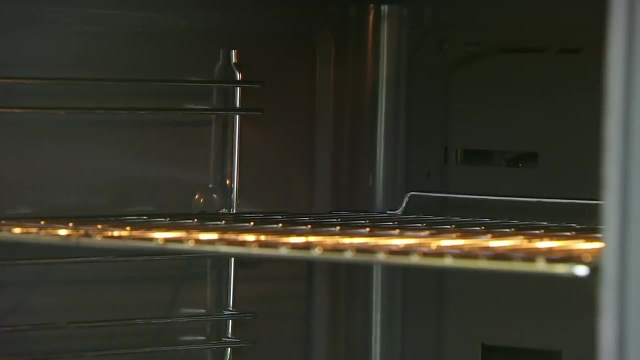 So don't go near. You need to ask a grown-up to help you here. So you're going to help, So I'm going to help. So why don't you pass me them one by one Now? we've cooked with you and had lots of fun. 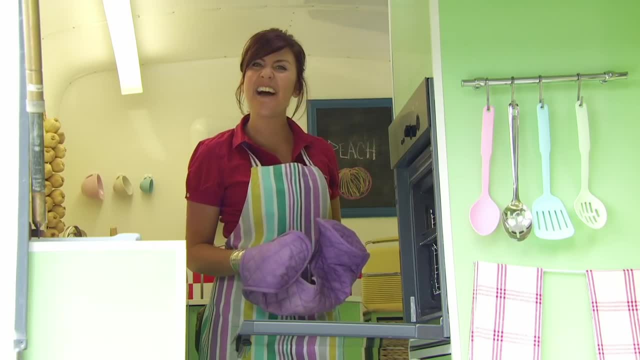 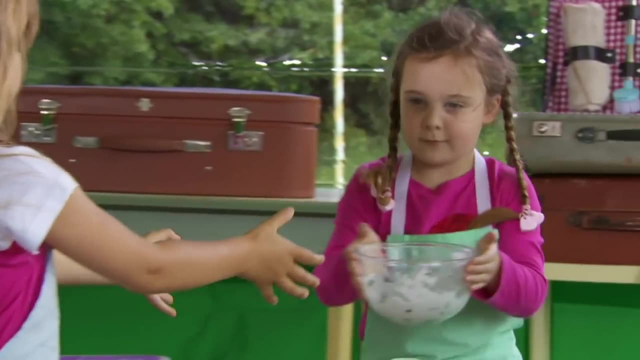 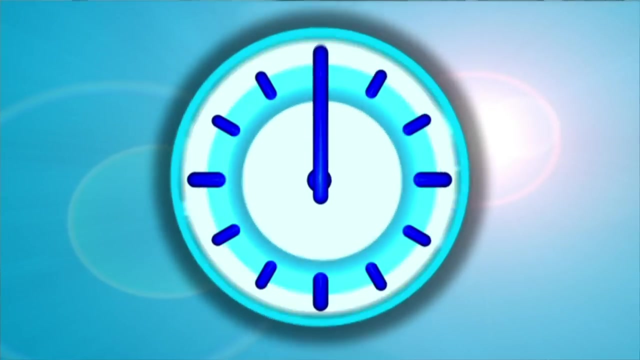 Let's tidy up and think of all the things that we have done. There was Flipping, Mixing, Rolling, Brushing. Now clearing any mess and putting things away is always fun to do at the end of the day. And here they are all ready to eat. 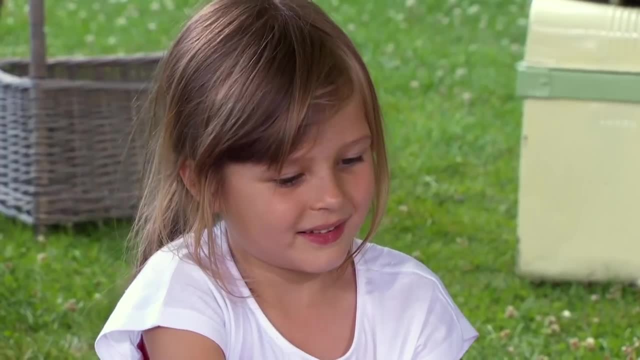 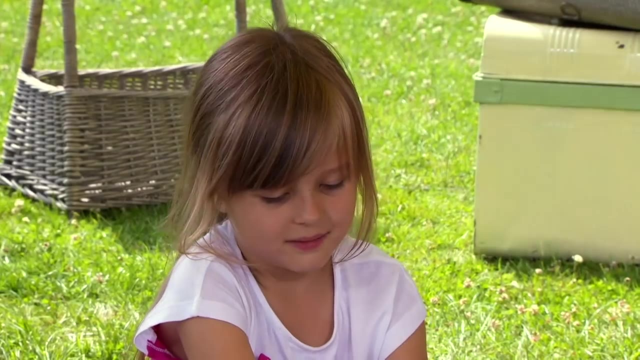 You've made your very own haddock puff. Let's have a look at yours, Leonora. Wow, that looks fantastic. Ami, let's have a look at your one. That looks yummy, That is delicious. And look, I can see the fish inside. 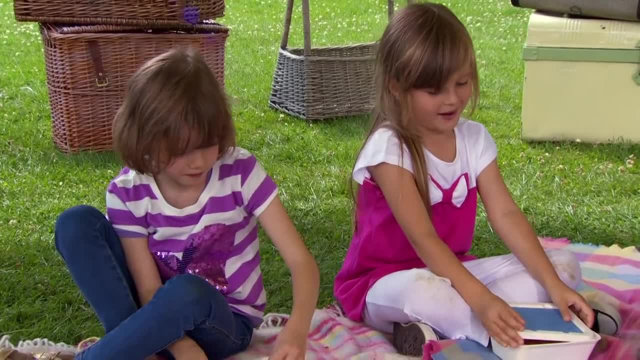 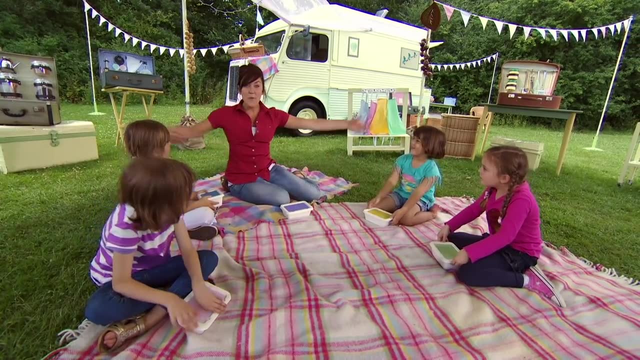 Right, let's put the lids on top. We'll save that for later on. We've travelled to you, We've cooked and had fun. Now let's have a party with everyone. Yeah, Come on, you can come too. 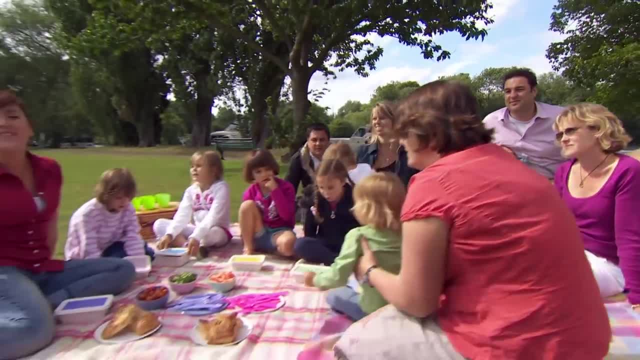 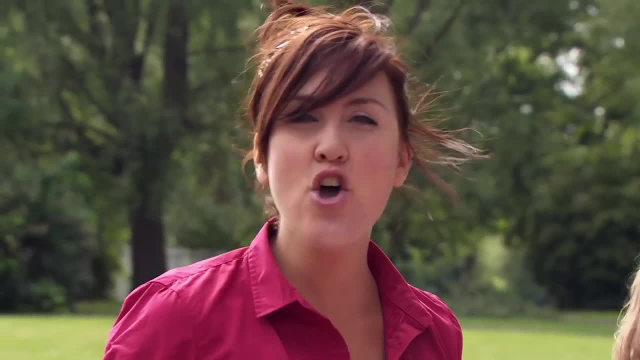 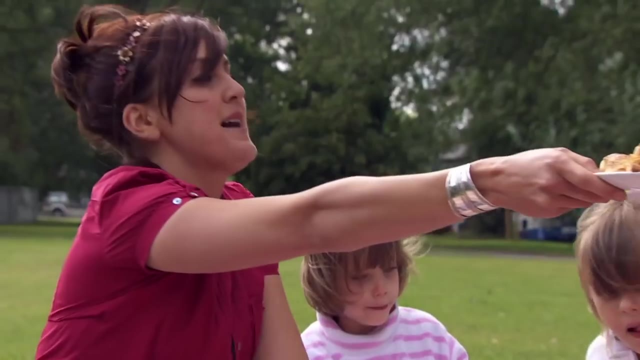 Well, here we are, back down by the river, and we're all ready to have a lovely picnic before we go and take the dogs for a walk. Now, who is hungry? Me, Brilliant. Well, we've got lots of haddock puff to share with everyone, so who'd like some haddock? 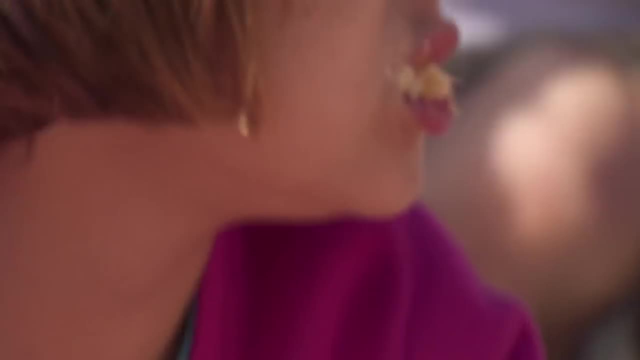 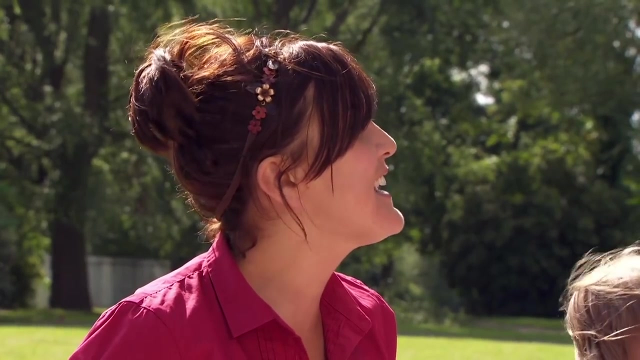 puff. That's mine. Oh, that is absolutely delicious, isn't it everyone? So Amelie's mum and dad, what do you think of Ami's cooking? Good, Beautiful, It's lovely Summer. what's happened to the pastry? 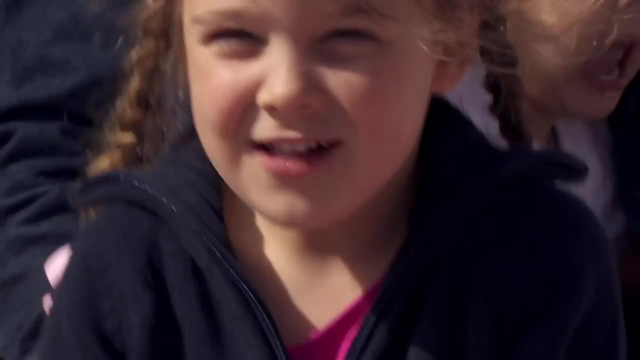 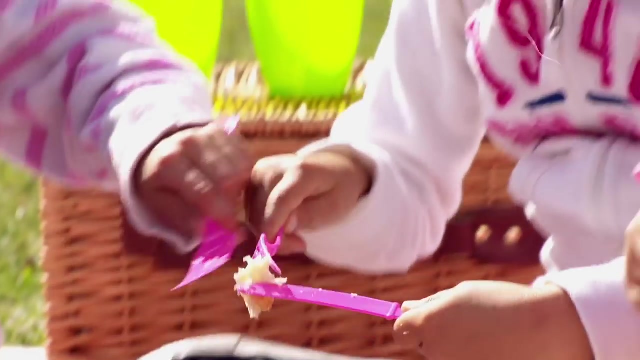 It's just gone hard. So, Otti, what's been the best part of your day? Um, me too. Me too, Mine's the yummiest. No, mine is, They're both the same yummy. So, everybody, what can you do? 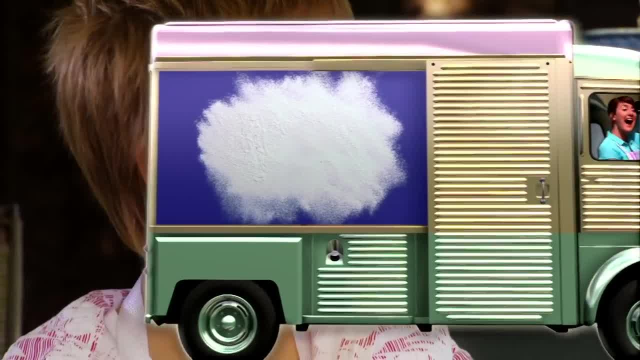 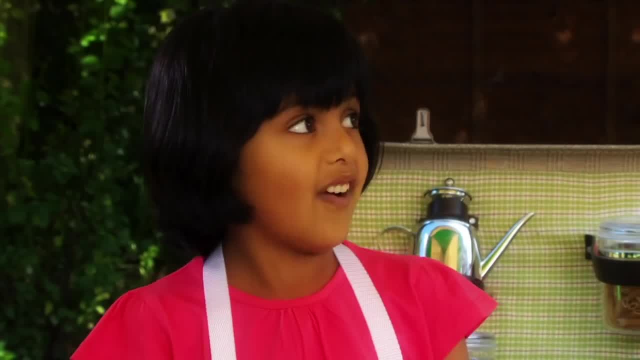 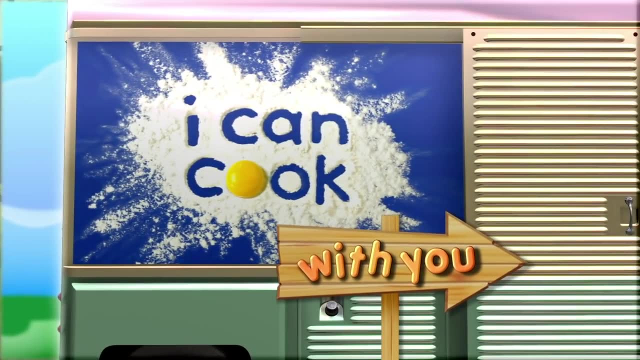 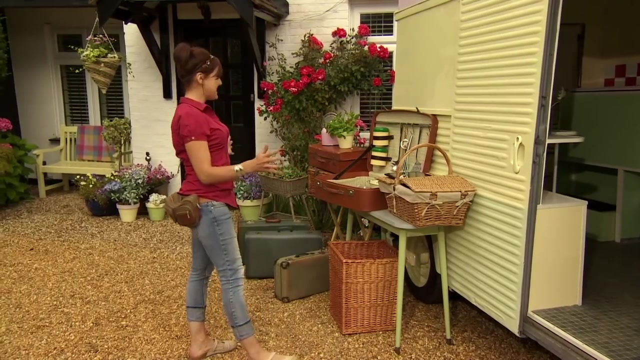 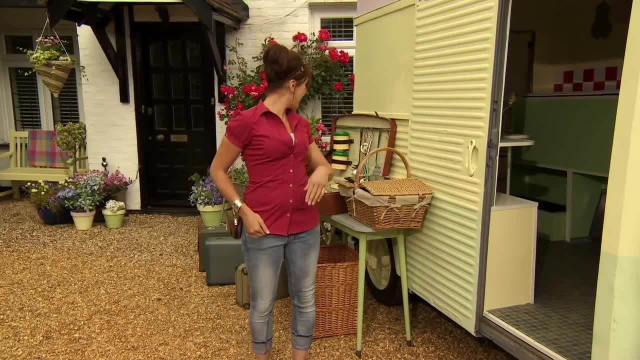 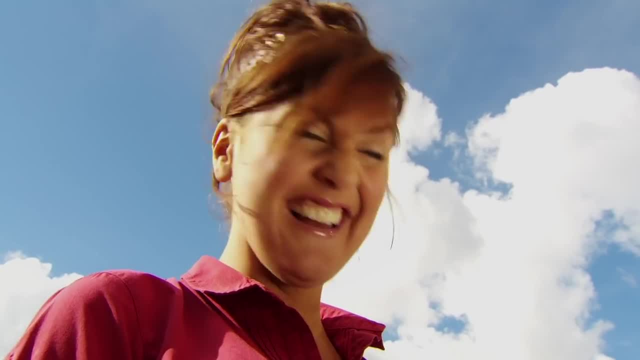 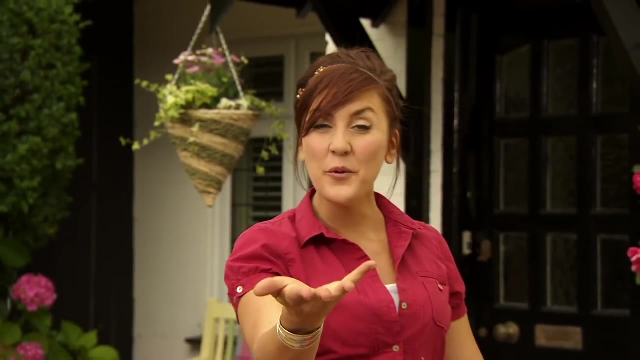 to come with me and meet some new friends. A-ha, Hello, Katie. I really like art and I love fruit. Katie, what's your favourite evening? My favourite evening, Katie, can you cook with me please? I can, Hector, and you can cook with me too. 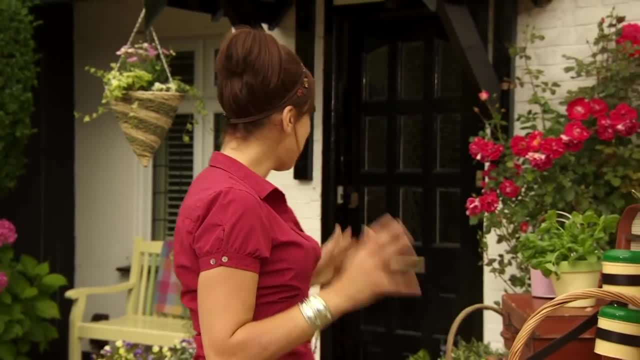 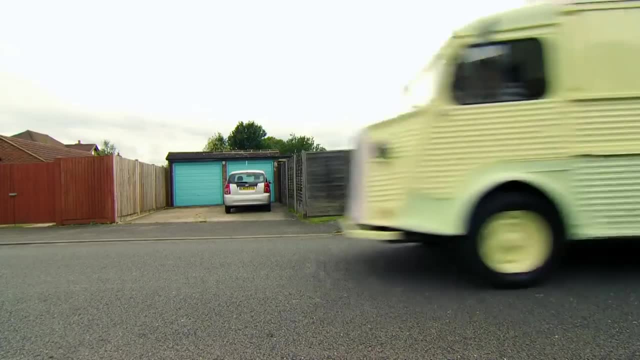 Hector's invite does sound really exciting, doesn't it? Right? let's get everything packed up as quick as we can, and then we'll get on the road, Off on a journey, and I'm coming to you. it's going to be busy and there's lots to do. 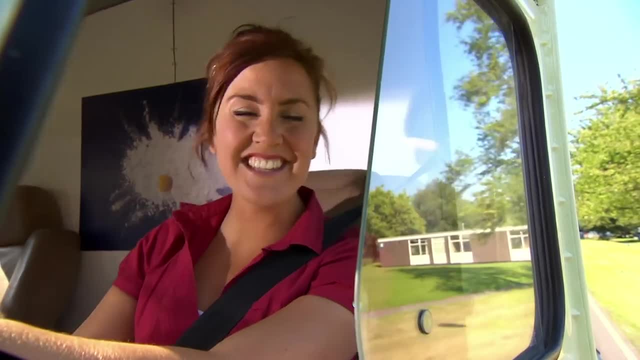 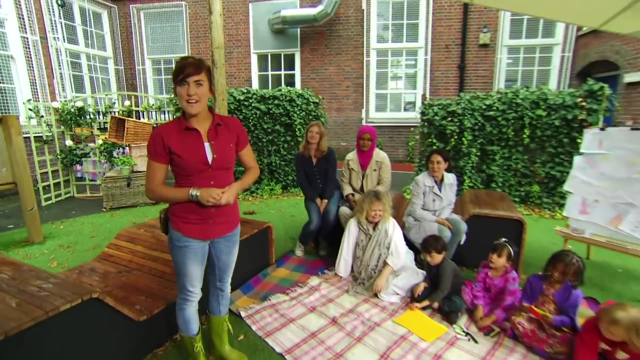 Get ready to help, join in and have fun. let's cook a feast for everyone. I can't wait to do some art. I really love drawing. Oh, it's Hector and all his friends. hi, Hector, Hello, Katie, What's your name? 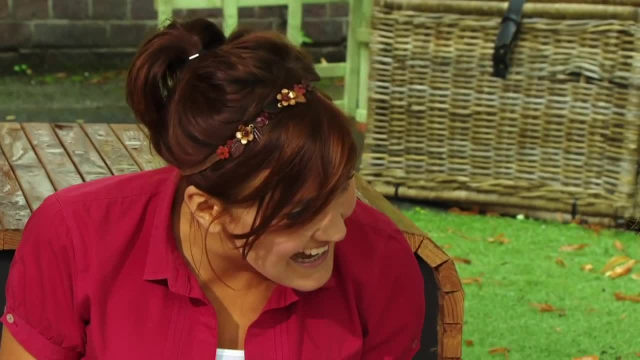 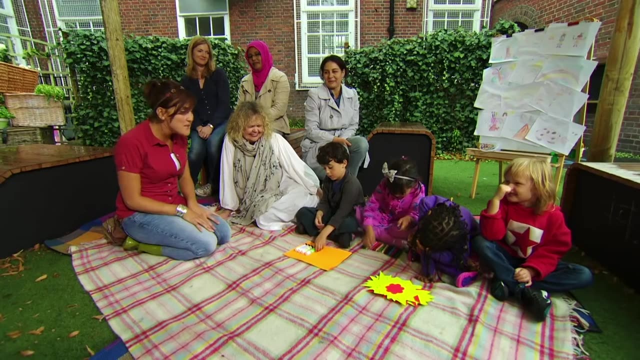 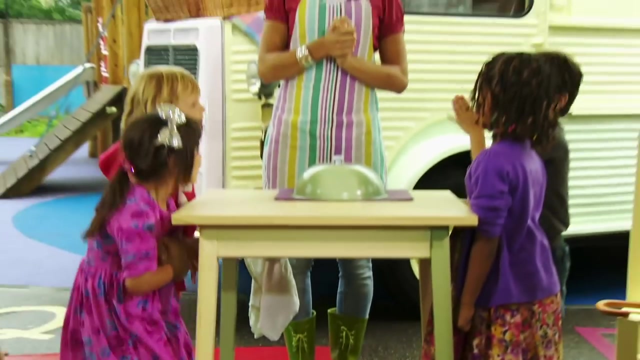 Asha, Nina, Jonah. So what are we going to do today? Hector, Make something with fruit. I have got an absolutely delicious fruity recipe. do you want to make it with me everyone? Yeah, Come on then, follow me. Welcome to my outdoor kitchen. 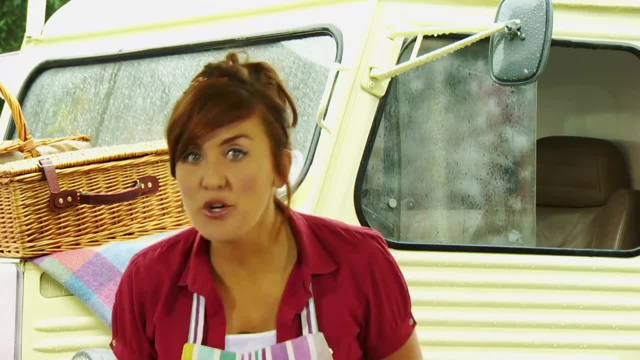 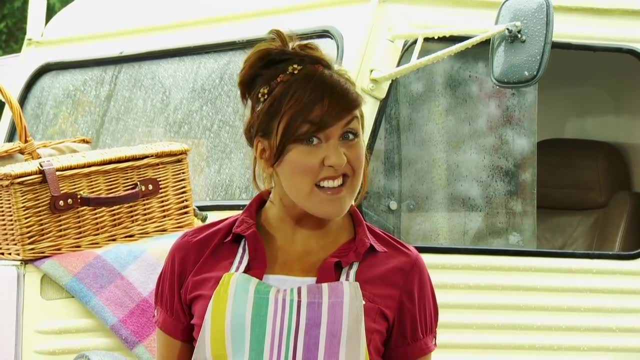 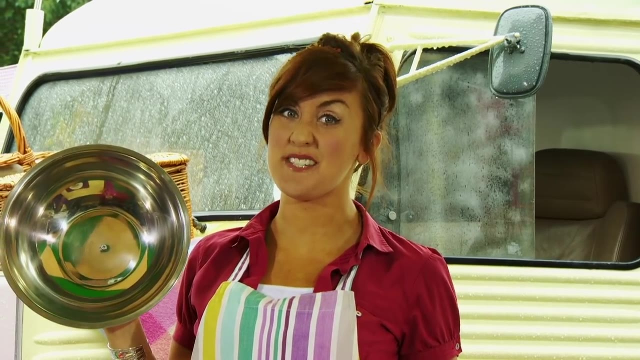 Do you want to know what recipe we're going to cook? Well, today we are going to cook fruity phyllo parcels. look at this Now. I can't wait to eat those. but before we cook them, we need to do something first. 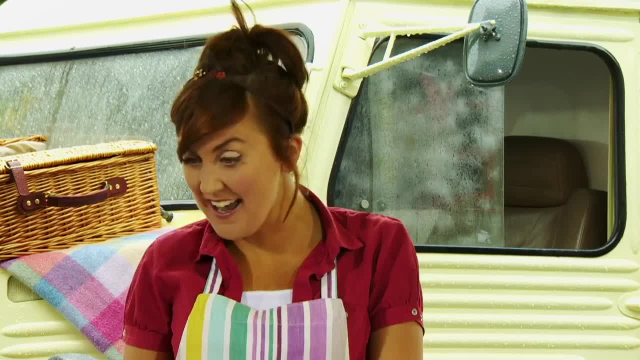 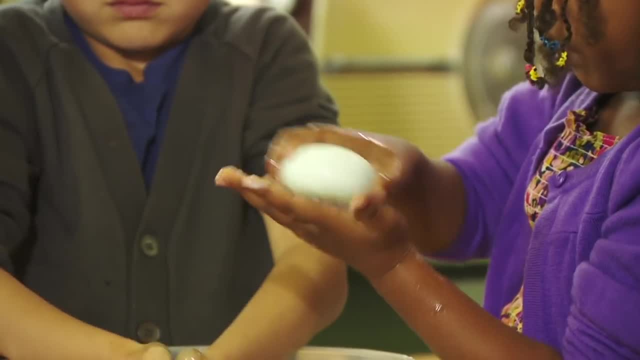 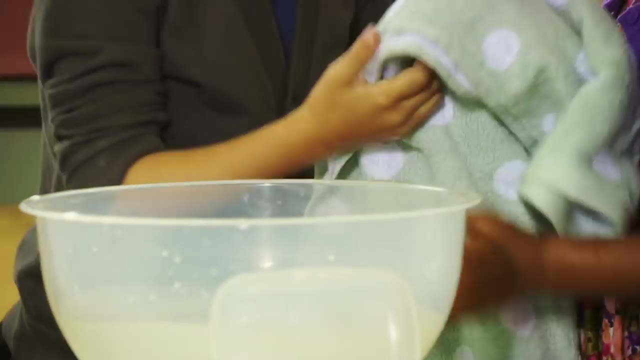 what do you think it is? Wash our hands, Wash our hands, that's it. come on, team, let's get going. Roll up your sleeves, give your hands a wash with slippy dippy soap, splish, splash, blosh. have you done your hands washed and dried? sleeves rolled up, apron tied, what can you? 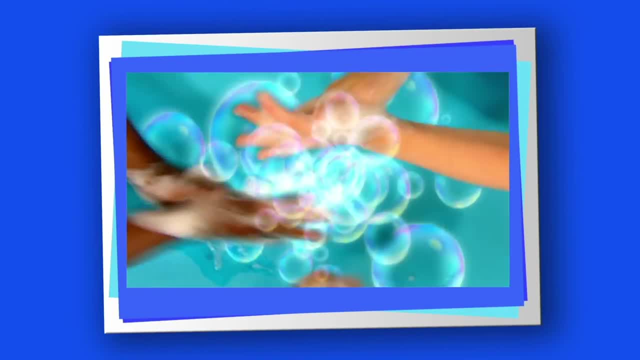 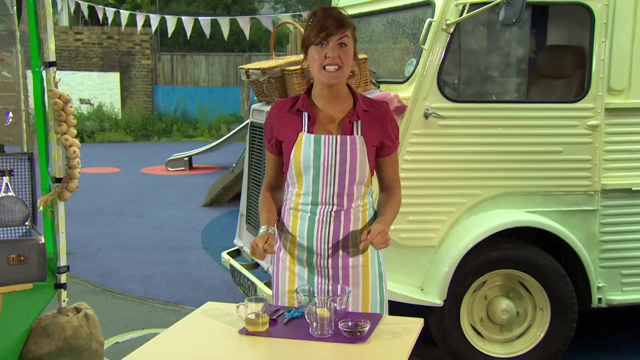 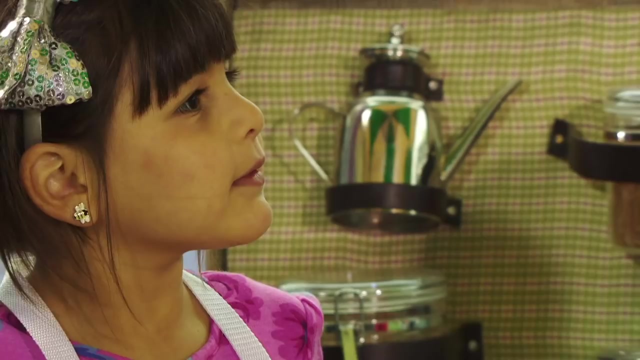 do, I can cook Right. then let's get started on these fruity phyllo parcels. first thing we need is Mr Teaspoon, and look, he's right here. Hello, Hello, Mr Teaspoon, Oh, hello, Katie, are we going to do some measuring today? 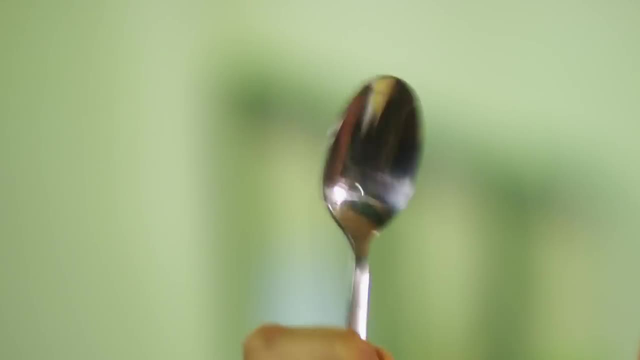 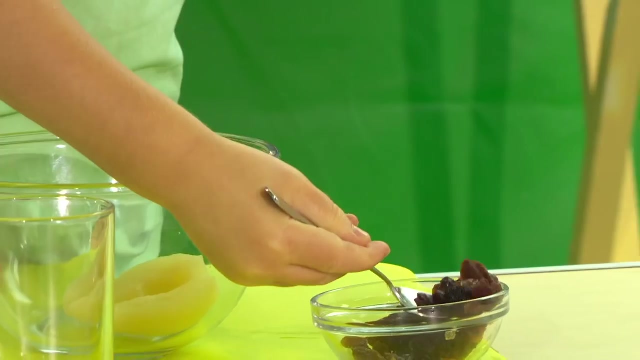 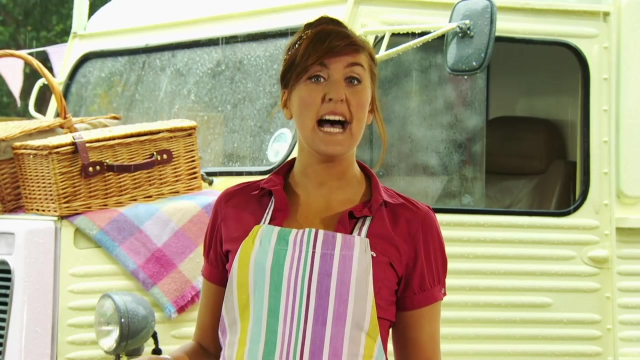 Indeed, we are Mr Teaspoon and we need your help. How many teaspoonfuls do we need? We need two teaspoonfuls of this mixed fruit down here, one, two. The next thing we need is Mr Tablespoon, who's down here. 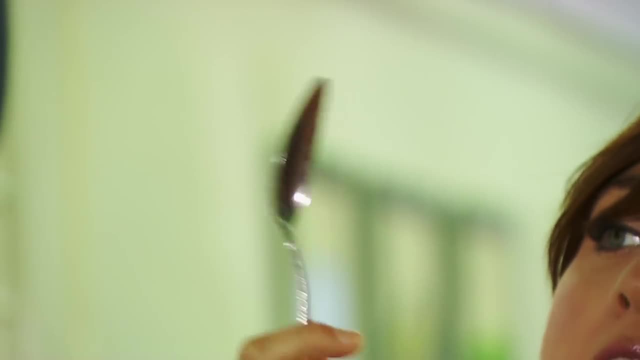 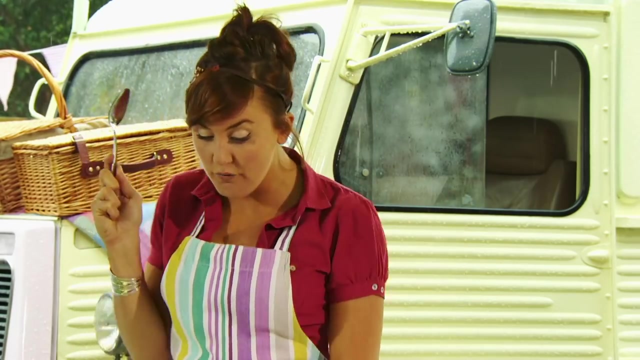 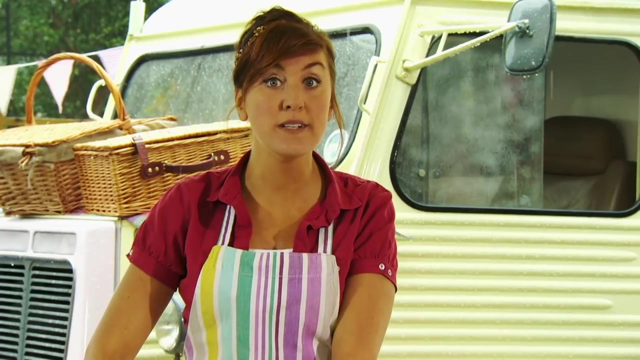 Hello Mr Tablespoon, Oh, hello Katie. Are we going to do some measuring? Yes, we are, Mr Tablespoon. we need one tablespoonful of this juice. So we put our spoon into the cup and we tip and load to fill it up. so hold the cup by. 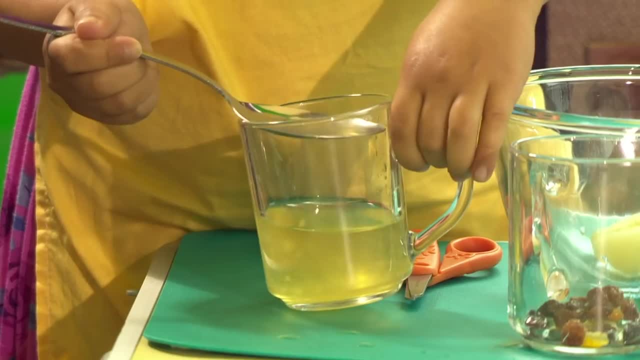 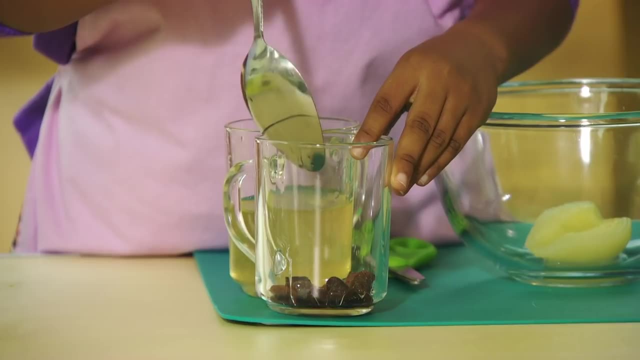 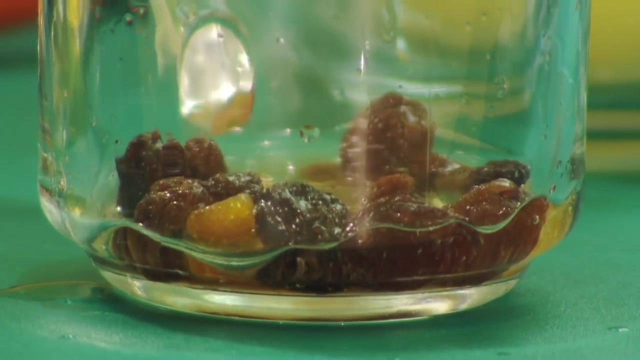 the handle everybody and gently tip it to the side and fill your spoon up with juice and then splash it in with your fruit, And what's going to happen is the fruit is going to soak up the juice. The next ingredient we need is a pear, but where's the pear? 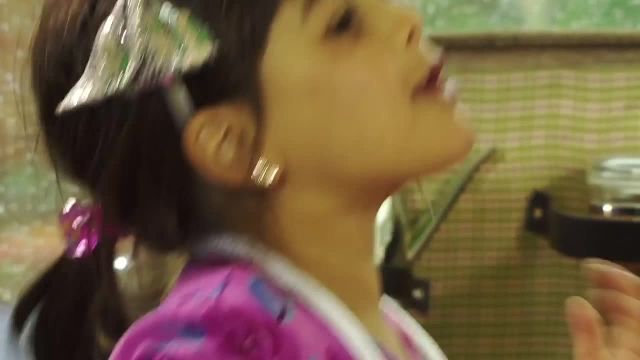 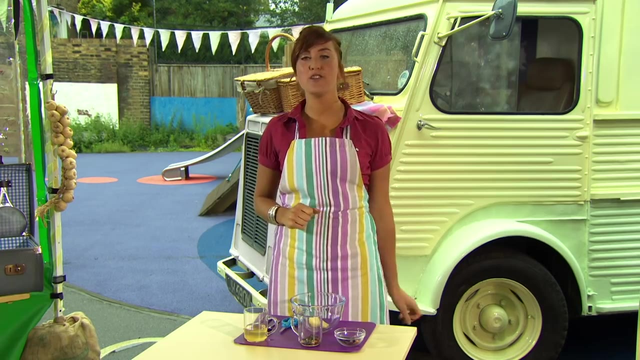 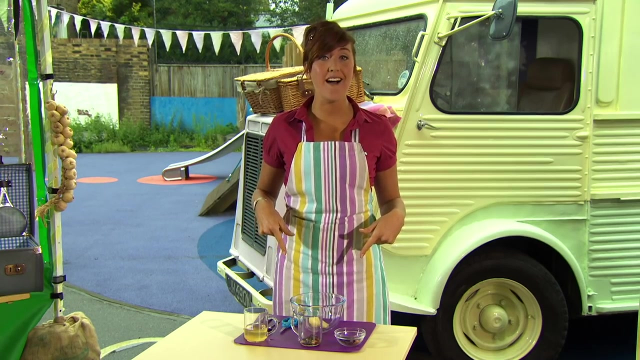 Pear's on the side of our face. Is it over there? No, It's on the pear Pear. Oh, there's the pear. and we are going to snip this pear up using a pair of scissors. but remember, be safe with scissors. everyone knows that we point them down towards our 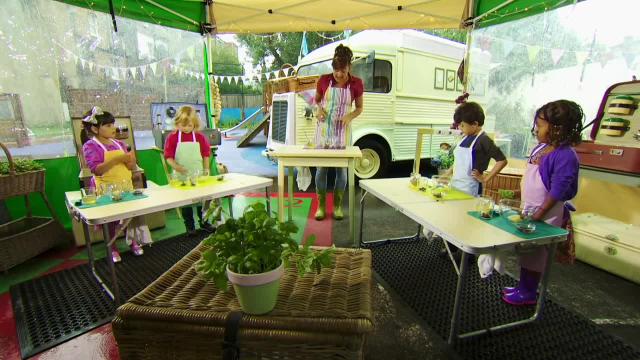 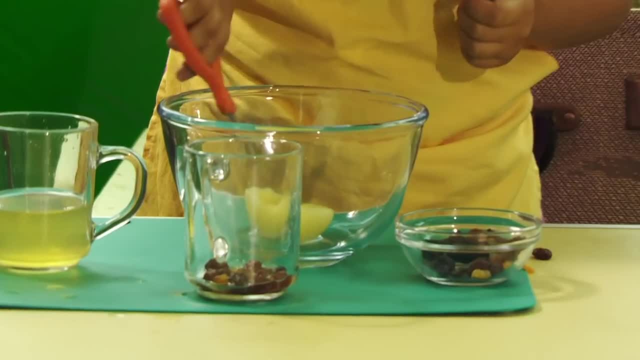 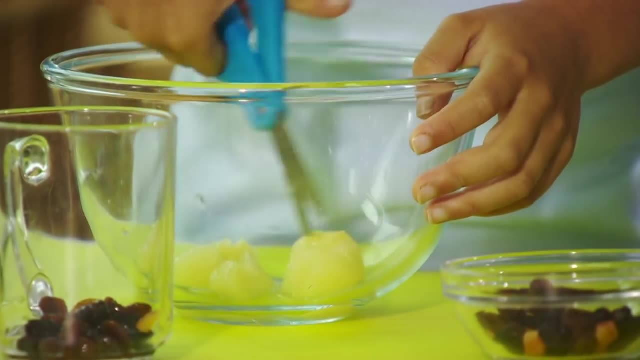 Toes, Toes towards our toes. so take your scissors and let's get snipping. Oh, it's a very soft pear, isn't it, Aisha? Yeah, It's slipping away from me. I snip the pear. I snip the pear. 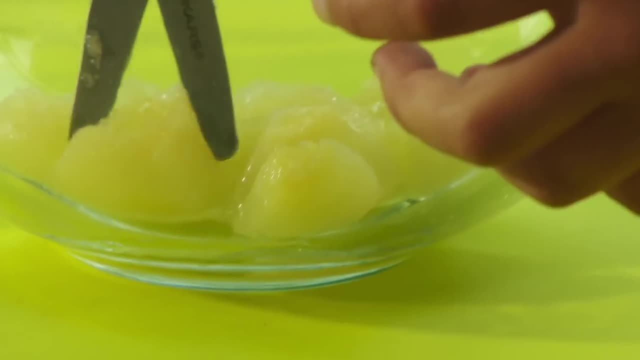 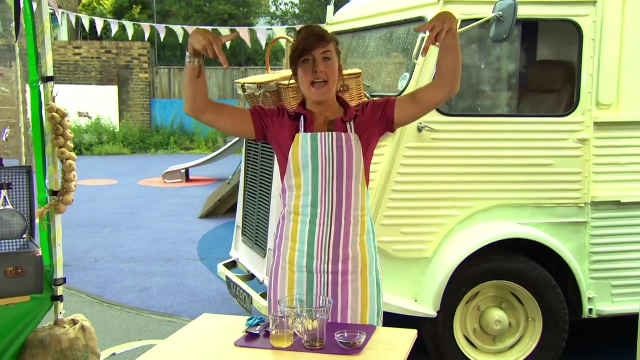 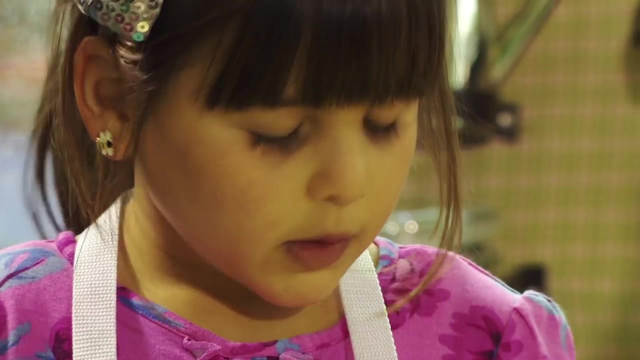 Snip, snip, snip, And you can do some snipping with us at home too. All you need are your scissors, like this, and then you can go snip, snip, snip. The next thing we have to do is add our mixed fruit that's soaked up, the juice in with. 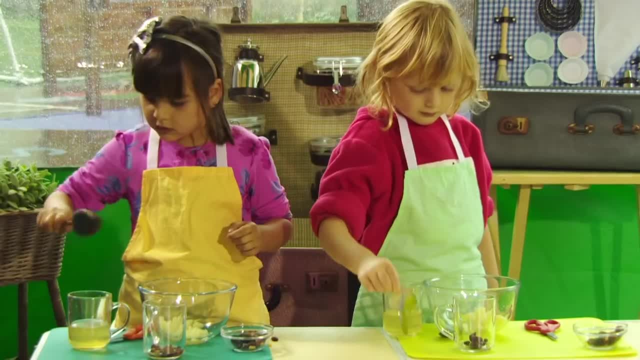 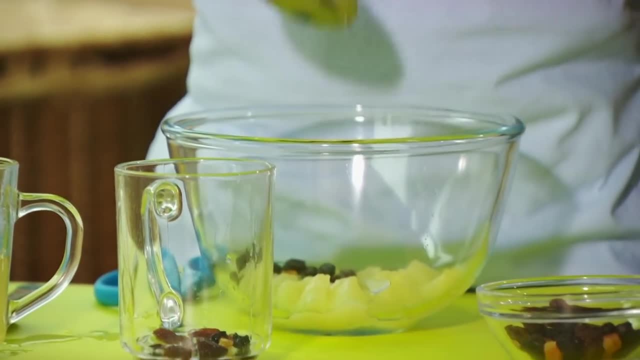 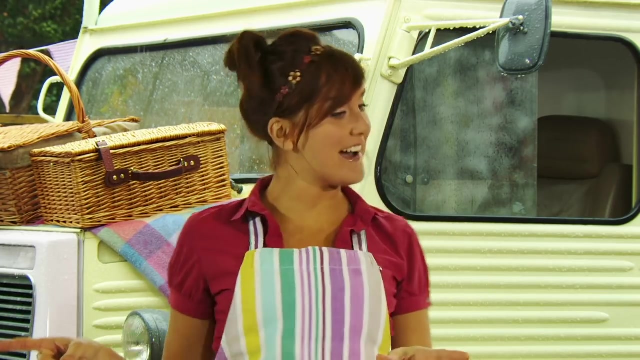 our pear. So let's take our big spoon and then scoop up the mixed fruit and put it into the big bowl. This dish is very fruity, isn't it? Who can do the fruity dance? Me, And you can join in with us. 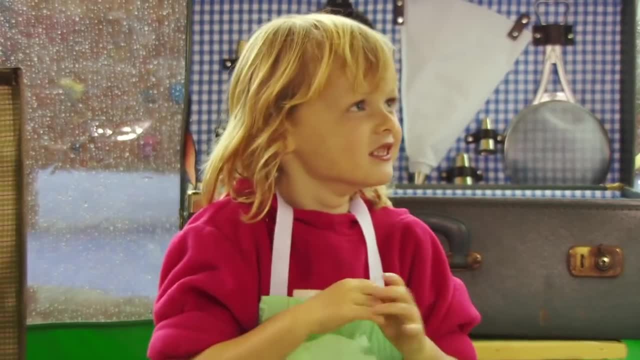 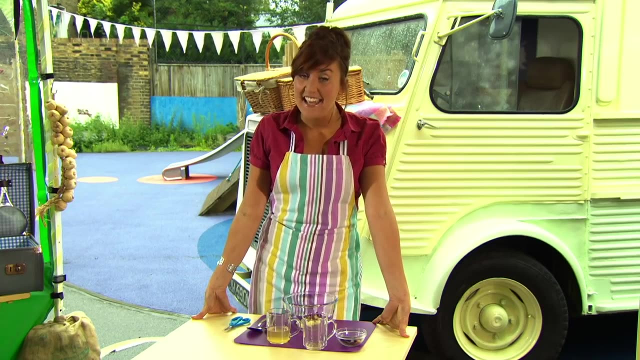 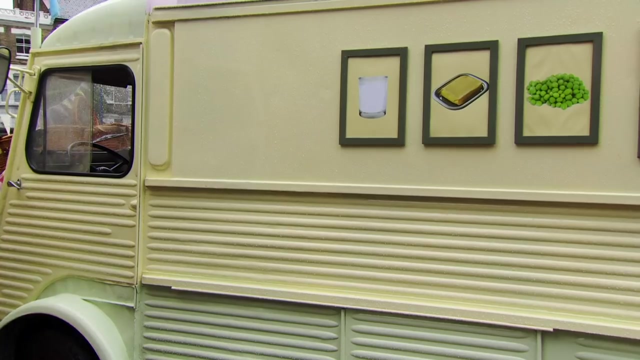 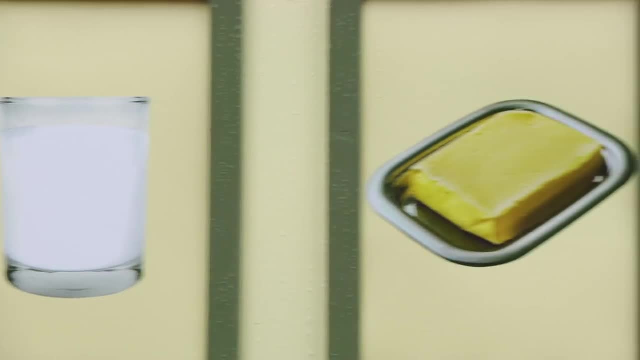 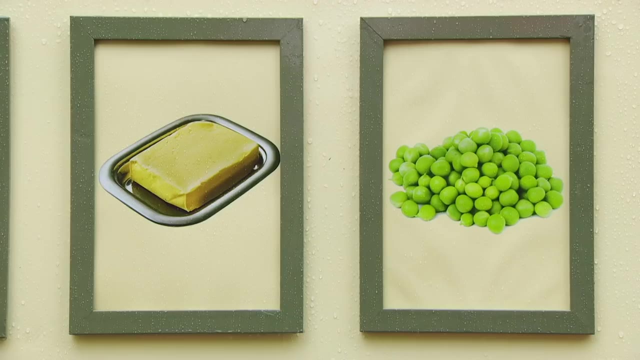 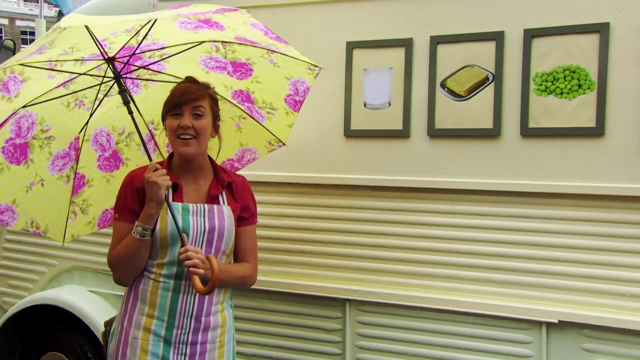 So we've got some milk, some butter and, ooh, some peas. What would you choose for our fruity phyllo parcels? The special ingredient comes from cows. Peas don't come from cows, do they? They come from plants, So we can definitely take that one away. 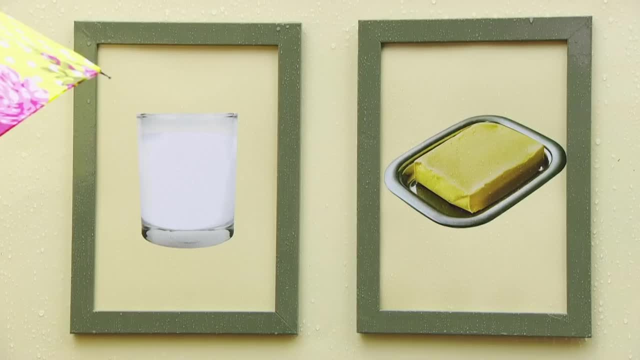 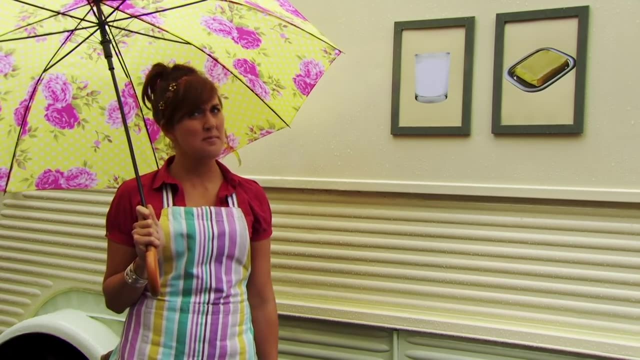 So here's another clue: Special ingredient comes from cows, and you can spread it on toast. Well, you can't spread milk on toast, can you? That would be extremely messy. So we can take that one away too, Which leaves us with butter. 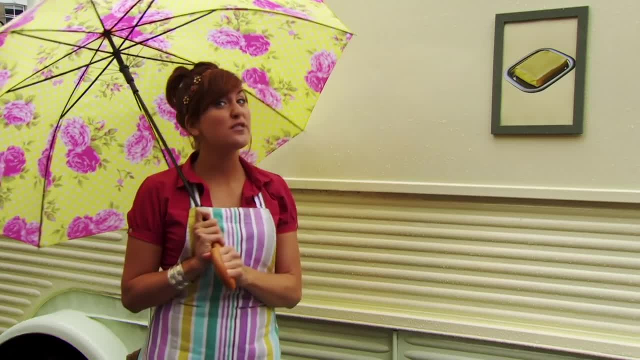 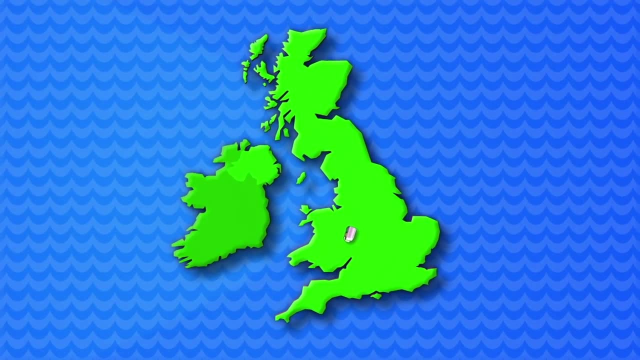 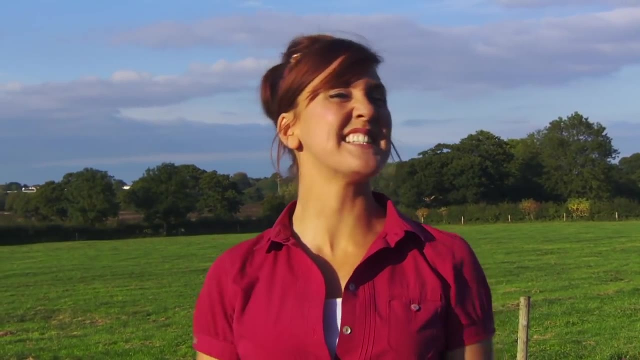 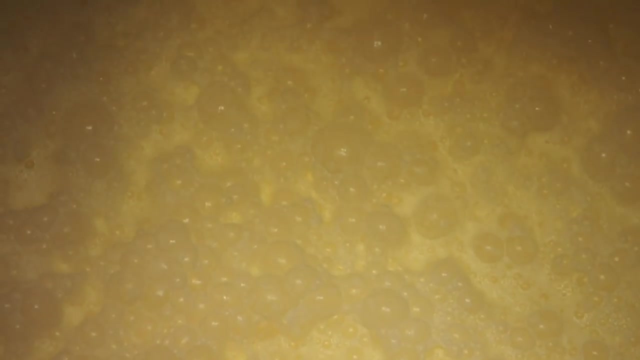 We're going to need some butter for our fruity phyllo parcels and I have been to find some. I've come to Rawton in Wiltshire to find out how butter is made. Let's go and find out. Butter is made from cream collected from cows. 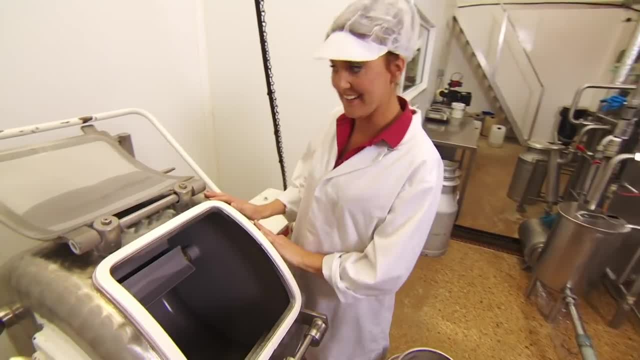 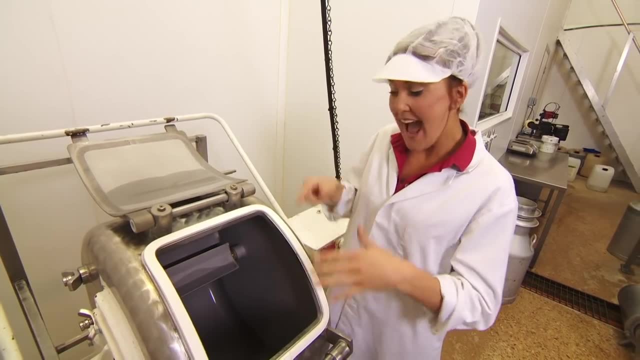 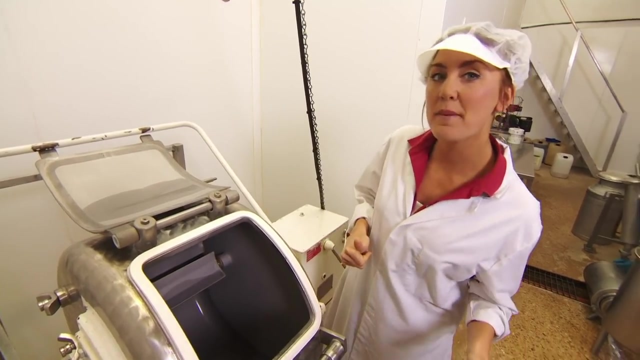 The cream gets poured into this machine- here It's called a churn And it's a bit like a washing machine because it goes round and round and round And it separates the cream into solid butter and into a liquid called buttermilk. And I'm going to help Dave from the dairy pour this cream into the churn. 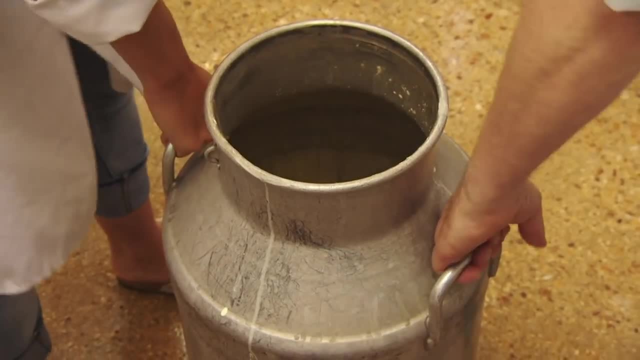 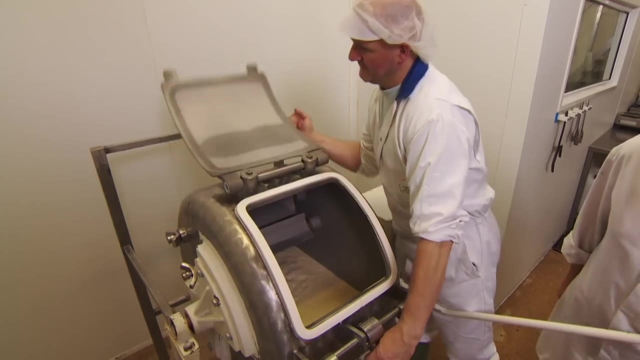 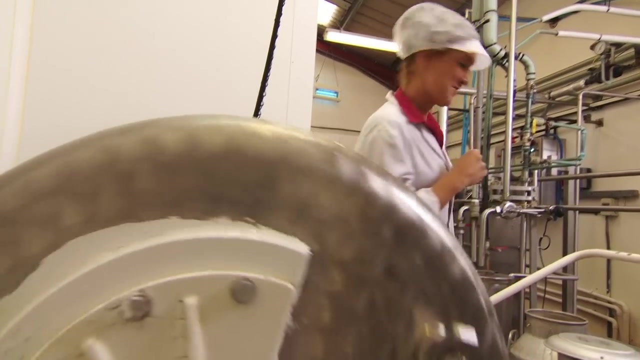 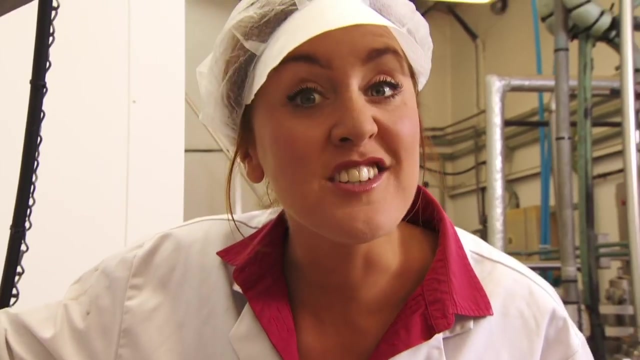 Ready, Dave, Yep, Okay, Ooh, it's heavy. Wow, look at all that cream. And now we just need to close it and switch it on And that spins around for about 40 minutes. Wow, look at that. All we need to do now is drain the buttermilk. 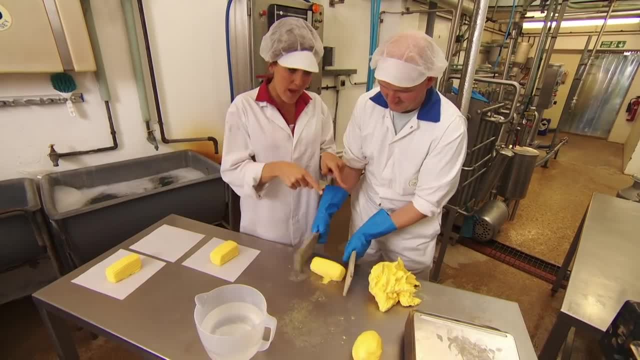 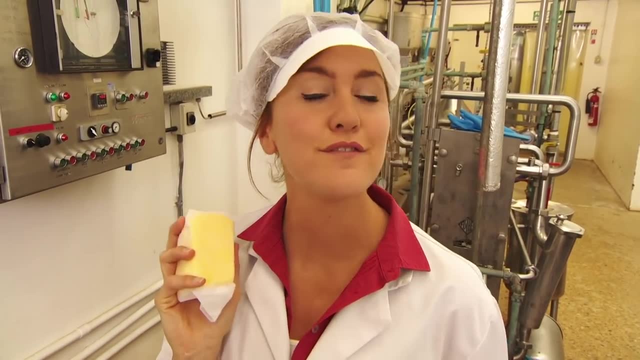 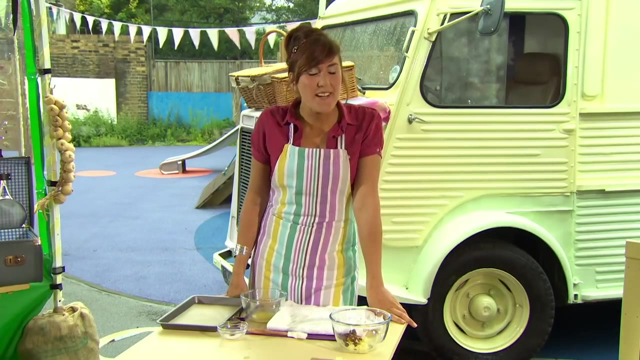 After that the butter is weighed and then we pat it and wrap it And that is going to be perfect to use for our fruity phyllo parcels. Thanks, Dave Bye. Butter is so interesting, isn't it? Look, we've got some butter here and we're going to use it in our dish. 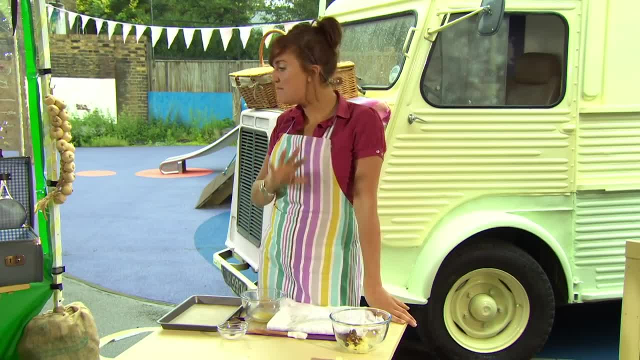 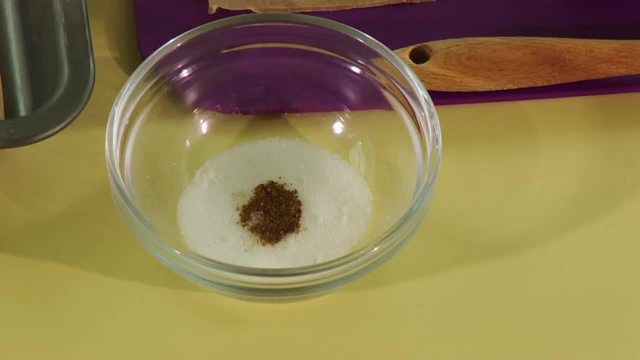 But for this recipe we need melted butter. So I've melted some butter for all of you and it's just the right temperature for us to use, And I've got some other ingredients here which I'm going to add to it. We've got caster sugar and we've got mixed spice, which is going to add a little hint of flavour. 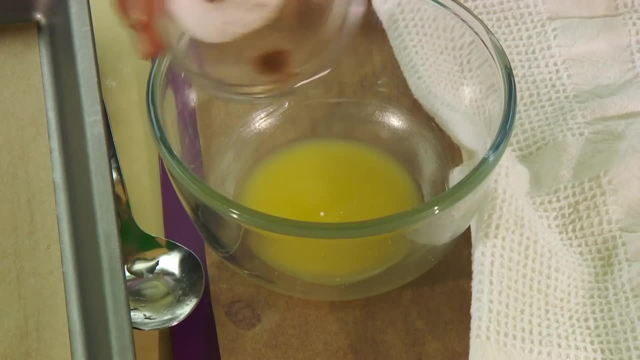 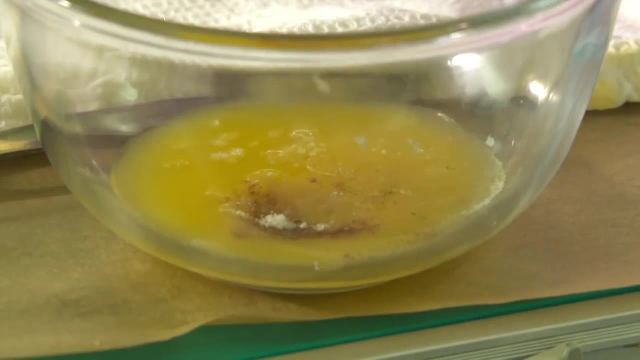 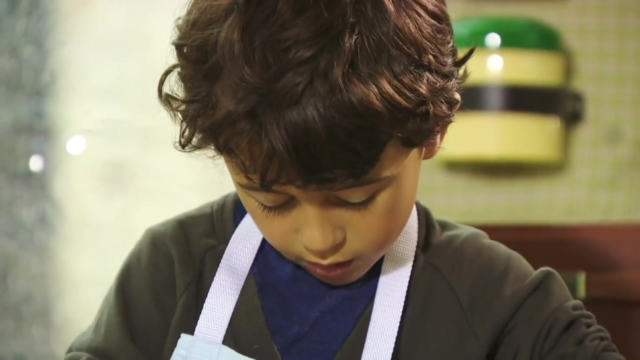 So let's sprinkle it in everyone, Sprinkle, sprinkle, sprinkle, Sprinkle, sprinkle, All, All of it. What happens when it goes into the butter? It turns a different colour. It does indeed. The butter swallows it all up, doesn't it? 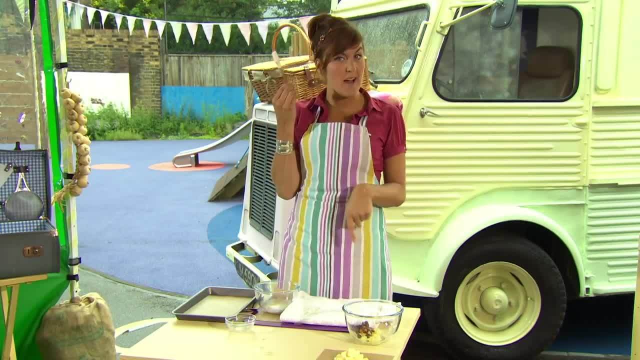 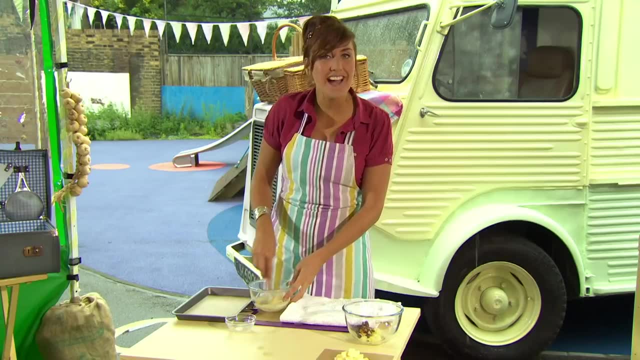 And we're just going to use our brush to mix it up like this. It's a bit like mixing paint, isn't it? Yeah, Why don't you do some mixing at home? You can get your bowl and get your brush. Have you got them? 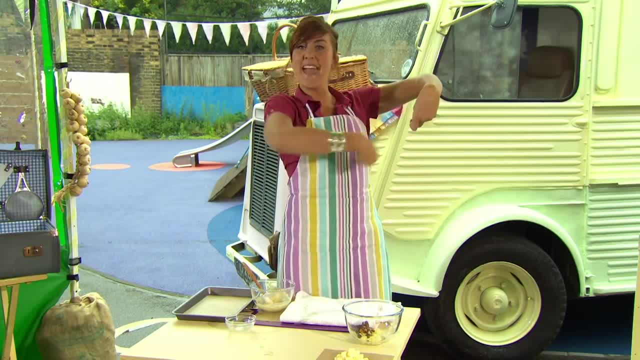 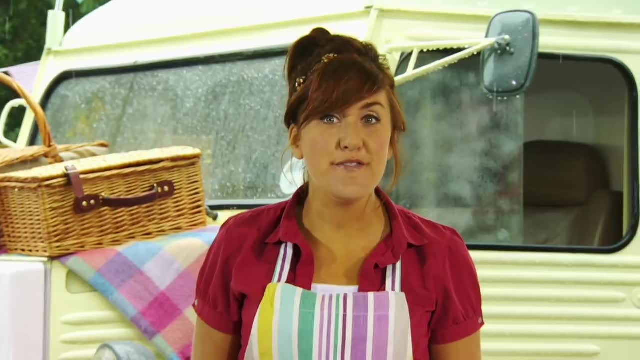 Good, good, And we're going to go mix, mix, mix With your brush With your brush, as Lena says. Next, we're going to use some phyllo pastry, which is a lovely type of pastry that goes yummy and crispy when it goes in the oven. 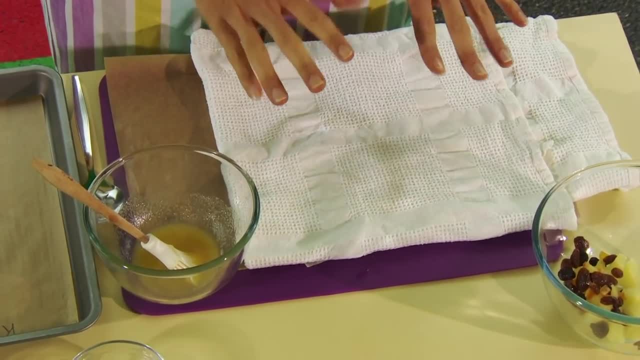 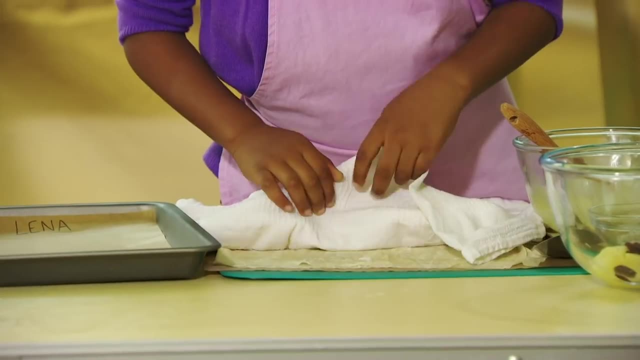 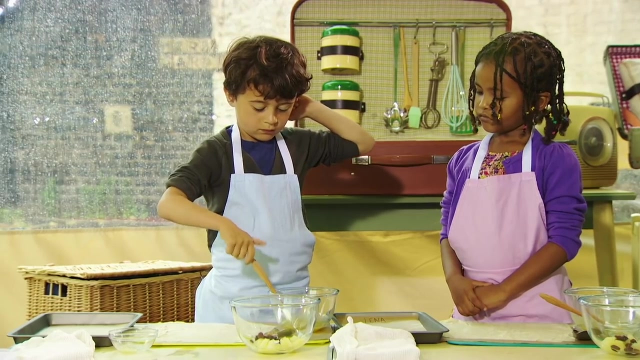 And it's hiding underneath this damp towel so that it doesn't dry out. So everyone, take the damp towel off and look. What does it look like? Aisha, It looks like tissue. Like tissue, It does look like tissue. First, we need to do some dib-dabbing. 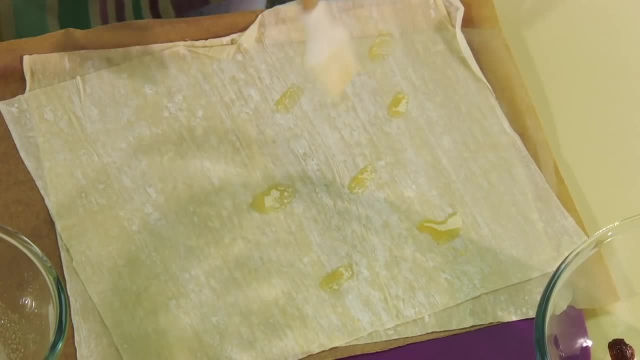 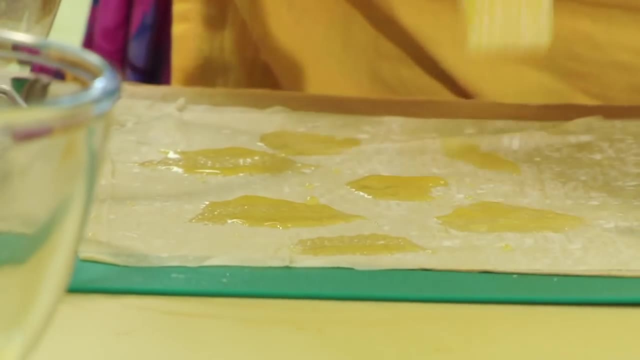 So dib-dab, dib-dab, dib-dab, dib-dab. all over the phyllo pastry It looks like a spotty dog. Dib-dab, dib-dab, dib-dab, dib-dab, dib-dab. 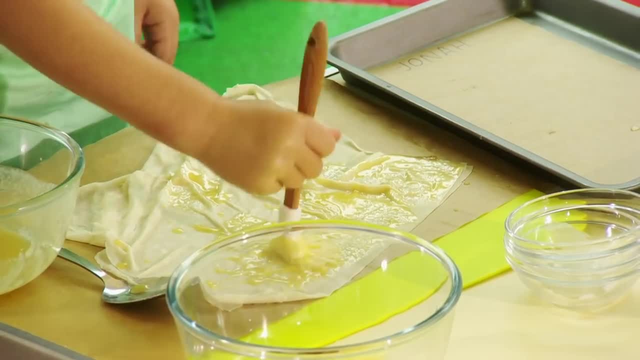 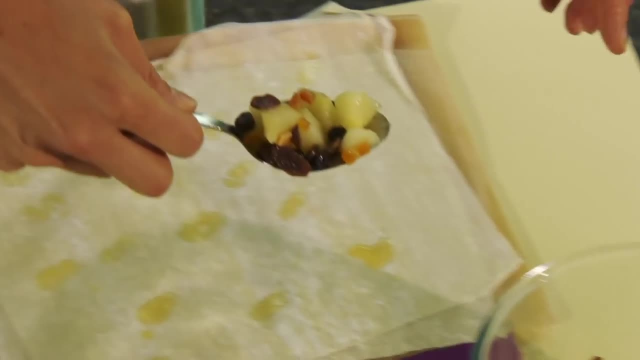 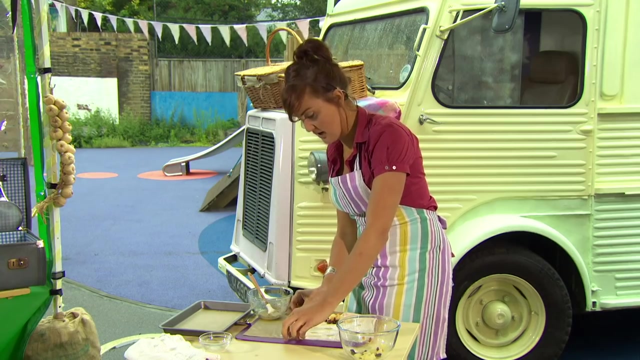 I love dib-dabbing. Now, once you've dib-dabbed, we're going to take a big spoonful of our fruity mixture and put it at the bottom of the phyllo pastry There. Okay, fantastic. Now we need to fold the pastry over on this side. 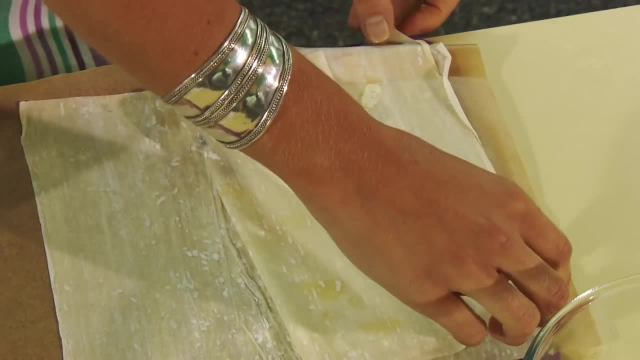 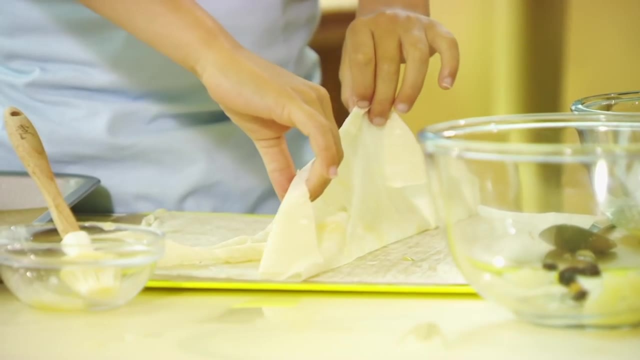 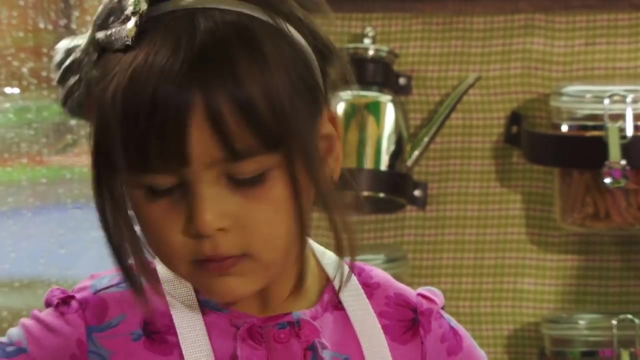 It's like wrapping up a birthday present And then fold the pastry over on this side. Okay, you try that. Next we have to do some more dib-dabbing. So dip your brush in the butter and then dib-dab all over. 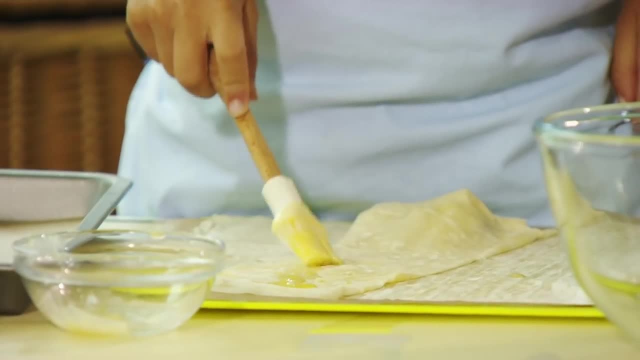 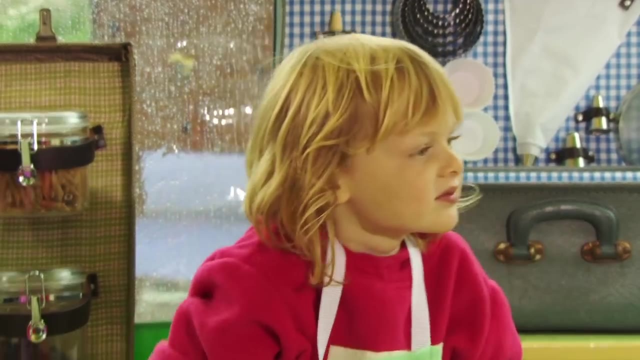 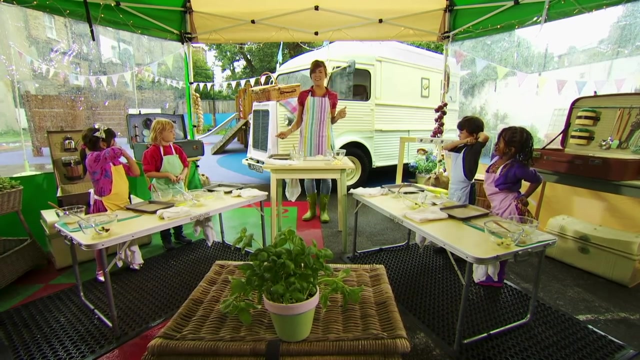 The pastry. The next thing we have to do is the rolly-poly. Can everyone do some rolly-polying like this? Roll up and then roll down and then roll it all around. Let's do that again really quickly, but this time you can join in with us. 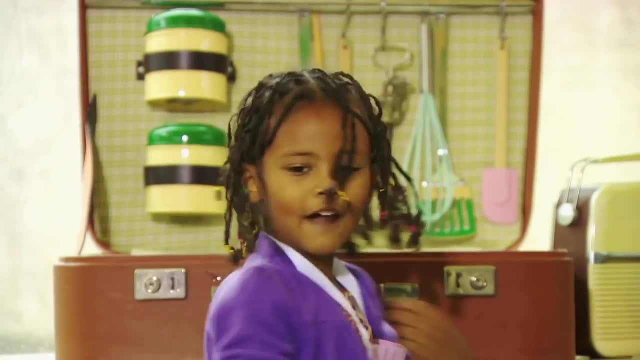 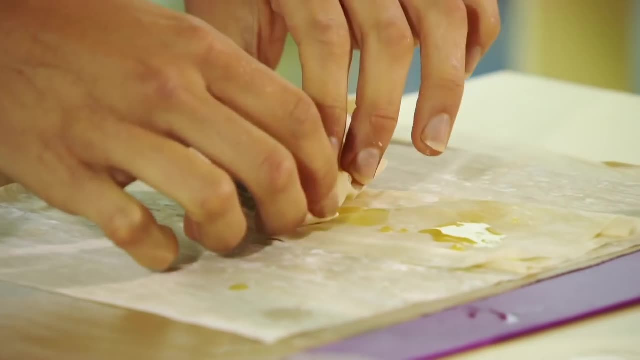 Roll up, roll down and roll it all around. Who's ready to do some rolling Me? Okay, we have to roll our fruity mixture up in our phyllo pastry like this, So it looks like a little phyllo. I've done it. 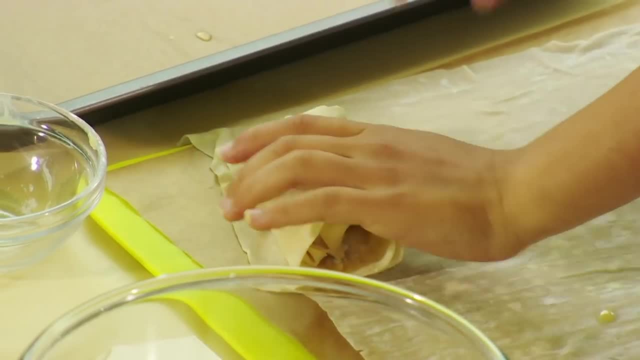 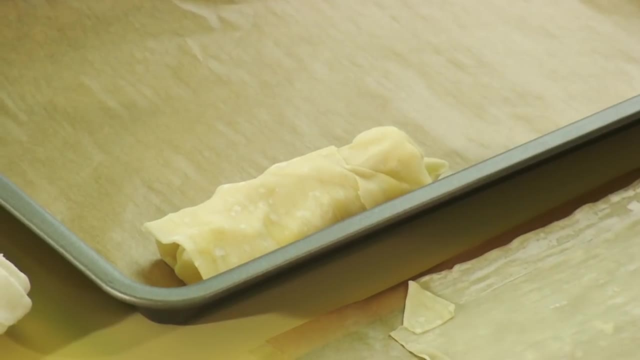 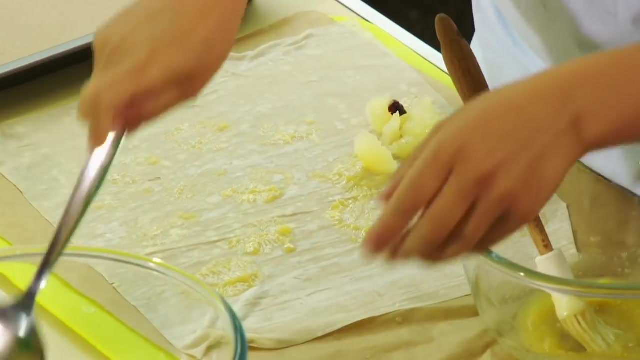 That's it. and then put it onto your tray- Fantastic. And then you have to do it all over again. So you start by dib-dabbing your piece of pastry, Dib-dab, dib-dab, Spoon up our mixture and then wrap it up like a birthday present. 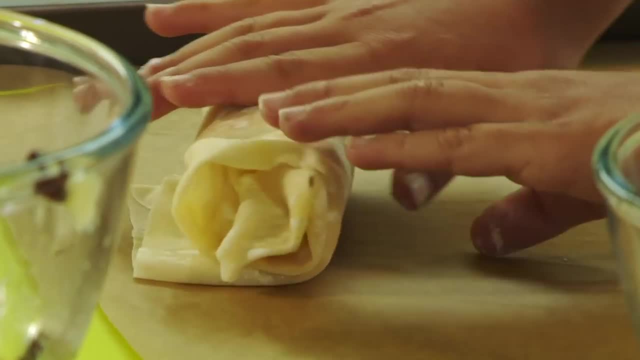 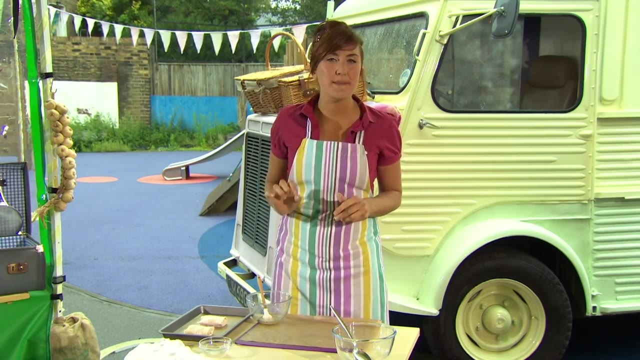 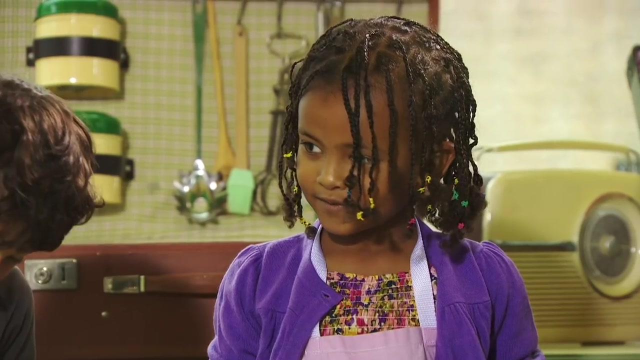 And then you rolly, Rolly And that is it. But the very last finishing touch is to give it a quick dib-dab of butter before we put it in the oven. I think it's going to taste nice. In fact it's going to taste incredible. 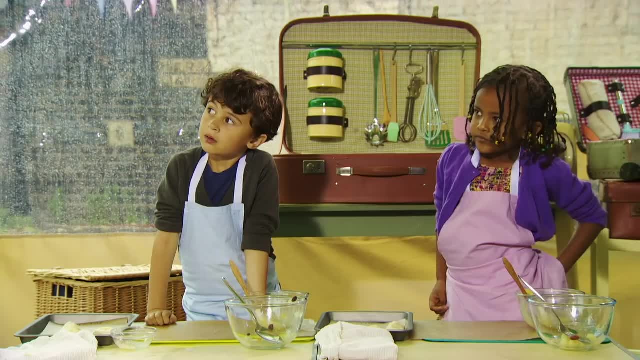 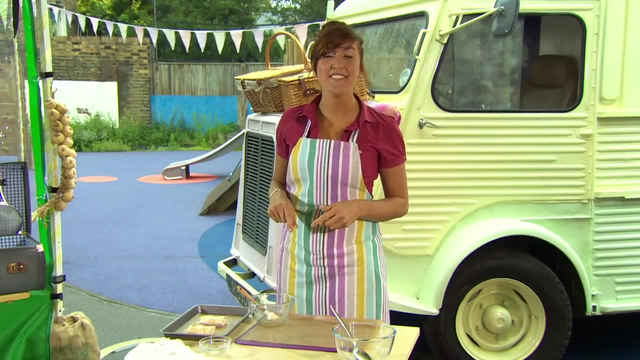 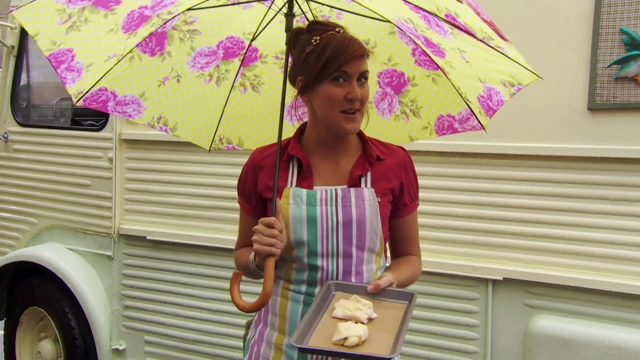 And that everybody is it. You've done it. You've put all the ingredients together for your fruity phyllo parcels and you did it all by yourself. Now it's time to put them in the oven to cook. But remember, ovens are hot, so don't go near. 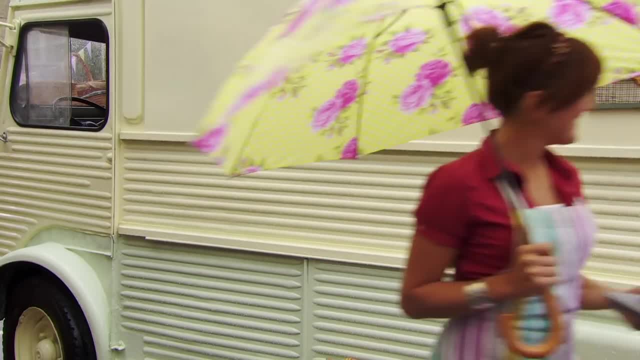 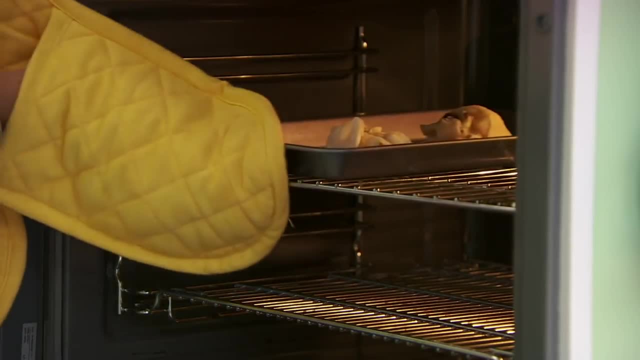 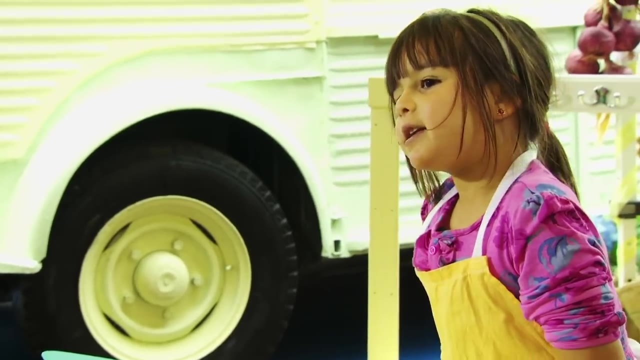 Ask a grown-up to help you here. Now we've cooked with you and had lots of fun. Let's tidy up and think of all the things that we have done. There was Best way. Dabbing Rolly Now, clearing any mess and putting things away is always fun to do. 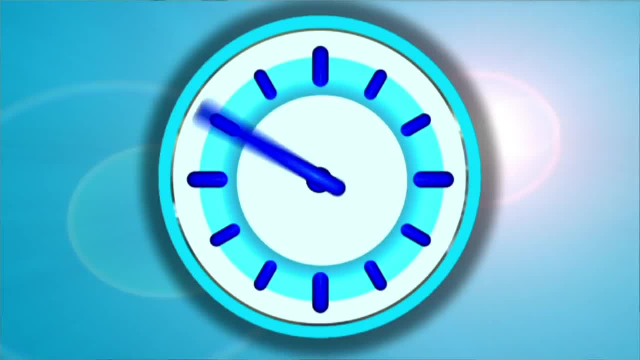 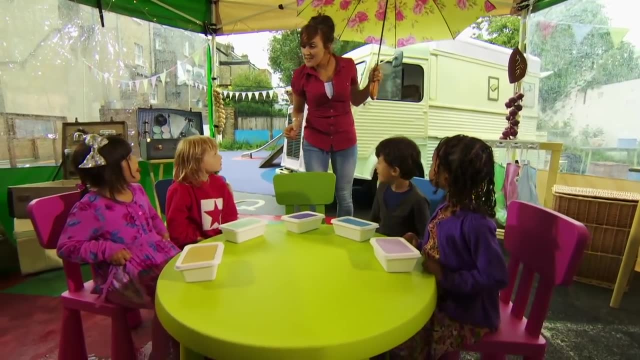 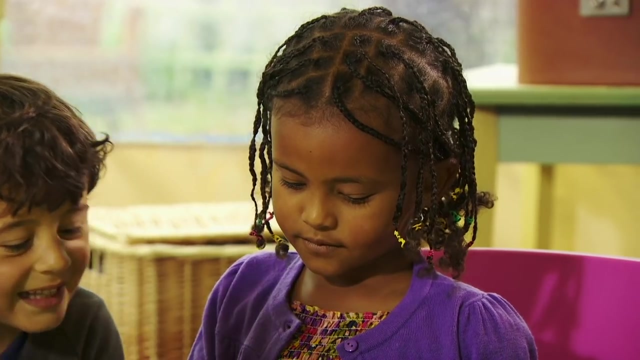 At the end of the day. Look everyone, our food's all cooked and it smells so delicious. Can you smell it? Yes, OK, Lina, let's have a look at your one. Ooh, What's happened to the phyllo pastry? 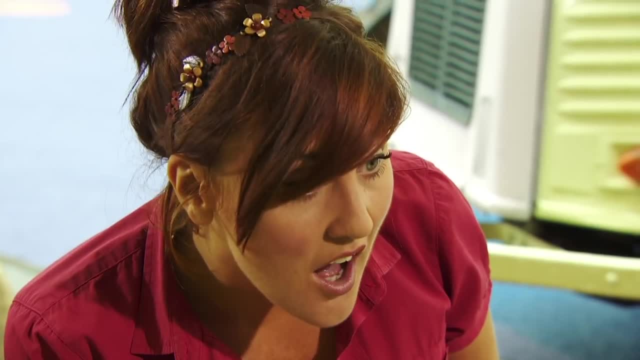 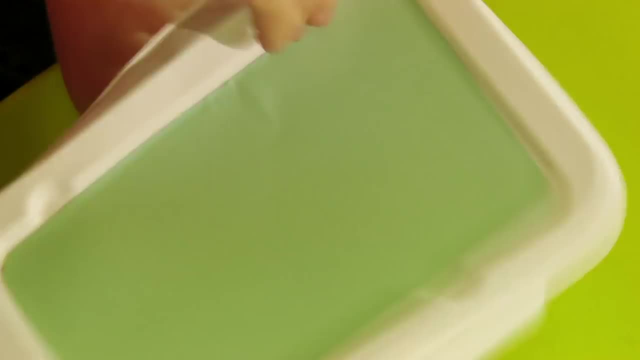 It's not soft anymore. It's gone really hard and crispy, hasn't it? Because you put it in the oven. You've got it, Lina. Let's have a look at Jonas. Oh, look, what's happened to it, Jonah. 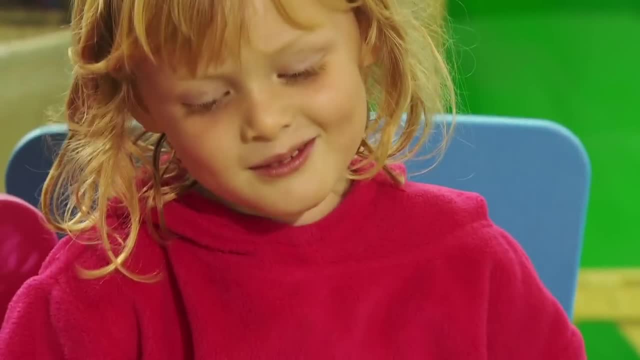 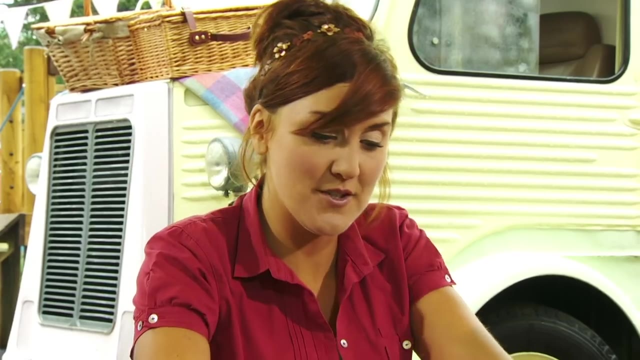 It has exploded in the oven. And what's coming out of it? Raisins. Let's put the lids on top and we'll save this lovely food to eat later on with everyone else. We've travelled to you, we've cooked and had fun. 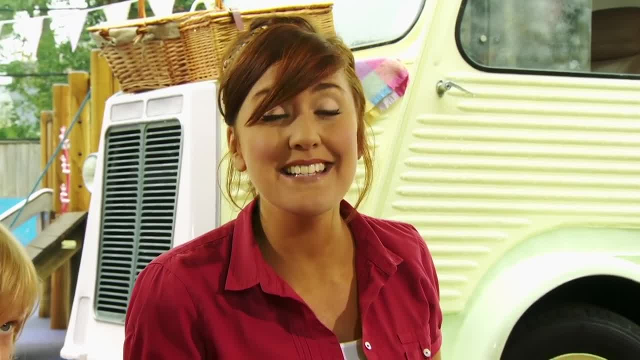 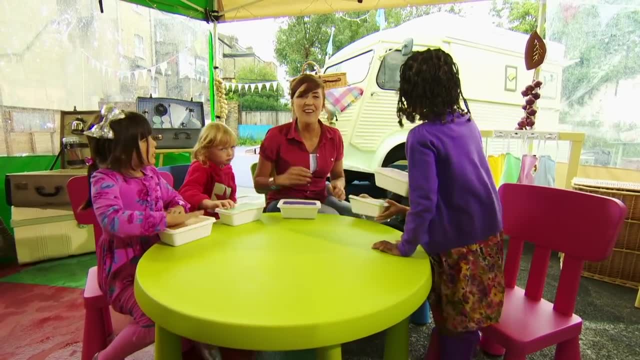 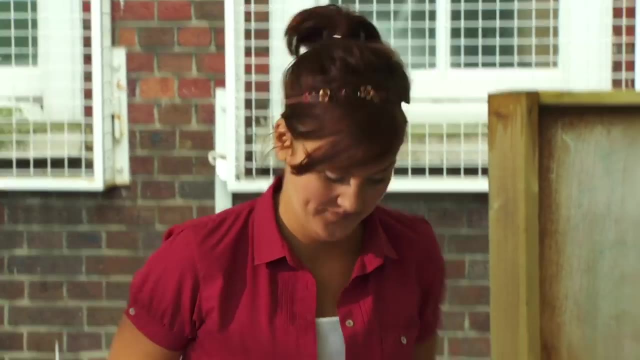 Now let's have a party with everyone. Yeah, Come on, you can come with us, Follow me, OK, Let's go. Well, here we are and we've got our food, so let's tuck in Mmm. 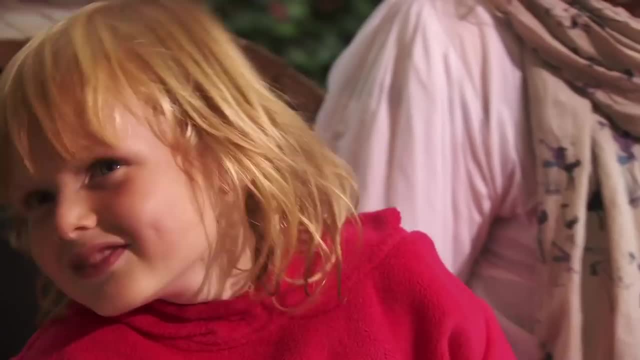 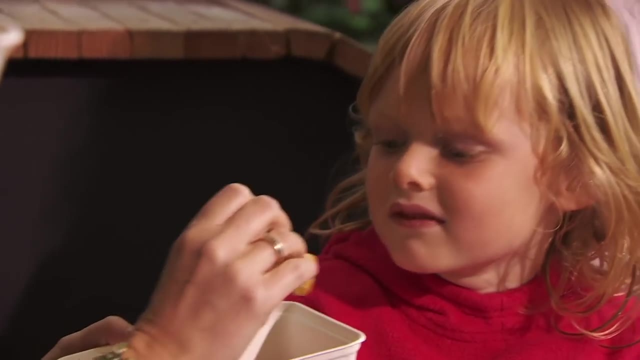 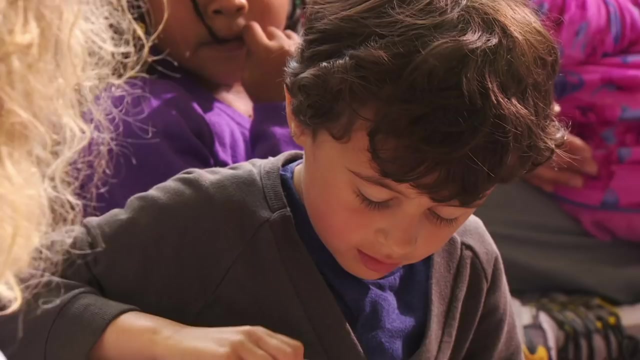 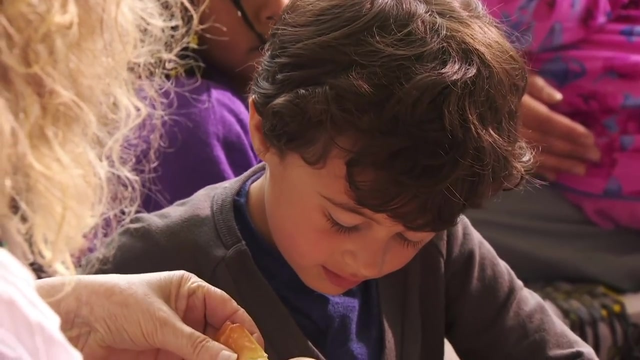 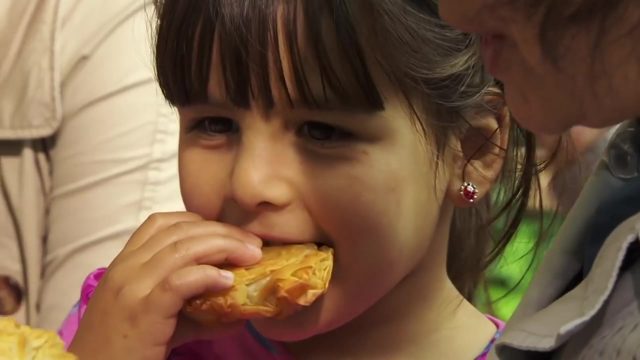 That is so yummy. What about the present? Mmm, It tastes like cake. It does taste like cake. Oh, wow, that looks amazing. May I take some? Ooh, they're nice Crunchy. Did you have fun? 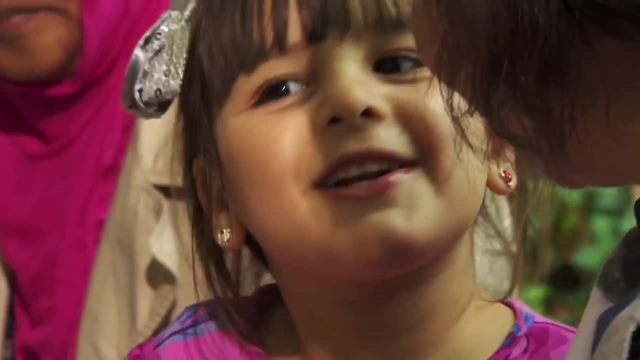 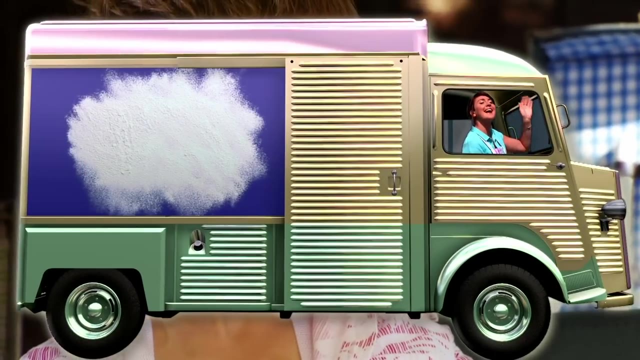 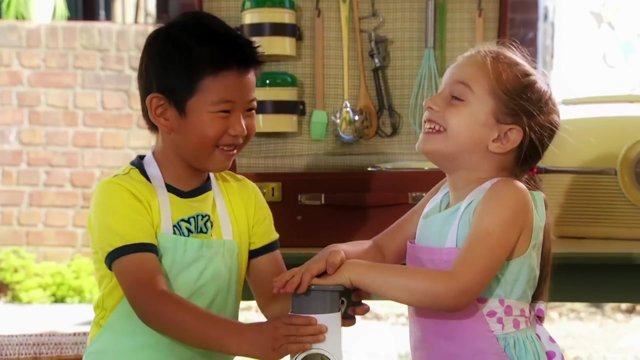 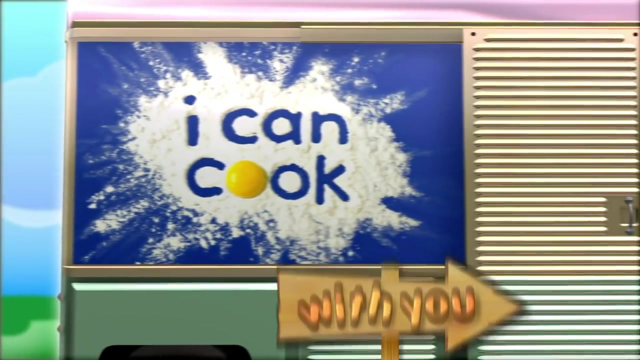 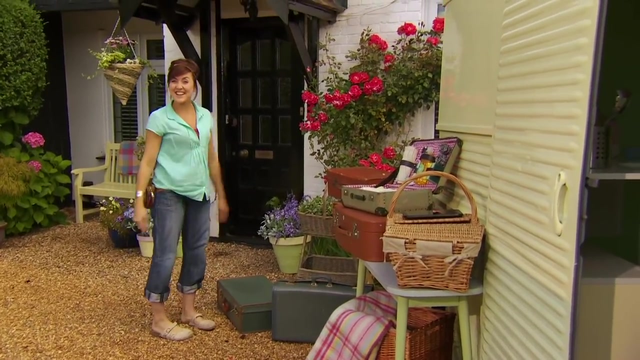 It's hot. Oh, you gave me the heart, Lovely. So what can you do? everybody, I can cook, I can cook. I can cook With you. Hello, Oh, it's good to see you. I'm just getting everything ready to go on a journey. 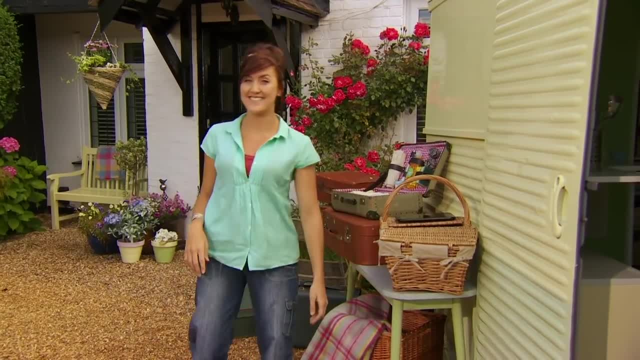 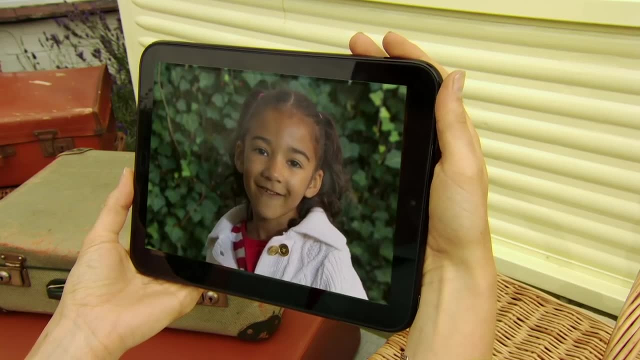 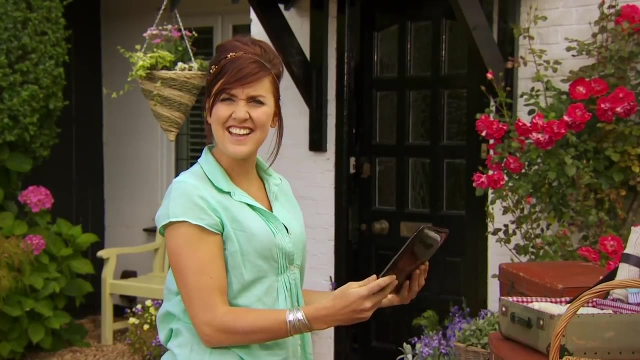 I hope that you're going to come with me and make some new friends. Aha, Hello, Katie, I love riding my scooter. My favourite food is cheese and pasta. Katie, Katie, can you cook with me please? I can, and that sounds like loads of fun. 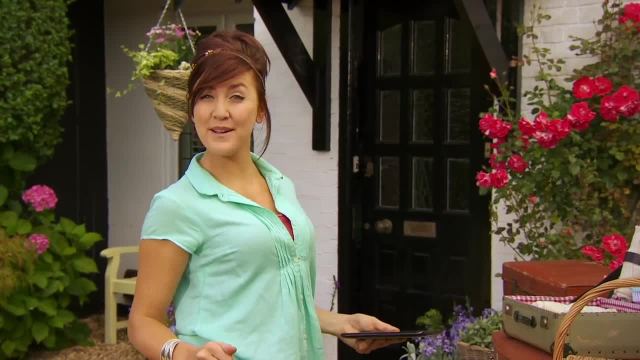 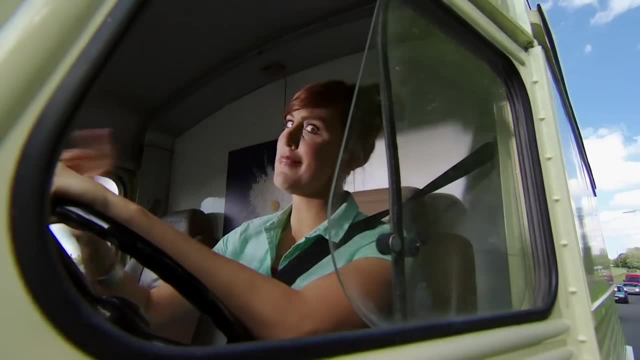 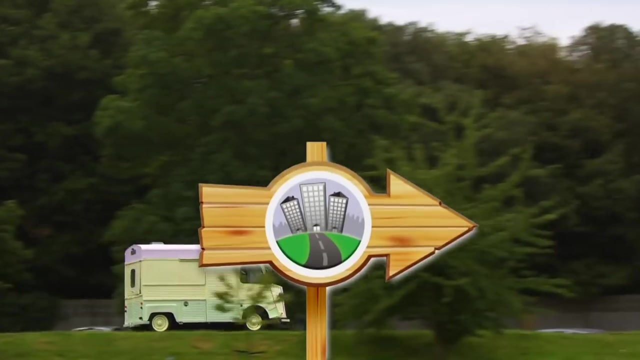 And you can cook with me too. Let's pack up and go Off on a journey, and I'm coming to you. It's going to be busy and there's lots to do. Get ready to help, join in and have fun. Let's cook a feast for everyone. 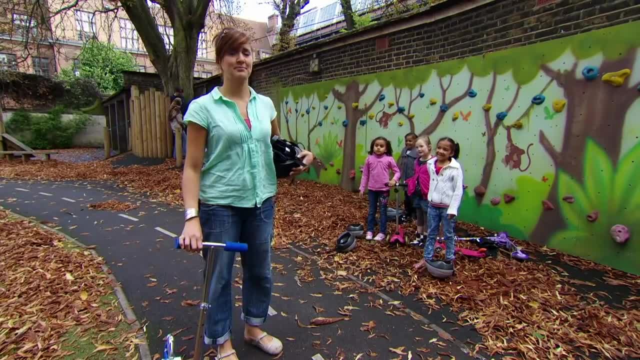 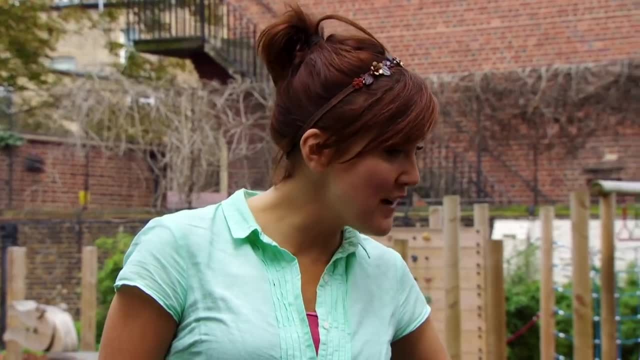 Well, I've got my gear and I am ready to do some scooting, But where's Jada? Oh, there you are. Hi Jada, Hi Katie. So, Jada, are these all of your friends? Yeah? 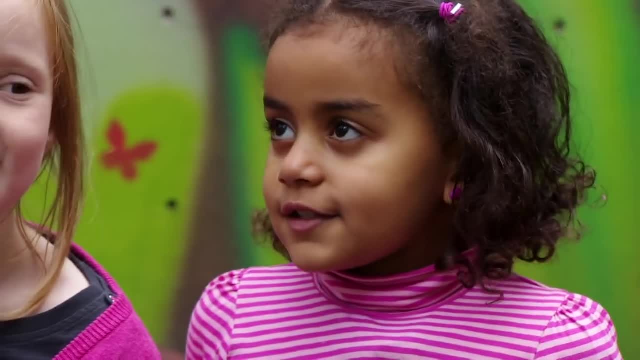 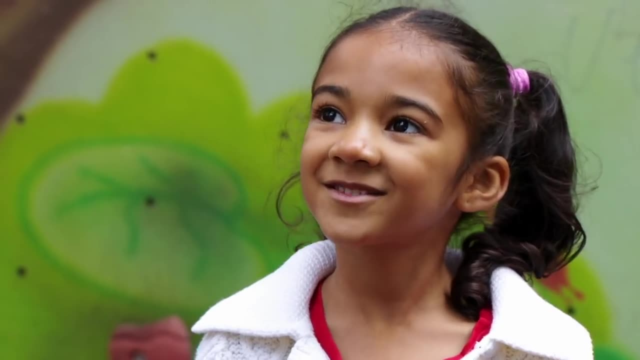 What's your name, Kaya Freya, And what's your name, Fatima? Well, it's fantastic to meet all of you. I'm really excited. What are we going to do today? Jada, Make something with cheese and pasta and ride in our scooters. 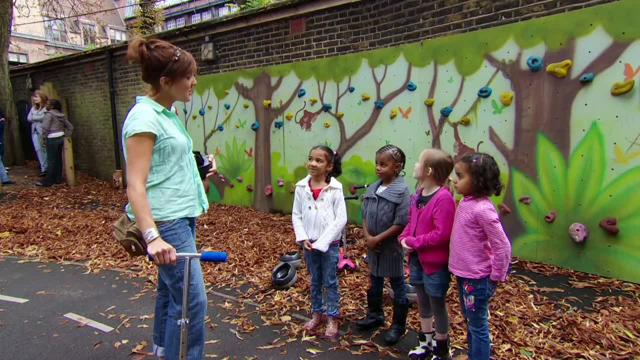 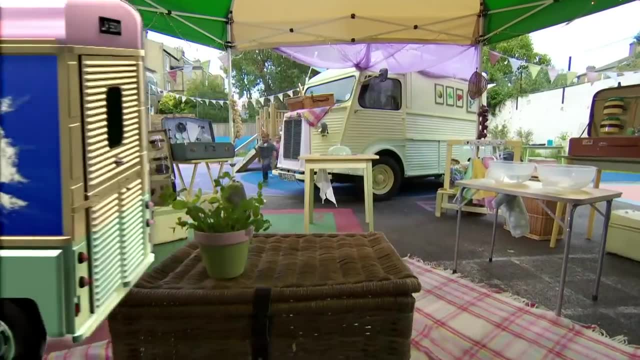 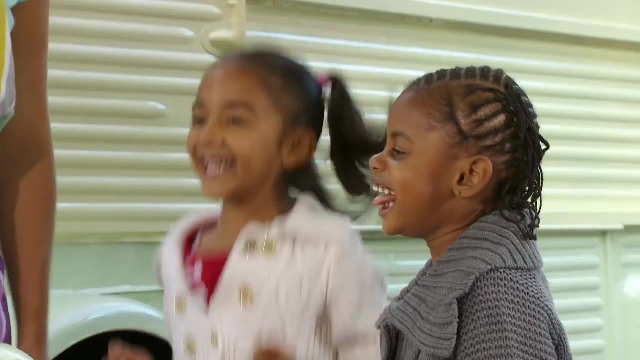 I have got the perfect recipe for us to make. Shall we go and do some cooking, girls? Yeah, Come on, let's go This way. Welcome to my outdoor kitchen. Who's excited Me? Me too, actually. Who wants to know what we're going to cook today? 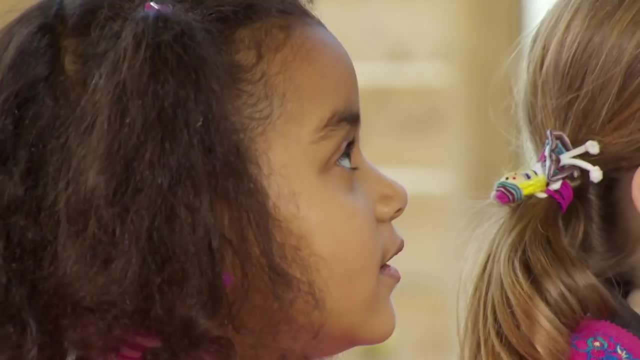 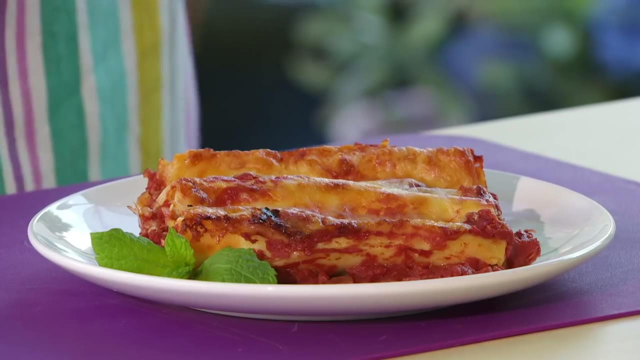 Me. Well, today we're going to cook cheesy pasta rolls. Look at this. Wow Smells good, doesn't it? Yeah, Now, before we get started on the cooking, we've got to do something really important first. What do you think it is? team? 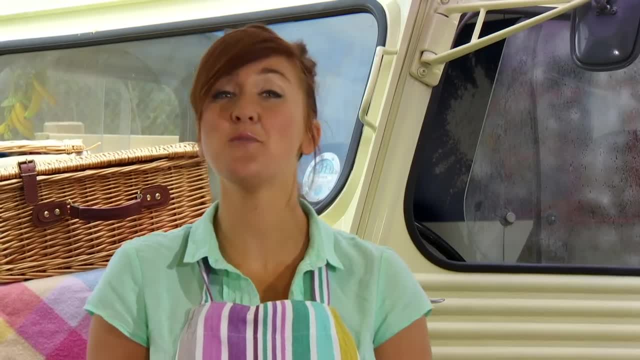 Wash our hands. Of course We have to wash our hands. Let's go, everyone. Roll up your sleeves, Give your hands a wash With slippy, dippy soap. Splish, splash, splosh. Have you done your hands? 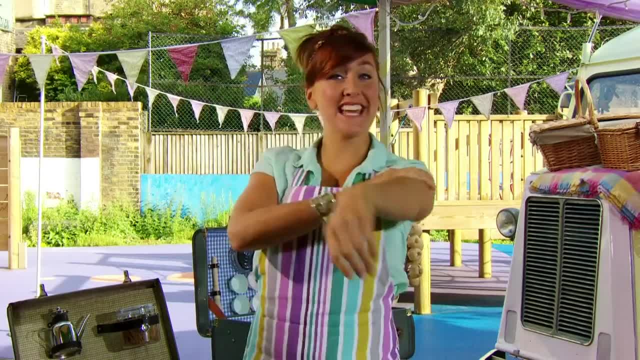 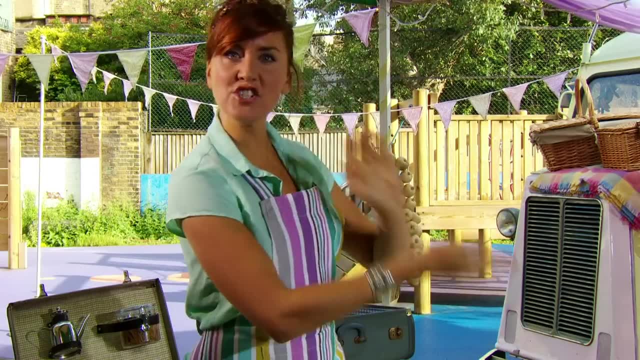 Washed and dried, Sleeves rolled up, Apron tied. What can you do? I can cook. Right then, everyone, Let's get started on our cheesy pasta rolls. Are you ready? I'm ready, I'm ready, I'm ready. 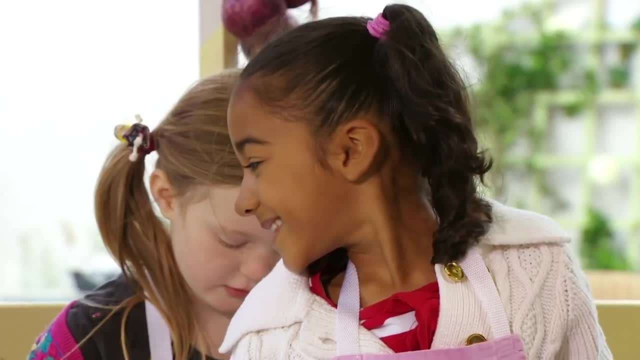 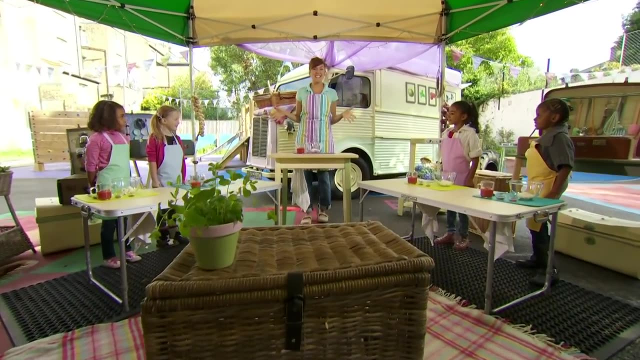 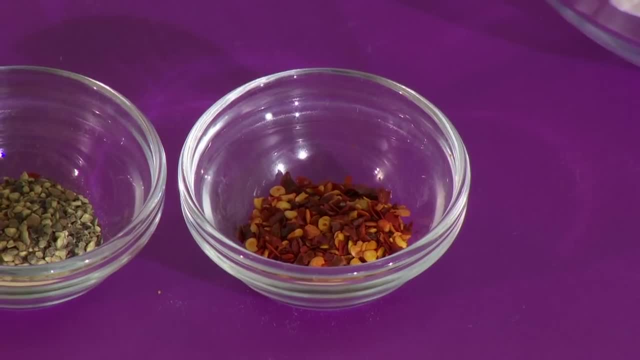 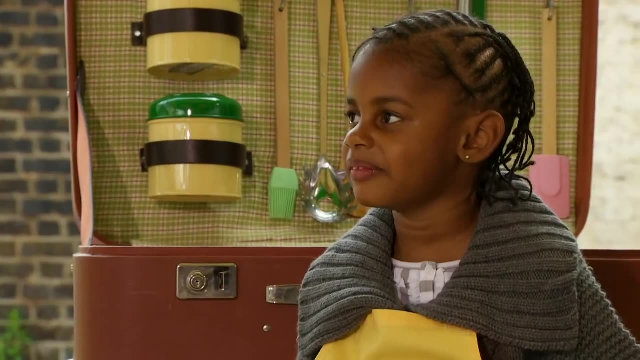 Yeah, Now the first ingredient we need is chili flakes, And chili flakes are going to add a really great flavor. They're going to add some Kazam to our recipe. Can everyone go? Kazam, Kazam? And we need a pinch of these chili flakes. 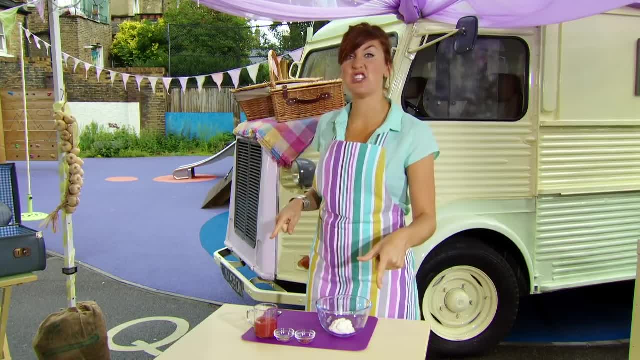 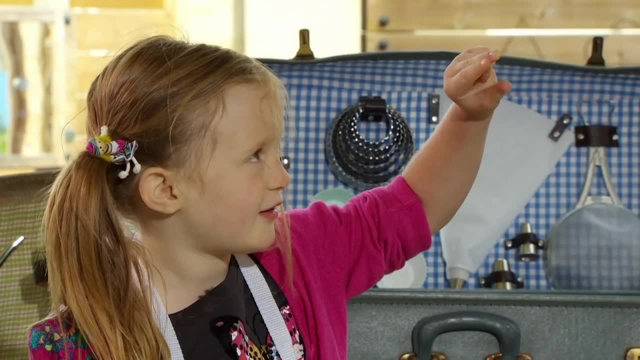 And for that we need our pinchy parrot. So, make a pinchy parrot. you do this, You put your thumb down, like that, And then we put our two fingers on top. Can you do that? Yes, And then you do a really big squawk, like this: 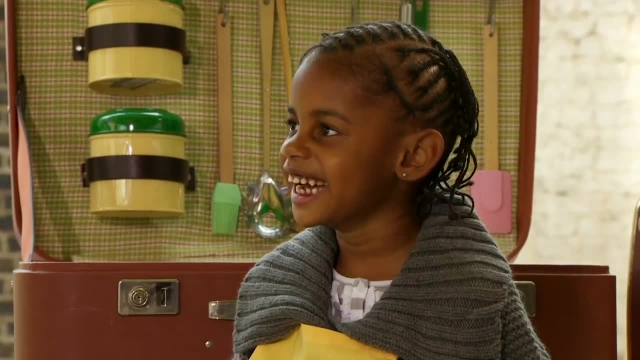 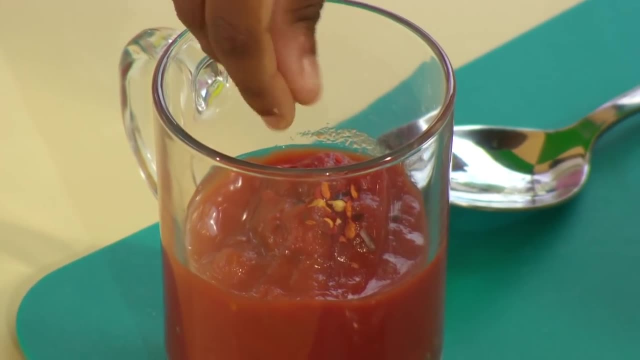 Quack And then take a pinch of chilli flakes with your pinchy parrot and put it into this cup of chopped tomatoes. We're going to wipe our hands because the chilli flakes have got a really strong flavour so we don't want to get them anywhere near our eyes. 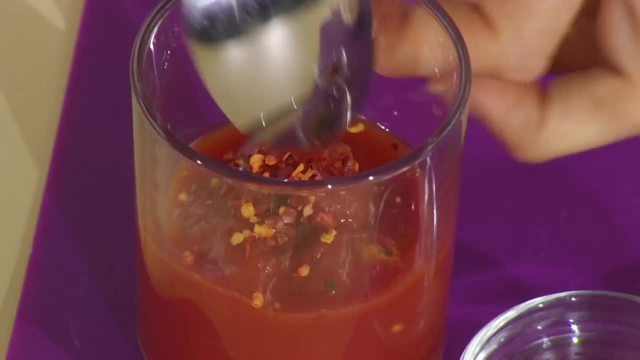 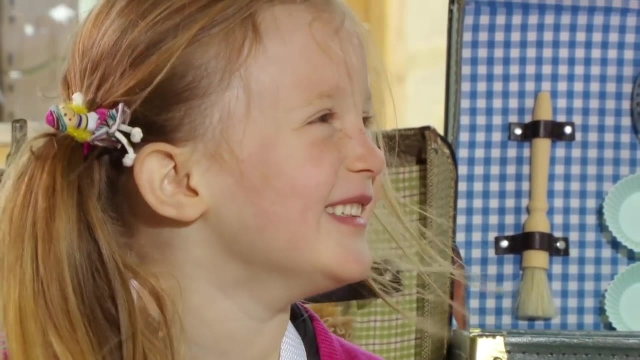 And then you're going to take your spoon and mix them in. What's happened to all the chilli flakes, Freya? They've gone into the tomatoes. Yeah, they've disappeared, haven't they? OK? next we need our pinchy parrots again. 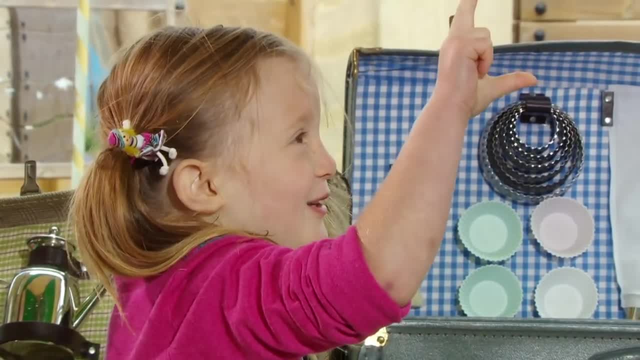 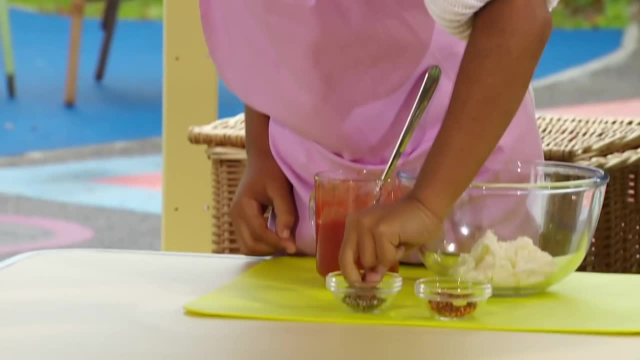 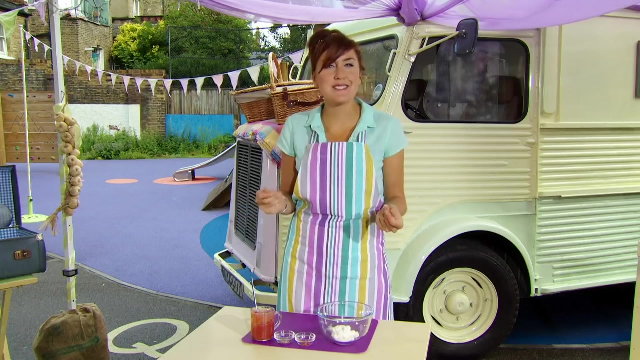 Where's your pinchy parrot girls? They are loud parrots. Take a pinch of pepper and we're going to put this into this bowl here of ricotta cheese. This is a really lovely cheese that's really smooth and creamy. I wonder what ingredient we're going to need next for our cheesy pasta rolls. 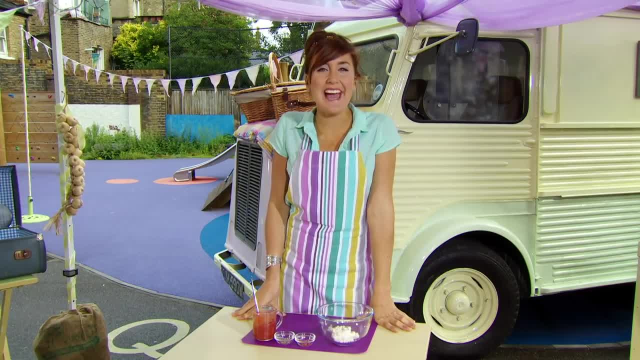 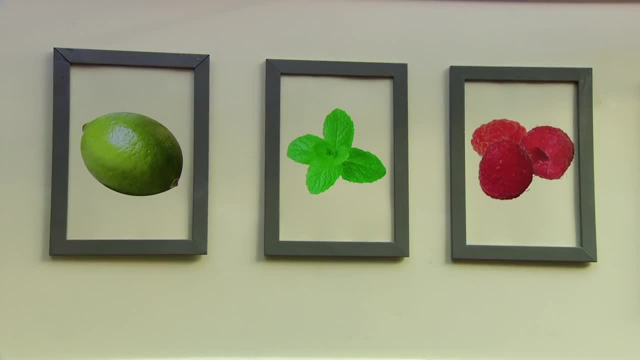 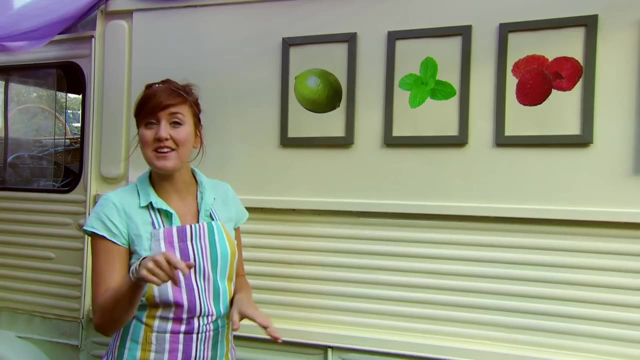 What's next? Well, let us see. Let's see if you can guess what it could be. So we've got a lime, we've got some mint and some raspberries. What would you choose for our cheesy pasta rolls? I'll give you some clues and then you can try and guess what it might be. 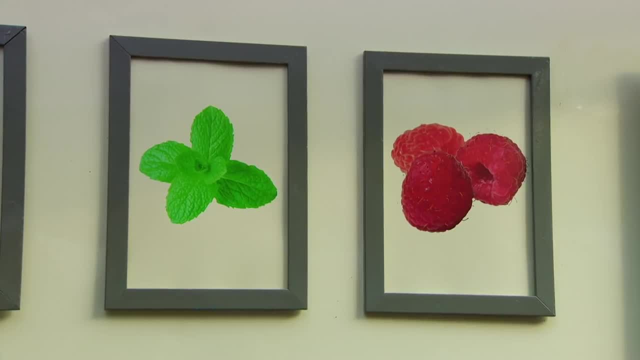 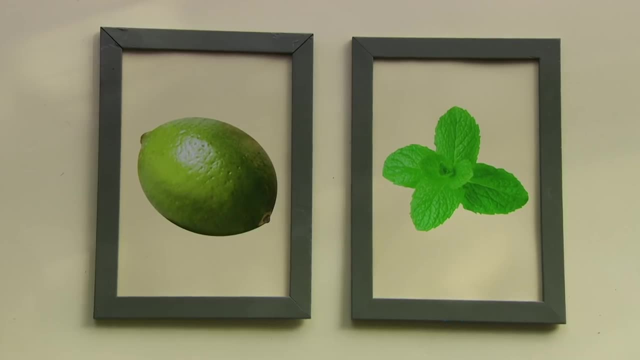 The special ingredient is green. Well, raspberries are red, aren't they? So let's take that one away for a start. Here's another clue: The special ingredient is green and it's a herb. Well, lime Limes are green, but they're not a herb, are they? 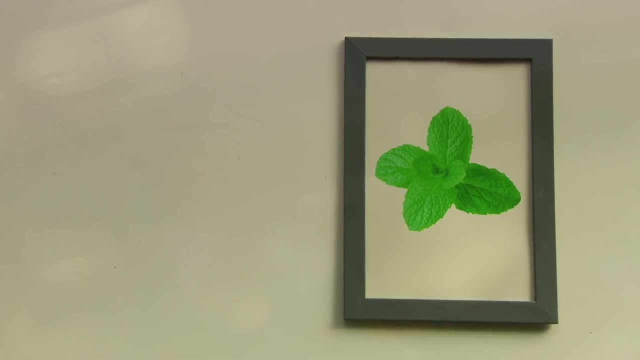 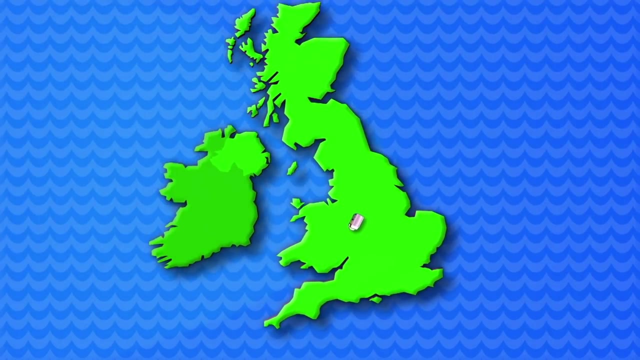 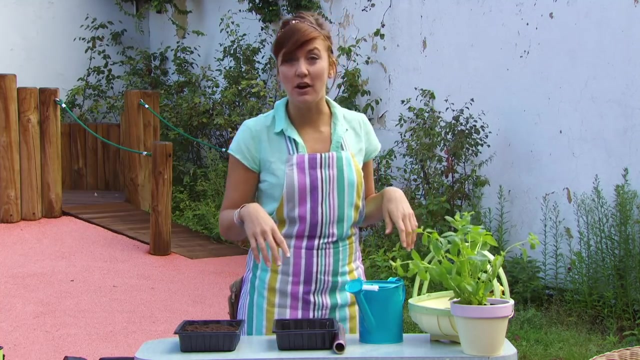 They're a fruit, So let's take that one away as well, which leaves us with mint. We're going to need some mint for our cheesy pasta rolls Now. mint is something that you can easily grow, and you don't even need that much space to do it either. 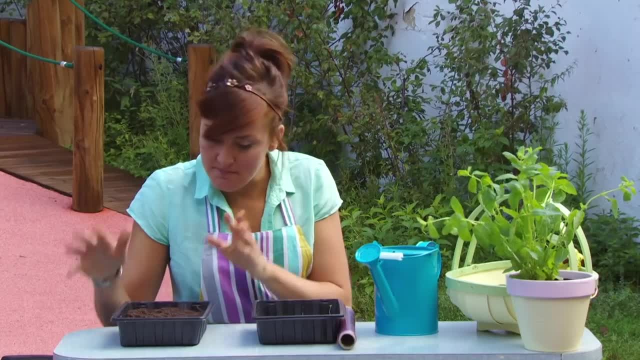 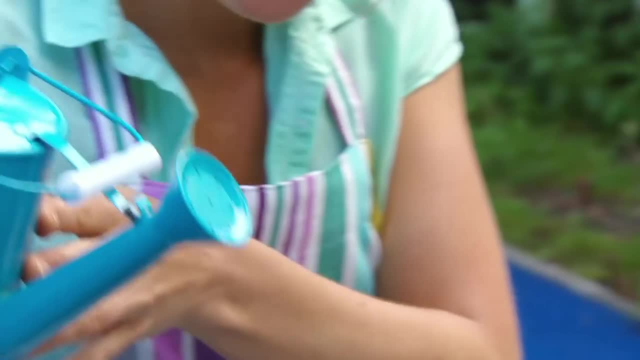 The first thing you're going to need is a little tray like this and then put some soil inside of it, But we need to keep the soil nice and wet, So we're going to give it a little water. first of all, Give it a drink. 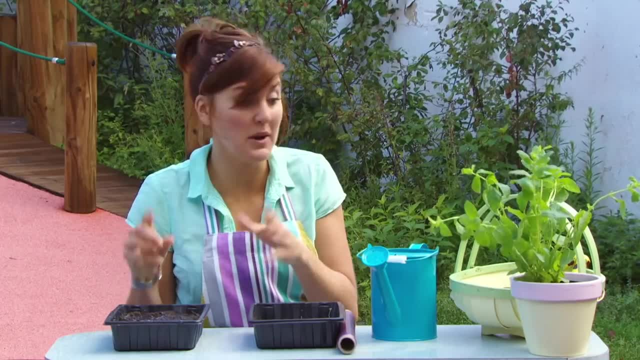 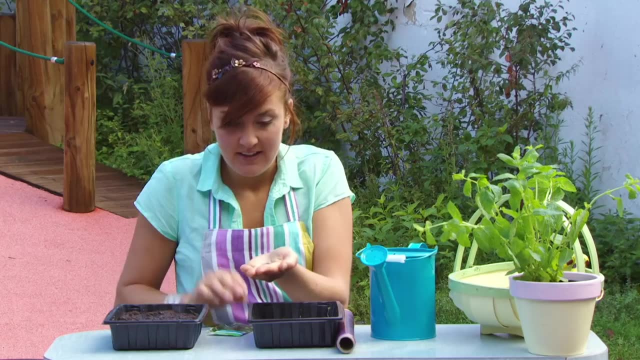 And once that soil has soaked up all of the water, we're going to need our mint seeds, which we've got over here. And look at these: They are so, so small. Now we're going to sprinkle these seeds all over the soil. 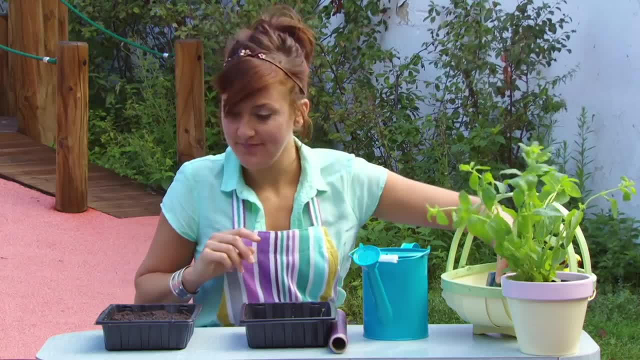 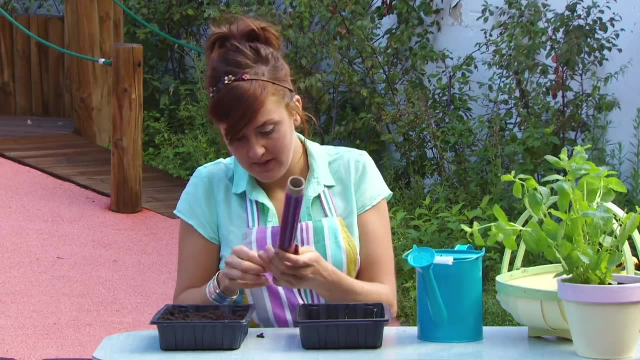 You can't even see them once you spread them. There we go, And then we're going to cover the seeds with all the soil And we need to keep them really nice and warm. So we're going to get some cling film and cover them up. 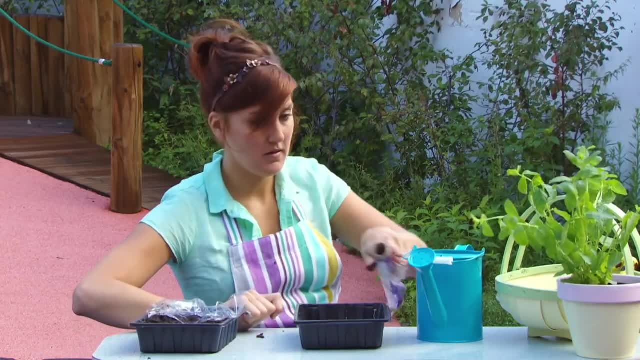 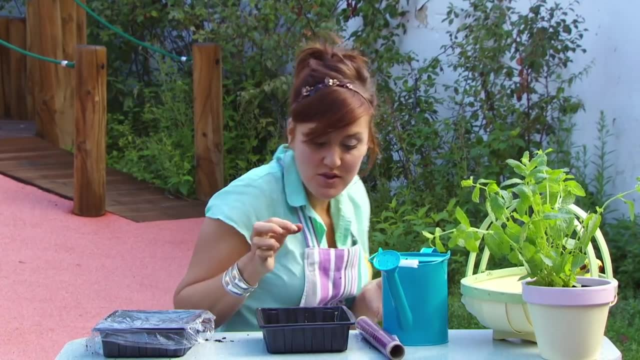 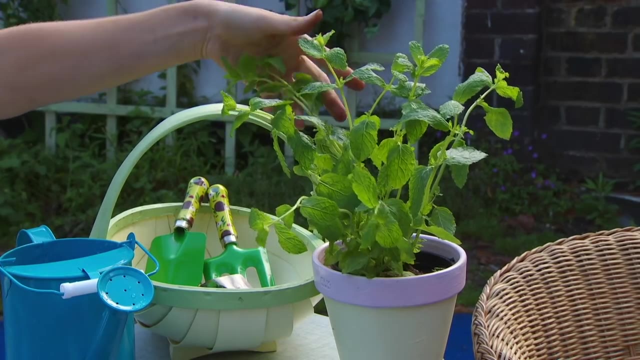 It's a bit like making a little greenhouse, And after a few weeks tiny little green shoots will start to sprout through the soil, like these here Can you see them? Then after about a month you'll get a lovely big mint plant like this one here: 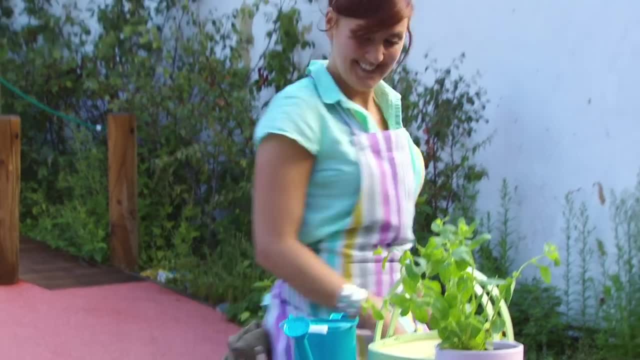 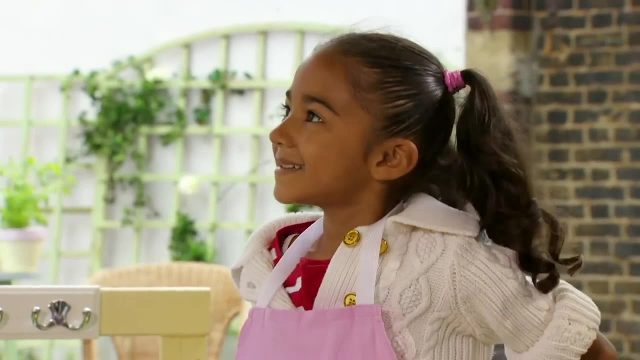 Perfect to use in our cheesy pasta rolls. Look, here's the mint that I've grown And we're going to use it in our recipe. Rub the mint leaf between your fingers like this, Give it a good rub And smell it. 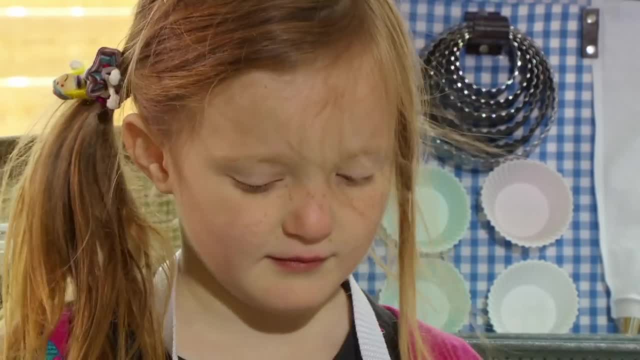 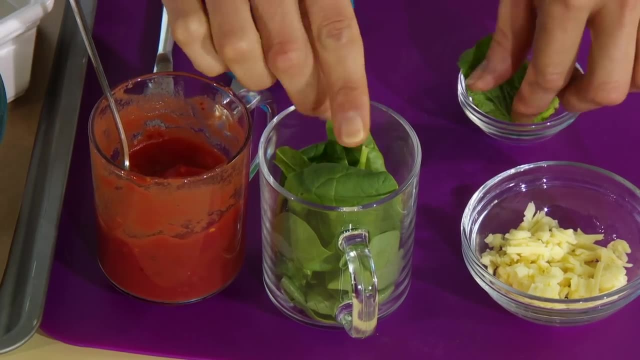 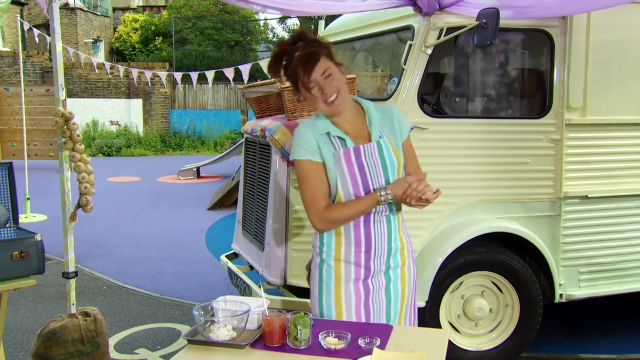 Amazing, isn't it? We've got a cup of spinach leaves over here And we're going to count five mint leaves into our spinach. So let's count Ready: A, one, two, three, four, five. And now it's time to do some snipping. 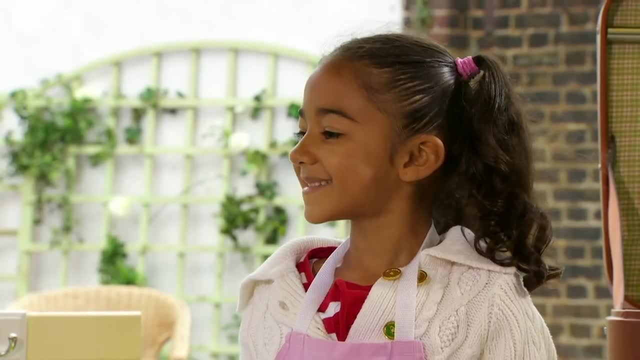 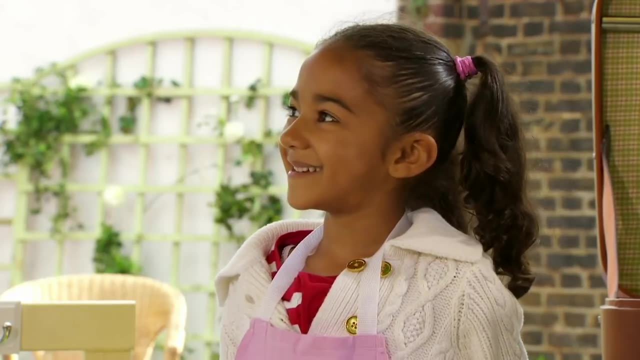 And to do snipping. what are we going to use girls Scissors, But remember, be safe with scissors. Everybody knows that we point them down towards our Home. You've got it. Let's get snipping girls. 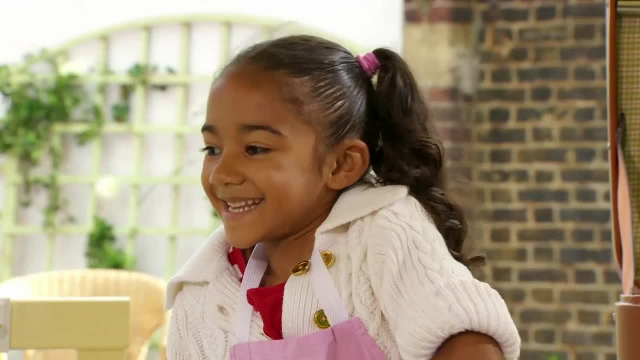 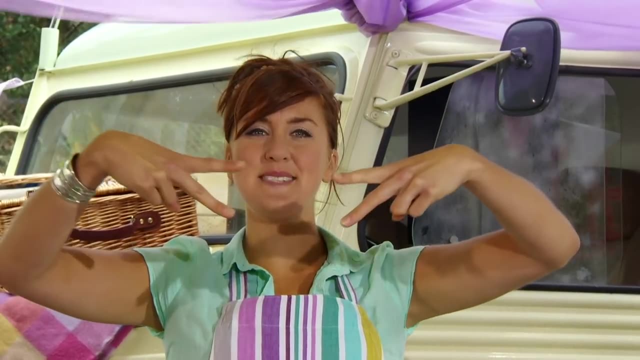 It smells minty. Yeah, It smells minty. And you can do some snipping with us at home too. Get your scissors like this and go snip, snip, snip, Keep snipping everyone. Snip, snip, snip. 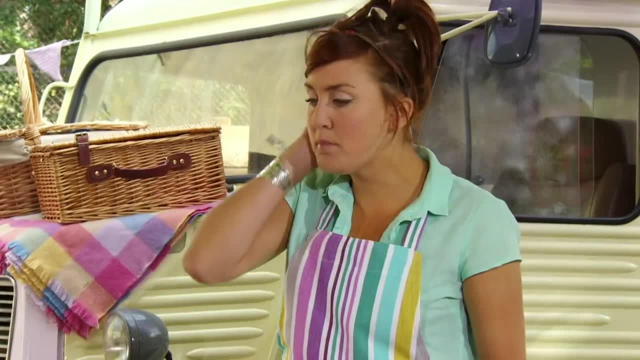 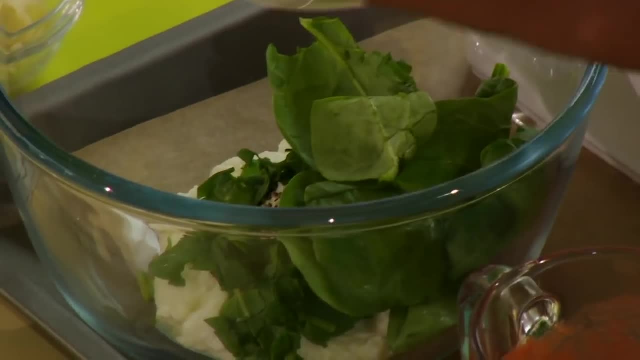 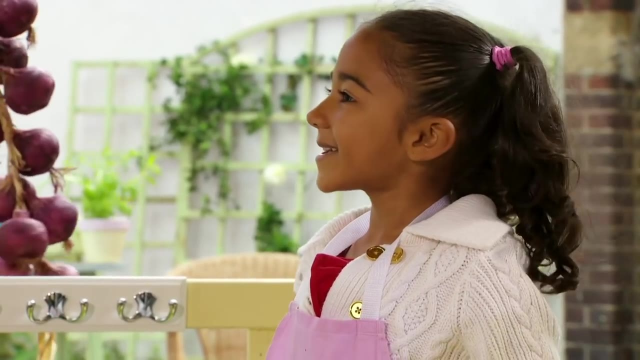 Snip, snip, snip And once you've finished snipping, you can put the mint leaves and the spinach leaves into your bowl of cheese. Mint leaves and cheese. When the scissors touch the bowl, it sounds like music. Oh, it does, doesn't it? 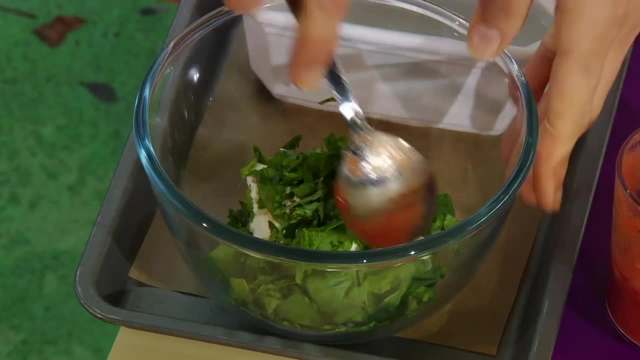 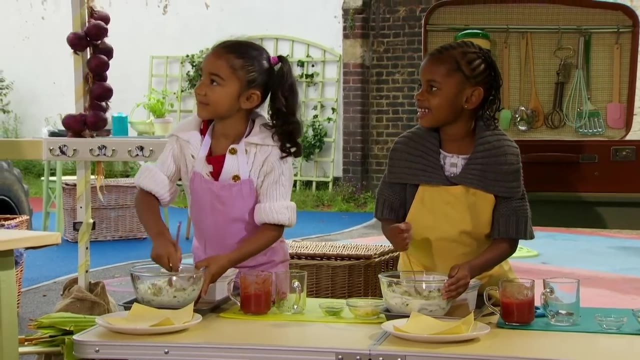 And then we're just going to give everything in that bowl a good mix with our spoon. Whiz it around everyone, Remember to mix with us at home. Get your bowl, You've got it. Get your spoon, You've got it. 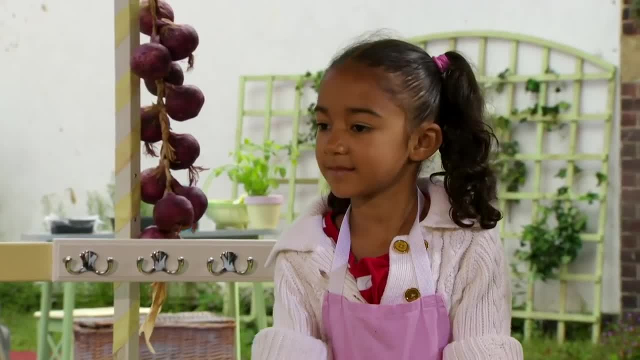 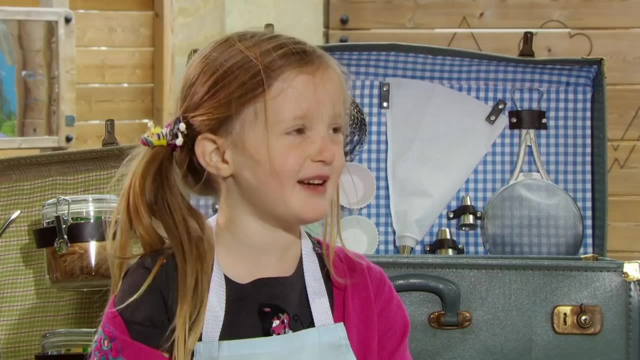 And mix, mix, mix, And next we're going to use this. It's a pasta sheet. Have you ever had pasta like this before? Yeah, I have. I use that for lasagna. It's really tasty, isn't it? 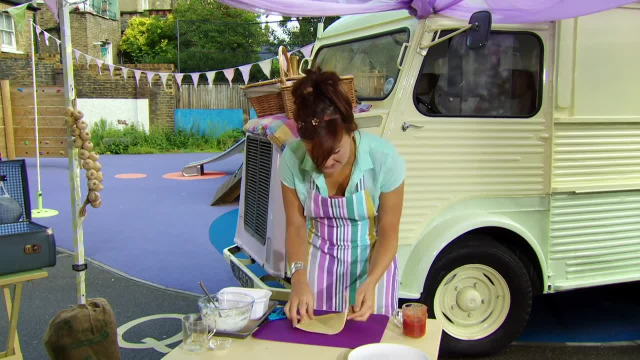 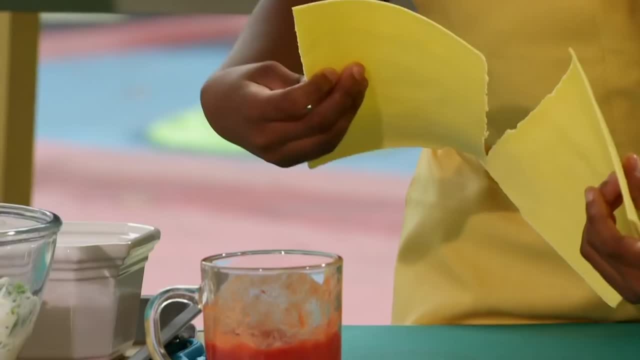 Right now we're going to take this pasta. We have to fold it in half, like this, Can you see, And then you can break it into two pieces. It looks like two little wings. That's it. So we're going to. 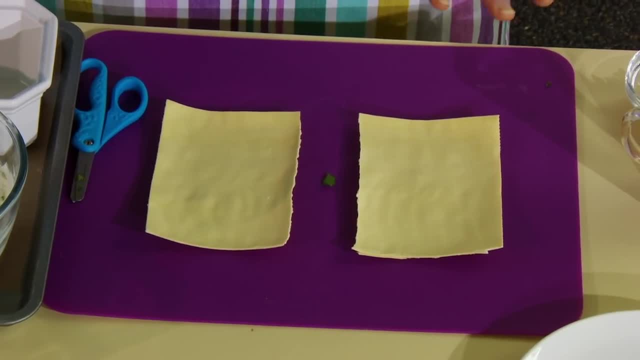 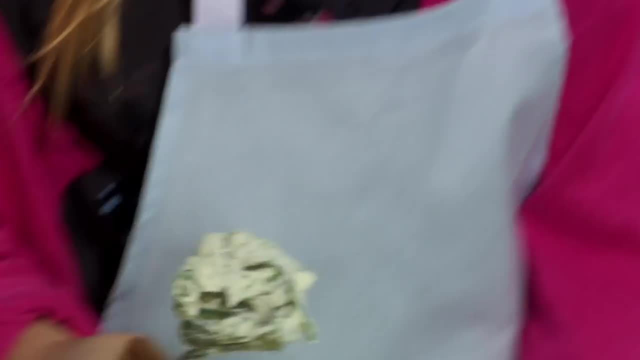 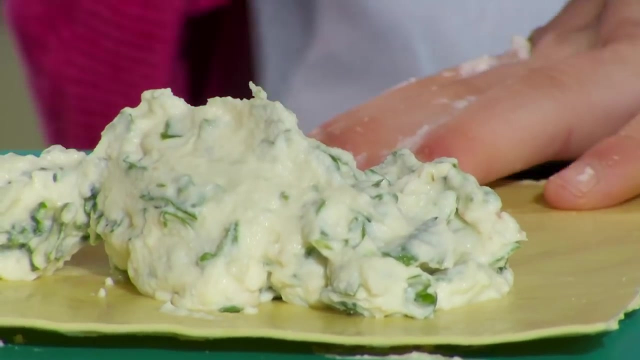 We're going to spread our cheesy mixture all over these pasta sheets And we're going to take a really big spoonful of our cheesy mixture and put that spoonful on top of one of the pasta sheets And then get another big spoonful and put that on top of the other pasta sheet. 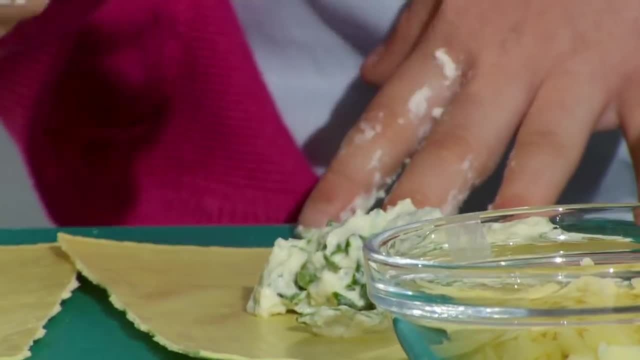 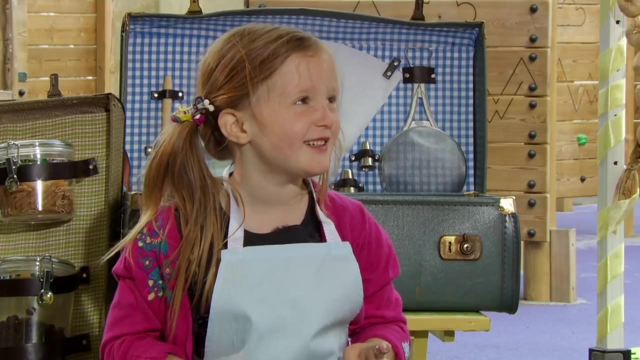 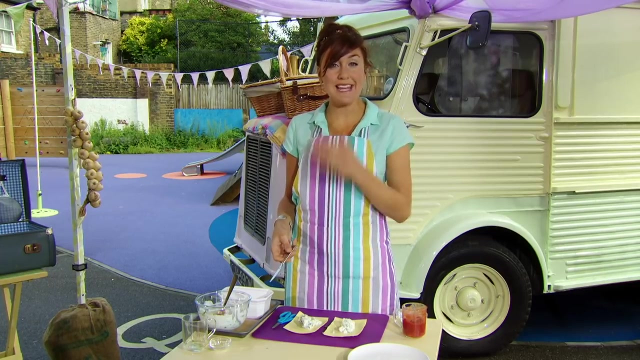 And you need the same amount on each sheet. I can see little green bits, So who's ready to do some spreading Me? Me, We're going to spread our mixture over the pasta sheets using a knife. Now, some knives can be quite sharp, so you do have to be really careful. 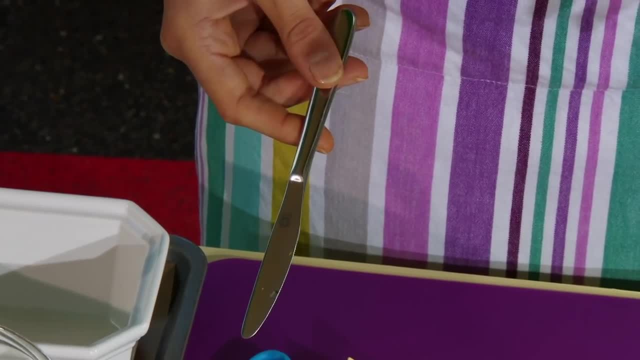 But this is just a table knife, which is the kind of knife that you might be used to using when you're at home, And it's absolutely fine for us to use. So, girls, are you ready to do some spreading, Yeah? 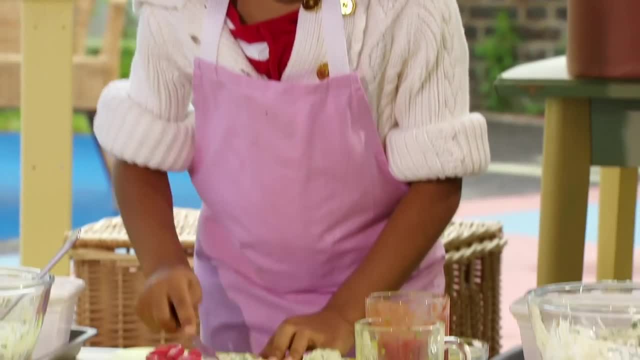 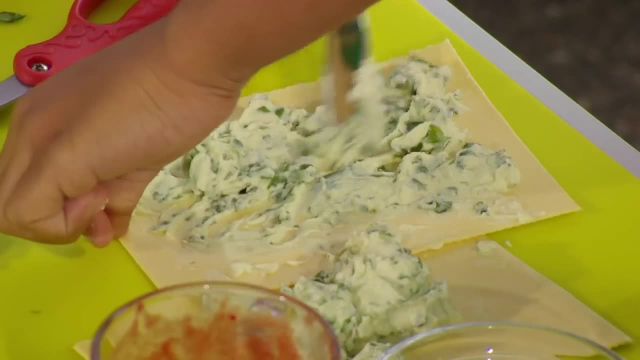 Come on, then let's get going. It's a bit like spreading butter on toast. Have you done that before? I have. Oh, it's like painting a pretty picture. It looks like It's like people making a snow picture, with leaves all fall down and snow. 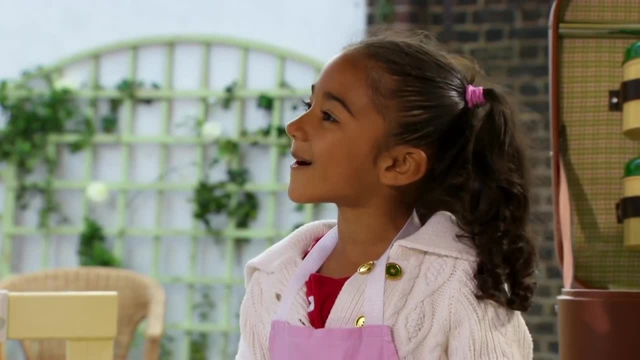 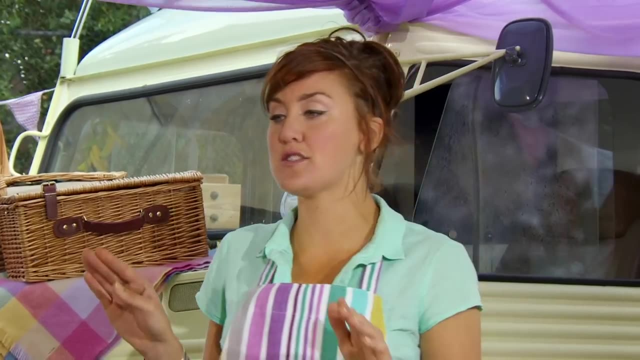 It looks like a house, but it hasn't got a chimney, so it looks like a tower, A very pretty house with lots of patterns around the front of it. And then, once you've finished spreading everyone, we are going to do some rolling. 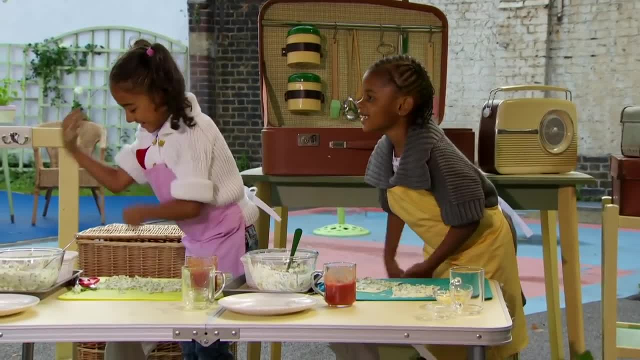 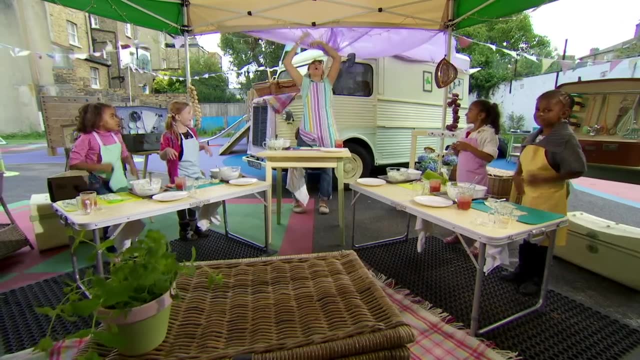 So let's roll up, roll down and then roll it all around. Whoop, Why don't you join in with the rolling dance? Roll up, roll down and roll it all around. Who's ready to roll their pasta Me? 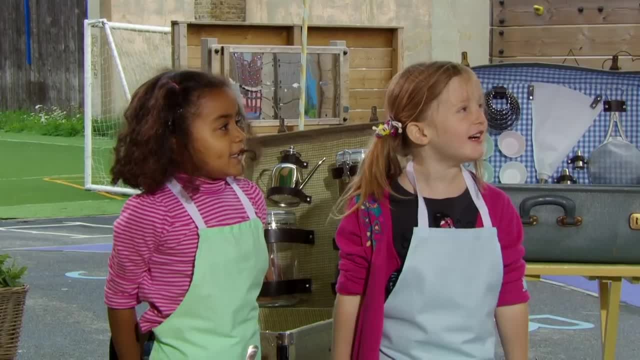 Right, I'll show you how to do it, girls, But we do actually have to be quite careful doing this. So get your fingers on the top bit and roll it up so that it looks like a mini rolling pin. Look at this. 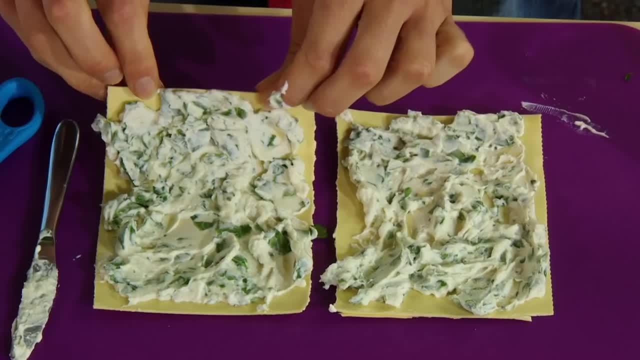 Can you see, And the pasta might break a little bit, but that's absolutely fine. Don't worry about that at all. It's a bit fiddly, isn't it, Jada? It's got bigger and bigger. That's perfect. 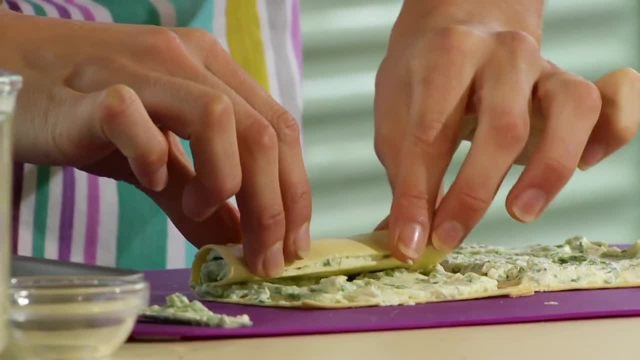 That looks absolutely great. Don't worry if it's squeezy, We're going to roll it all around. Who's ready to roll their pasta? Me Right, I'll show you how to do it, girls. But we do actually have to be quite careful doing this. 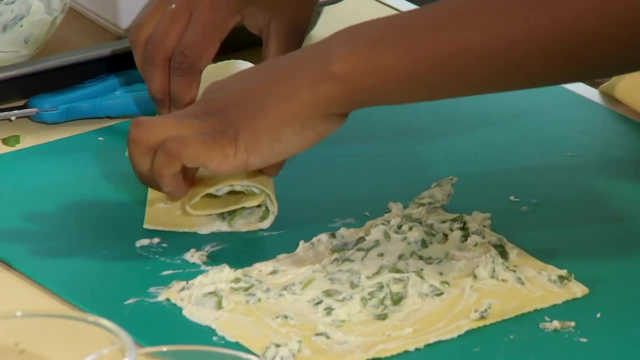 Don't worry about that at all. It's a bit fiddly, isn't it, Jada? It's got bigger and bigger. That's perfect. That looks absolutely great. Don't worry if it squeezes out the end either. 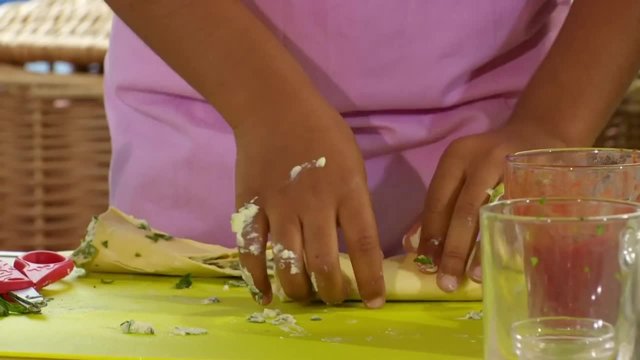 Actually, that's probably going to make it taste even better, to be honest. OK, The next thing we're going to do is take our spoon and scoop up some of our tomato mixture and put it into your dish. You don't want to use all of it, though. 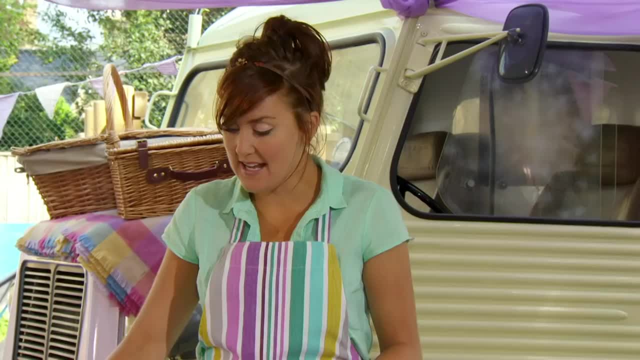 Only half of it And then spread it around at the bottom of the dish. OK, And now we're going to take our spoon and scoop up some of our tomato mixture and put it into your dish. You don't want to use all of it, though. 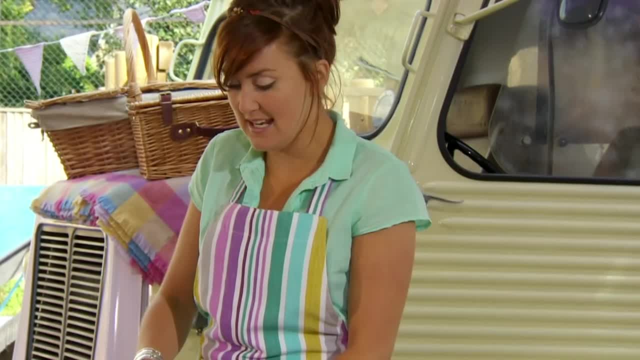 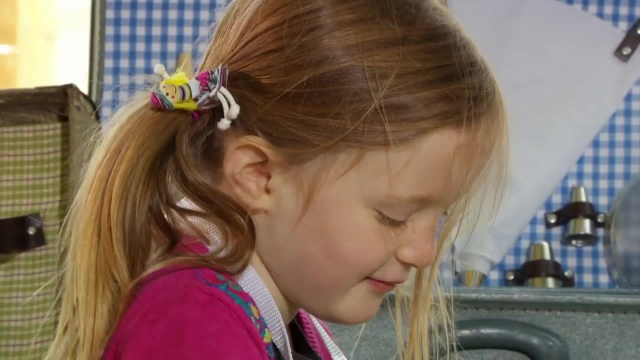 Only half of it, And then spread it around at the bottom of the dish. OK, And now it's time to put our lovely cheesy pasta rolls into their tomato bath. There's one, And then you can scoop up the rest of the tomato and put it on top. 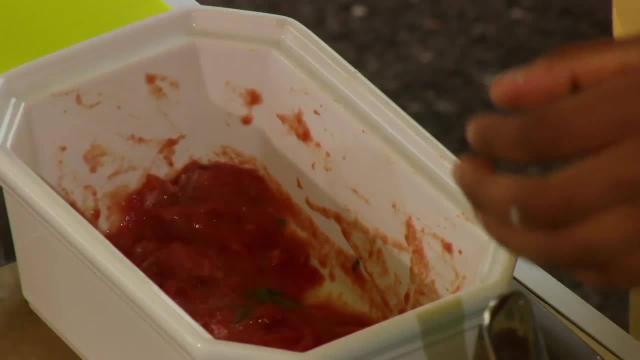 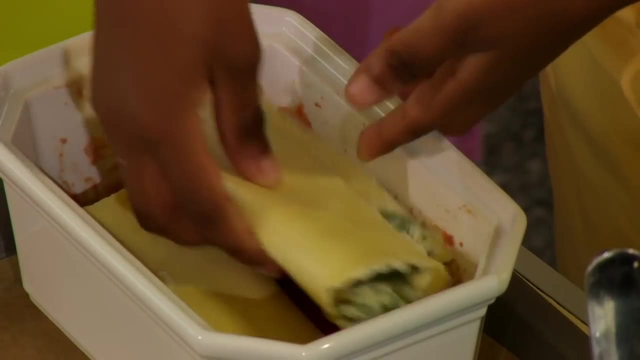 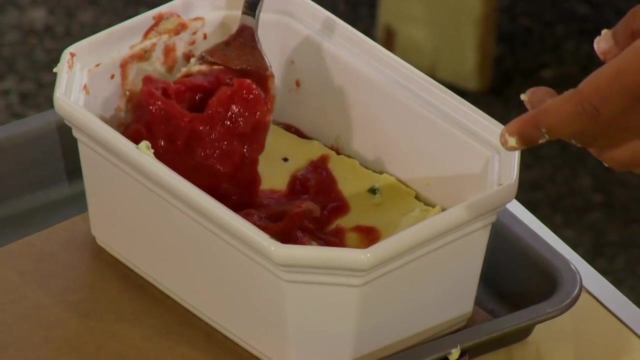 But make sure you cover all of the pasta rolls. So cover them all up like a tomato blanket. And then you're going to take your spoon and scoop up some of our tomato mixture and put it into your dish, OK, And now we're going to take our spoon and scoop up some of our tomato mixture and put 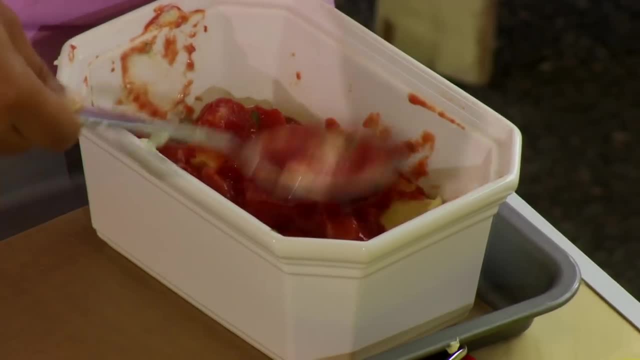 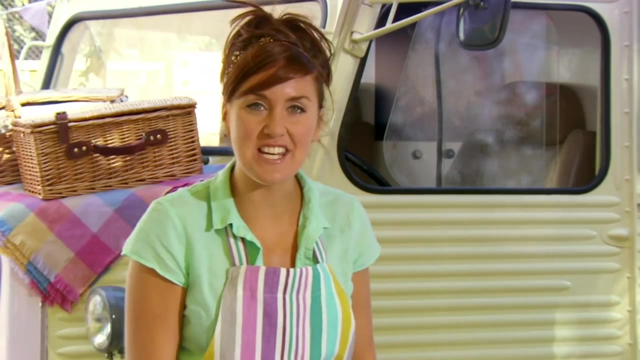 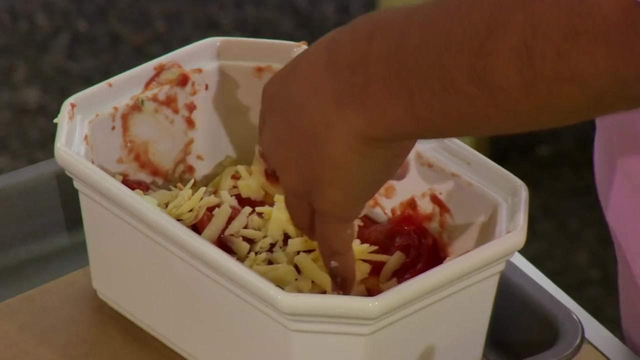 it into our dish, Right? And who's ready for the final part? Me Well, we're going to take some cheddar cheese and sprinkle it on top. Sprinkle, sprinkle, sprinkle, Sprinkle, sprinkle, sprinkle. Finished. Everyone say cheese. 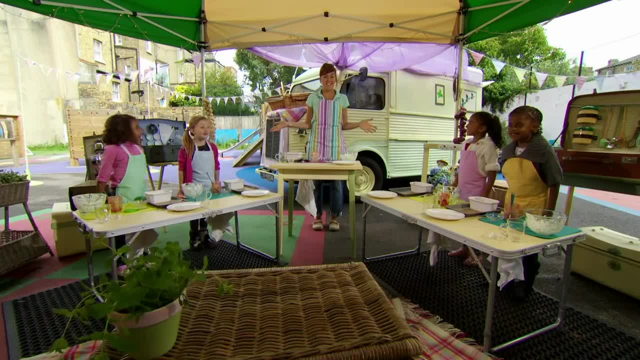 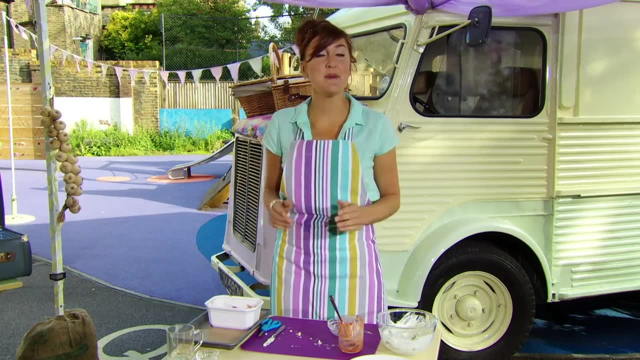 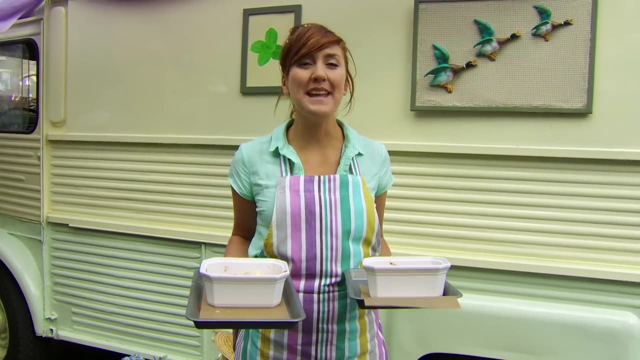 Cheese. Well, that's it, girls. you've done it. You've put all the ingredients together for your cheesy pasta rolls all by yourself, And now it's time to put them in the oven. But remember, ovens are hot, so don't go near. 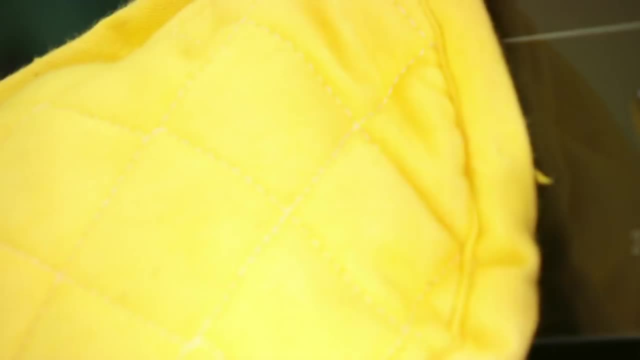 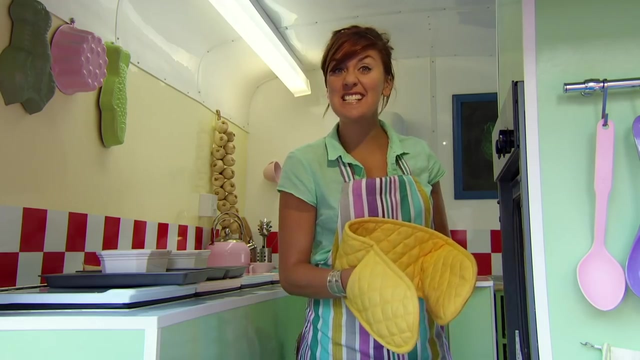 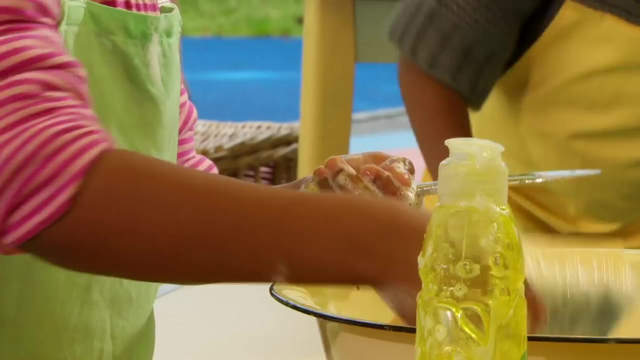 Ask a grown-up to help you here. Now we've cooked with you and had lots of fun. Let's tidy up and think of all the things that we have done. There was Mixing, Pudding, Rolling And Licking. 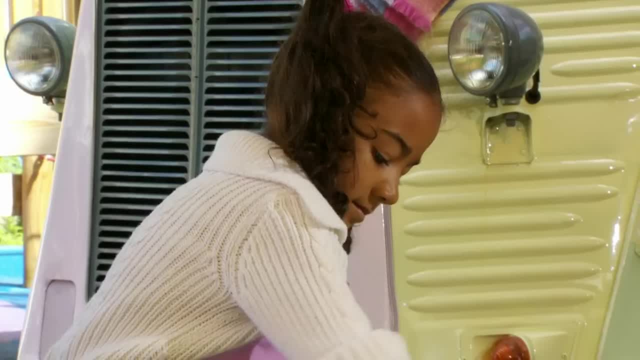 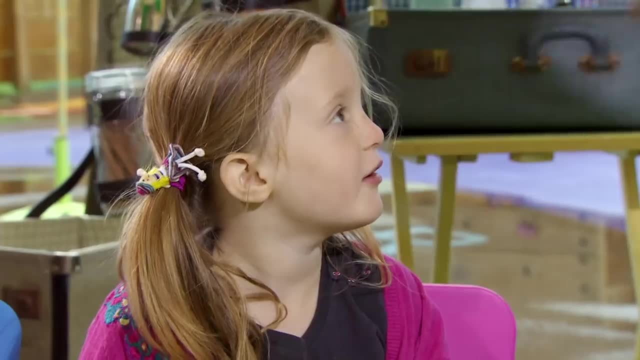 Clearing any mess and putting things away. It's always fun to do. at the end, All done. Have a good day. Look, girls, our food's all cooked in the oven. It smells absolutely amazing. Let's have a look at yours, Freya. 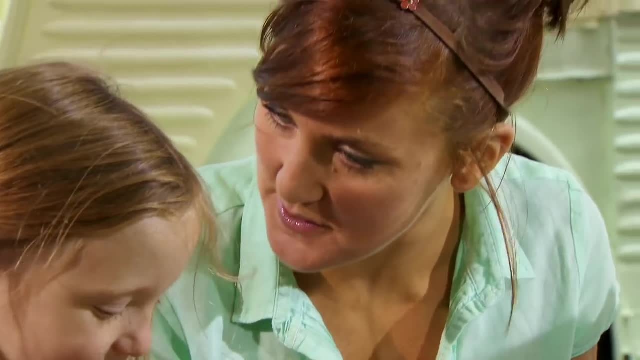 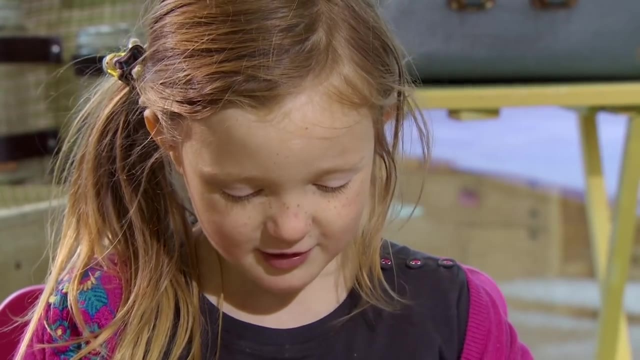 Looks like a sausage roll. Oh yeah, it does a tomato sausage roll, But there's no sausage in it. And what's happened to yours? in the oven, The cheese has melted and the tomatoes have gotten really sloppy. Let's have a look at your one, Jada. 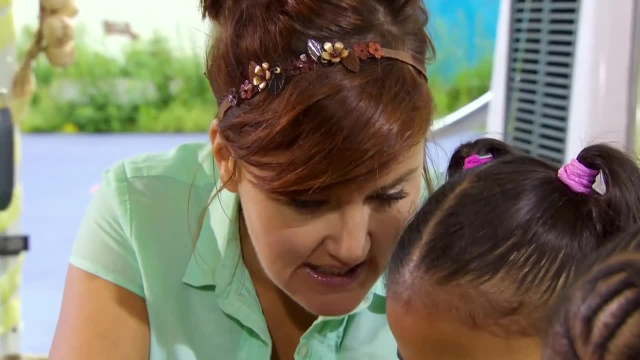 Jada, it looks brilliant. What's this bit sticking up here? The cheesy pasta. Cheesy pasta. Can you point to where the mint is? That's the baby leaf, that's the mummy leaf and that's the daddy leaf. 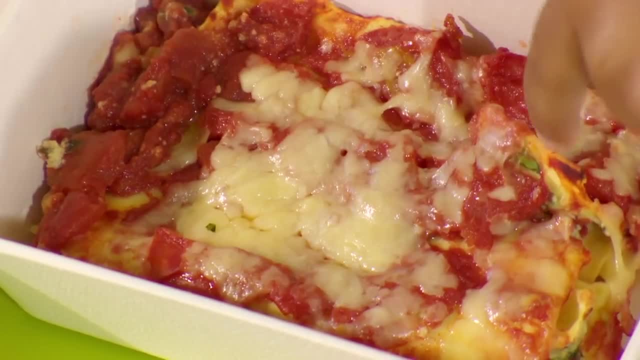 Oh yeah. Oh Jada, are you looking forward to eating it? This is making me extremely hungry, girls. Is it making you hungry too? Yeah, Let's put the lids on top and save our food for this afternoon. We've travelled to you, we've cooked and had fun. 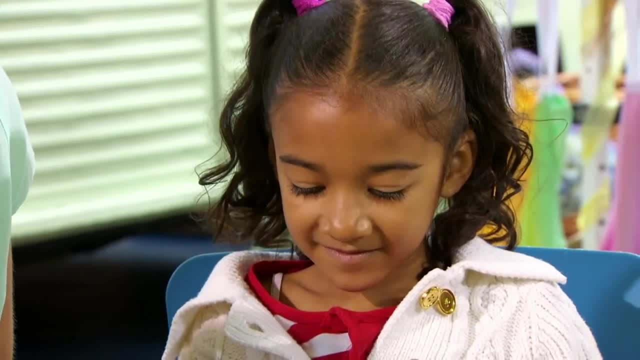 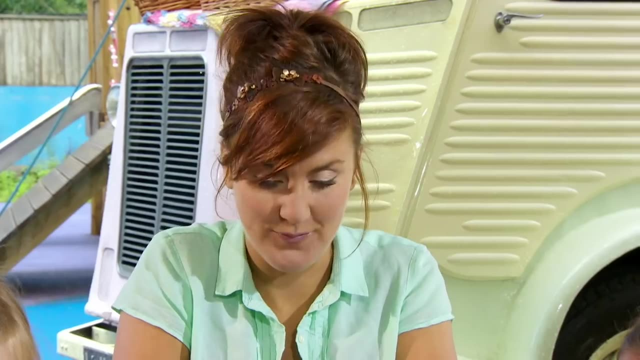 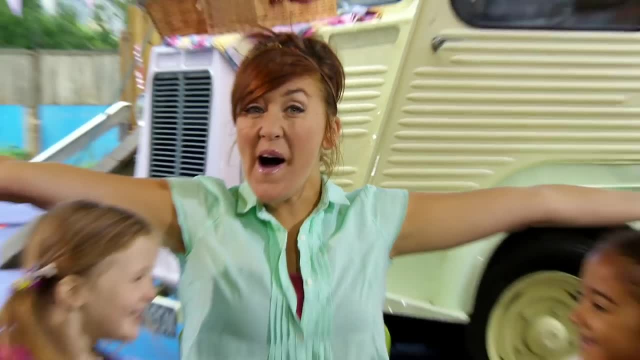 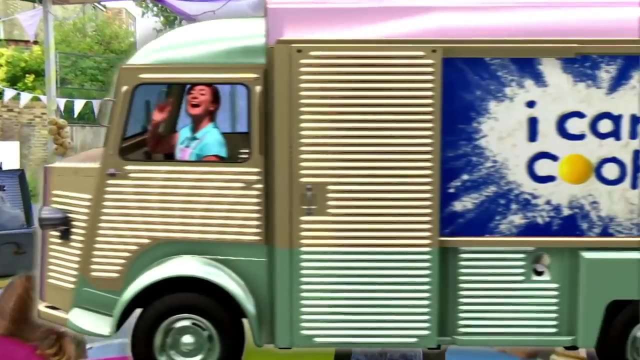 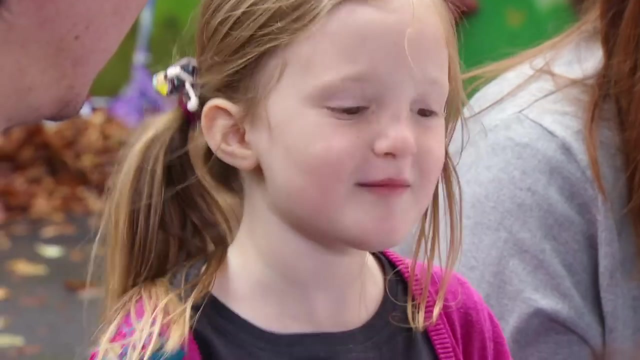 Yay, Yay, Yay, Yay, Yay, Yay. Come on, you can come with us. Let's go, girls. Come on, let's go and share our food. Look at that, Did you make that? 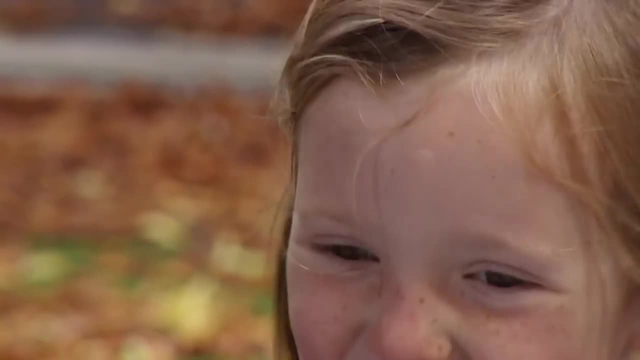 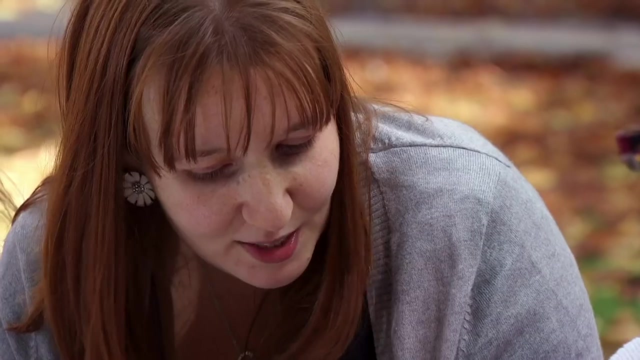 Wow, that's really good. You did a good job. Did you make this yourself? Yeah, It looks nice. How did you get the mint? Katie grew it. Katie grew it. wow, Mmm, that's yummy, Oh, that's delicious. 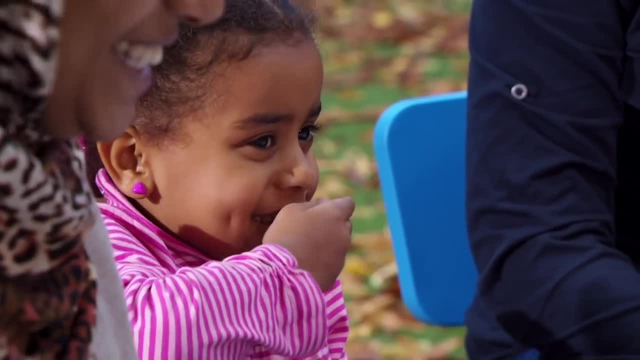 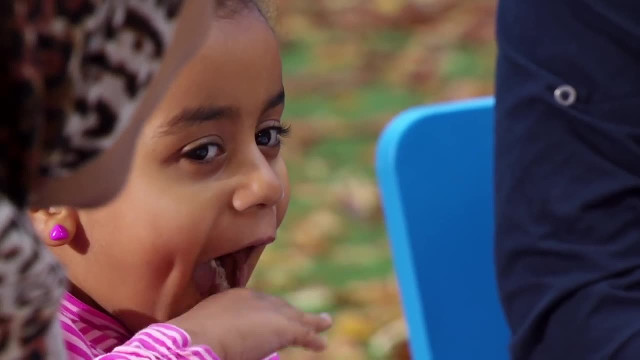 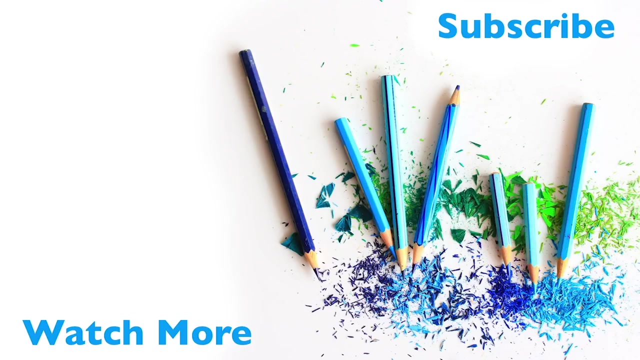 What can you taste? Oh, is it the chilli Hot Shall? I get the fire engine in. Ne-no, ne-no, ne-no, ne-no. So what can you do? I can't fit. Thanks for watching.